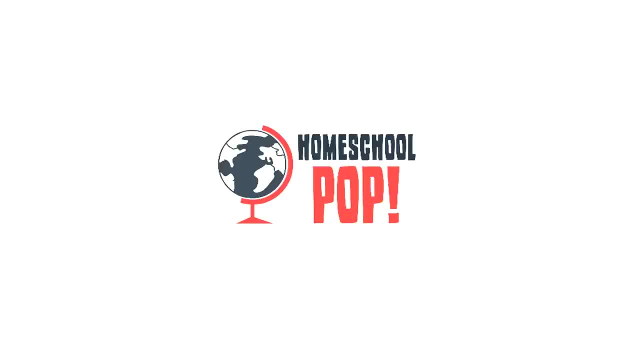 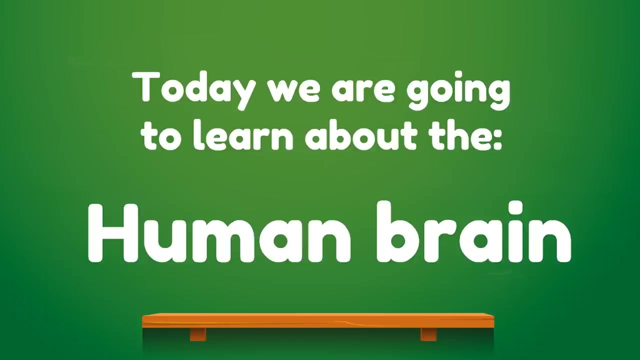 Wow, we are going to learn so many cool things on this homeschool pop video. Alright, what's the first thing we should learn? How about the human brain? Doesn't that sound cool and intriguing and maybe a little bit gross? Well, it's going to be a. 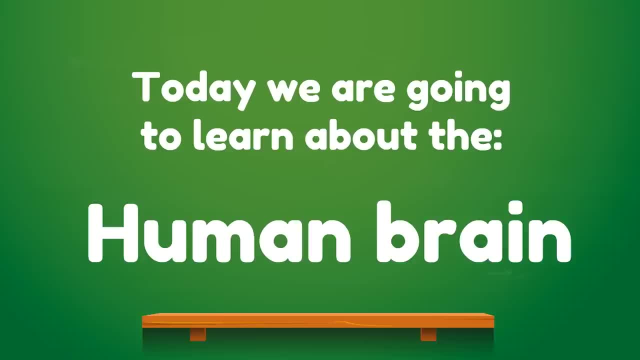 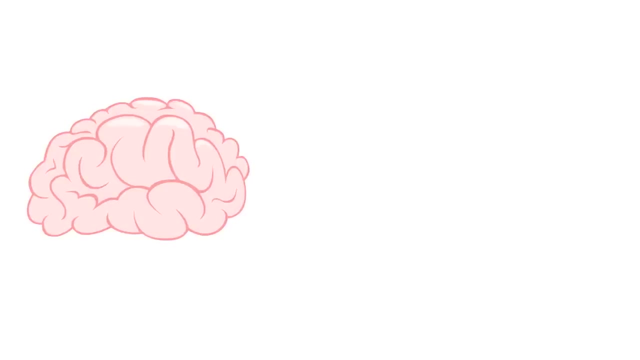 lot of fun because the brain is an amazing, amazing part of your body and you're going to understand it. after watching this video, I know we're going to jump right in. It's going to be so cool. So what is a brain? I mean hearing this drawing, it almost looks. 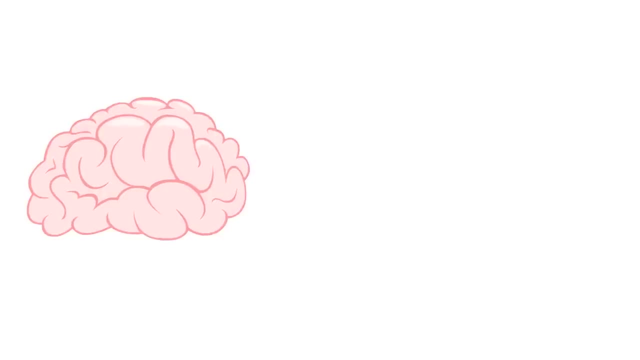 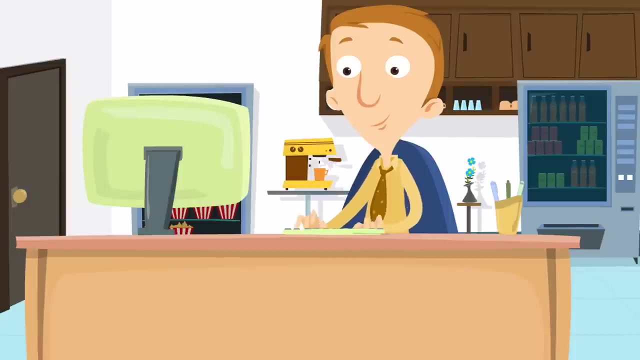 like bubble gum. What is a brain? Well, the brain is an organ of the body. Isn't that interesting? It's an organ of the body, Alright. so what is an organ? Ha, we have to know that to know what a brain is. 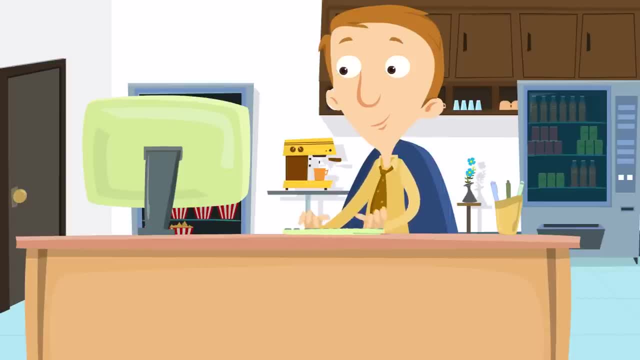 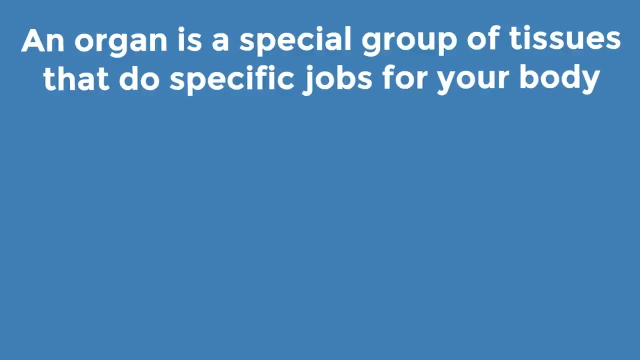 is an organ of the body. what is an organ? it's interesting. an organ is a special group of tissues that do specific jobs for your body, like your heart. your heart is a special group of tissues that does a specific job for your body. an eyeball is an organ, too. it's a special group of tissues that does a specific job for. 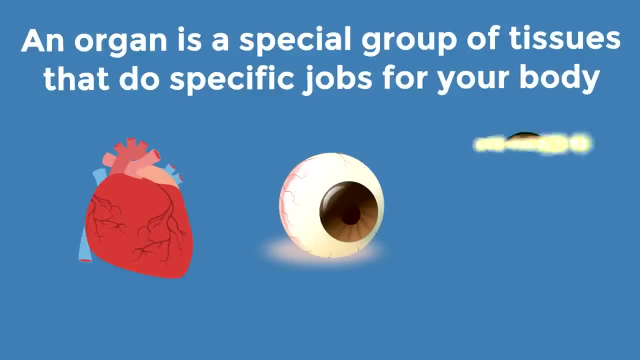 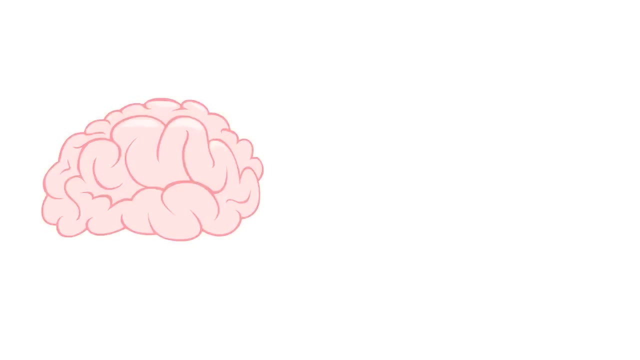 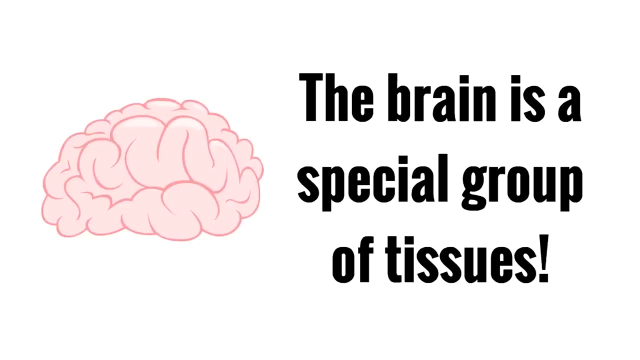 your body. and how about a kidney? a kidney is an organ that's a special group of tissues that does a specific job for your body. see, the brain isn't like just some wad of gums. the brain is a special group of tissues, and not only that. 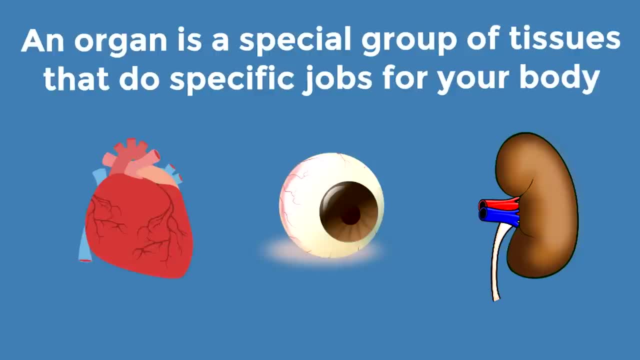 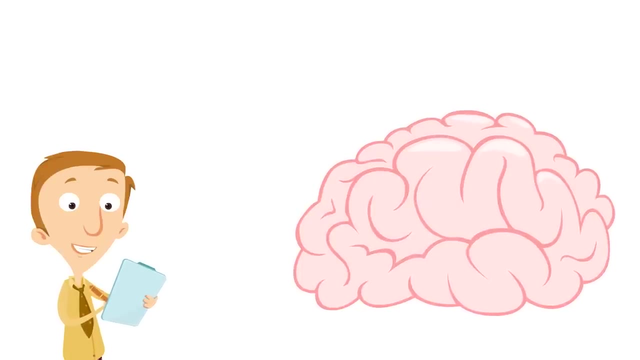 remember, an organ is a special group of tissues that do specific jobs for your body. they do different jobs. they have tasks to do. so we know there are special tasks that the brain has to do, but what does the brain do? what is it that the brain does? well, this might sound crazy. okay, this might. I hope you're sitting. 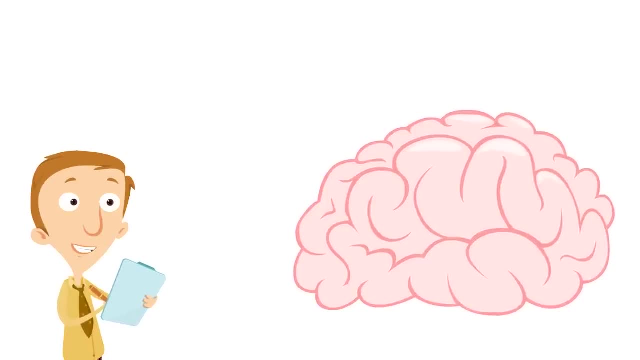 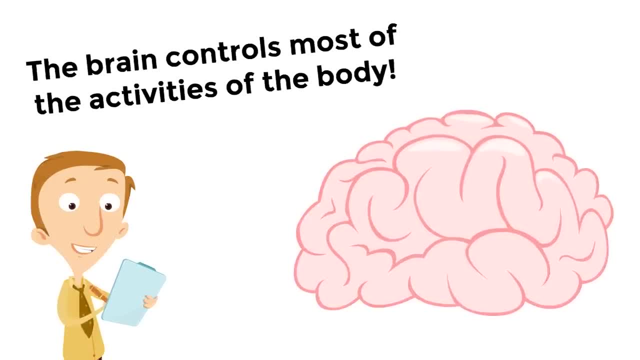 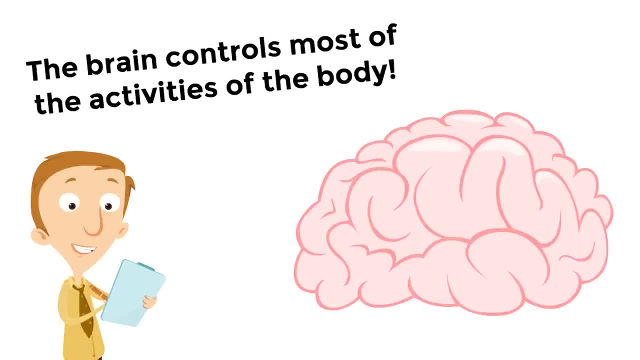 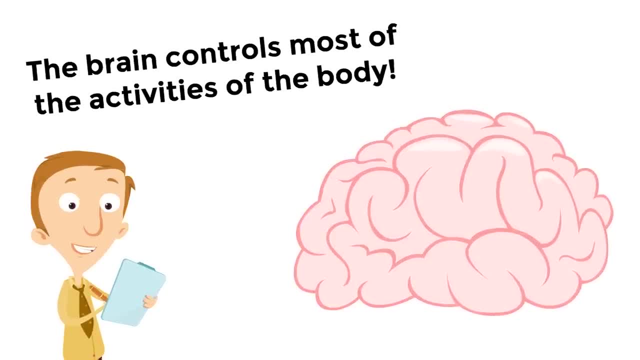 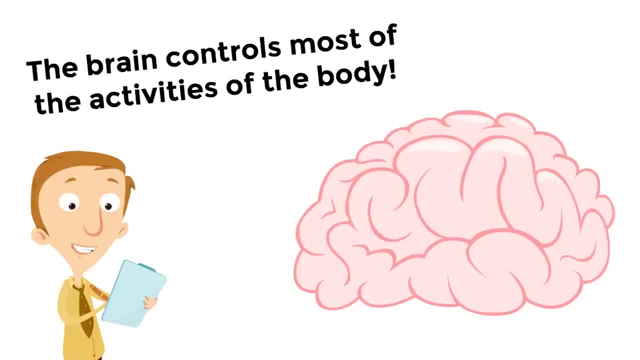 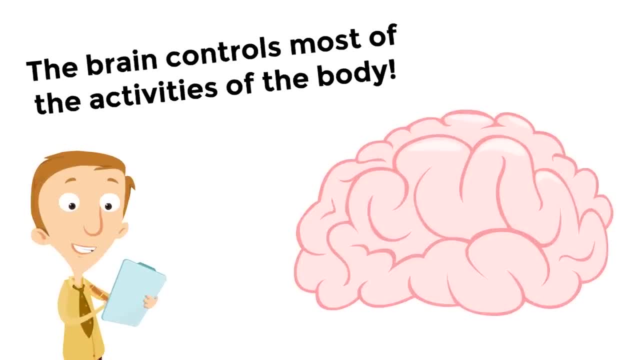 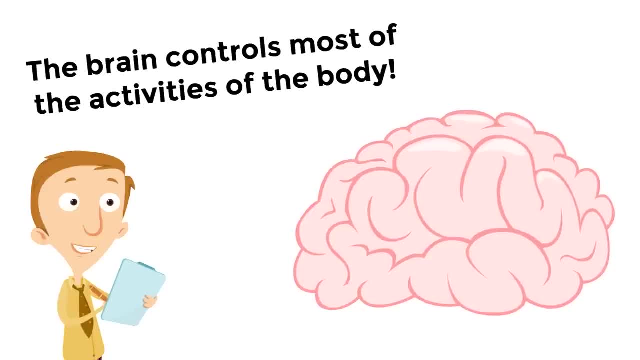 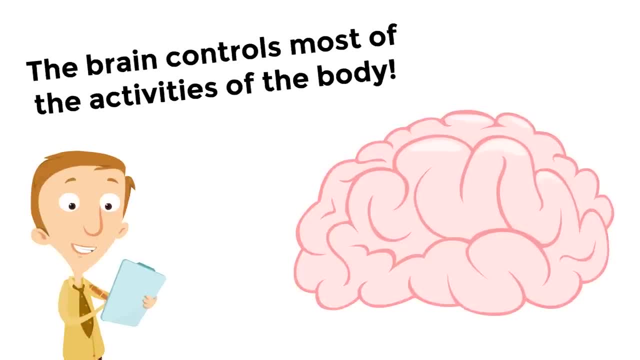 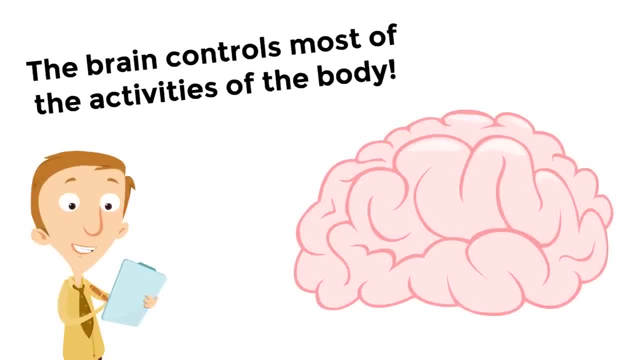 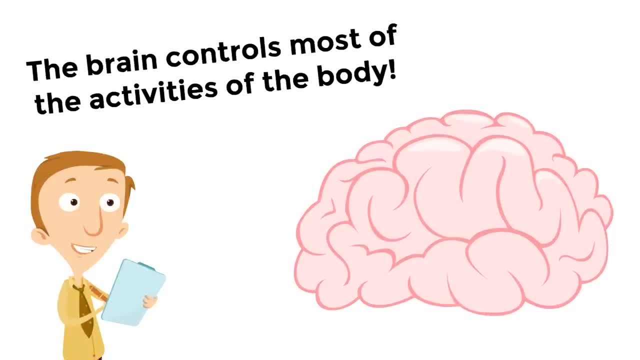 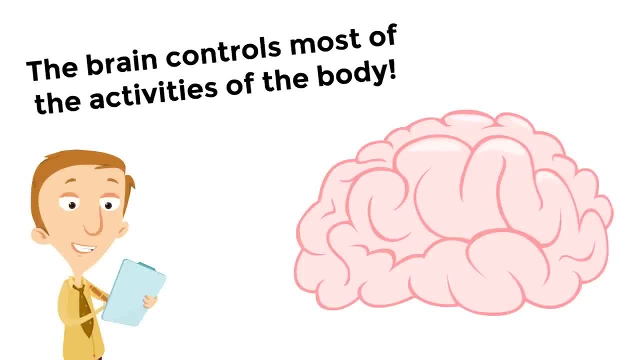 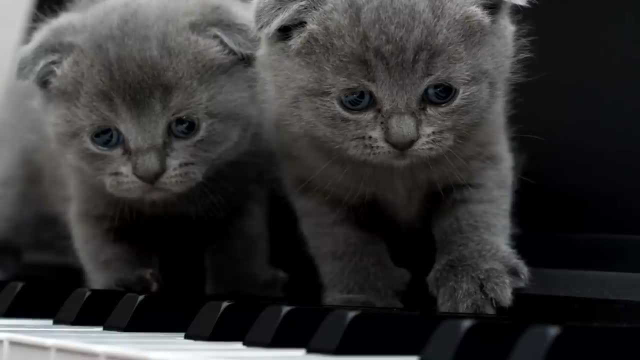 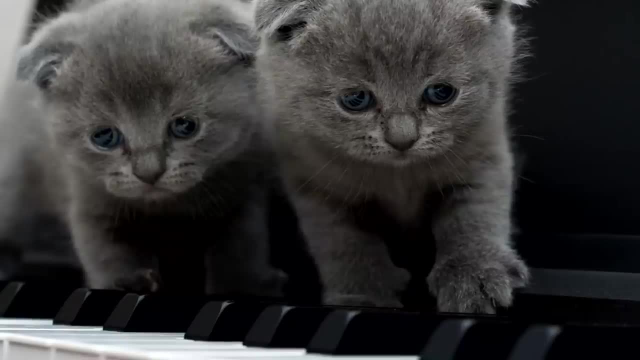 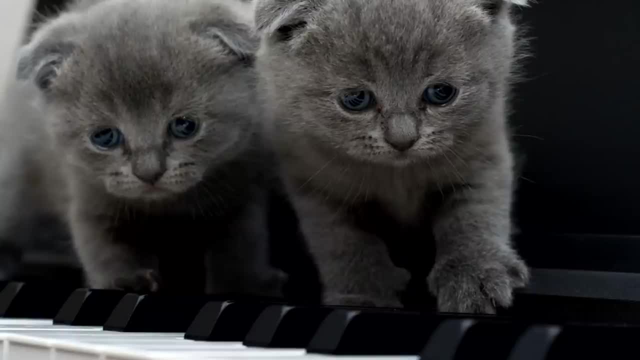 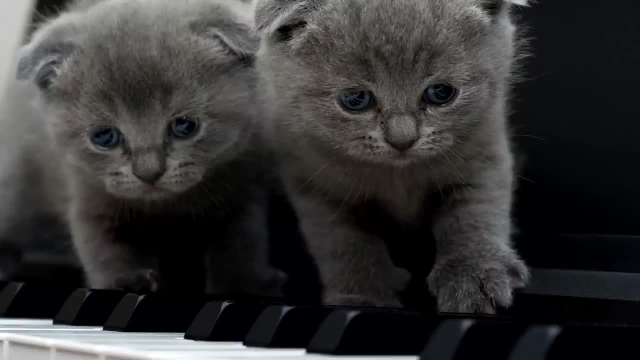 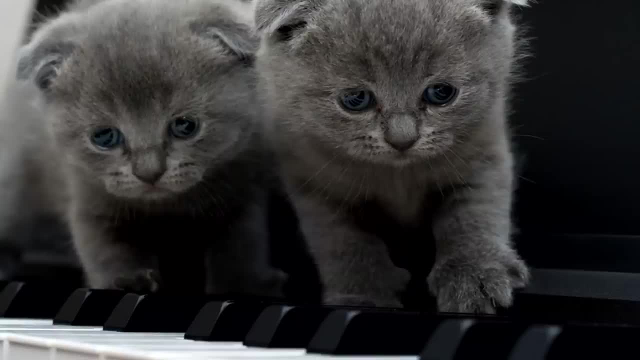 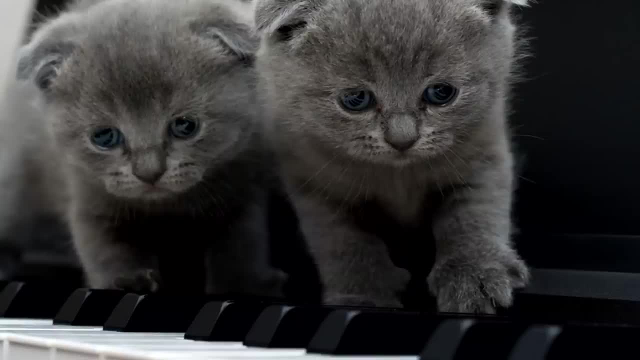 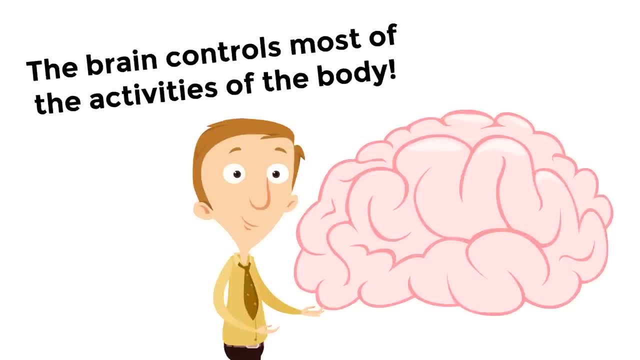 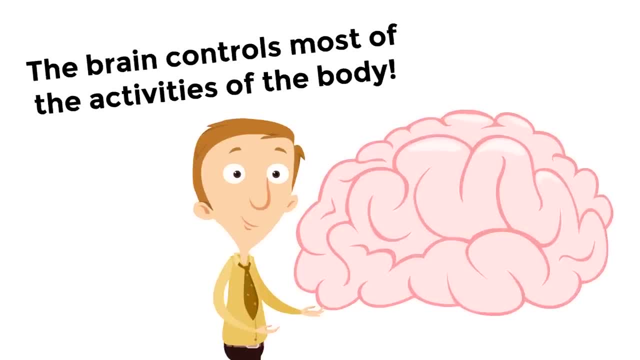 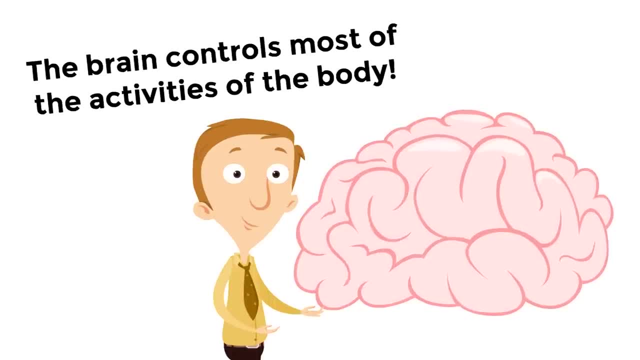 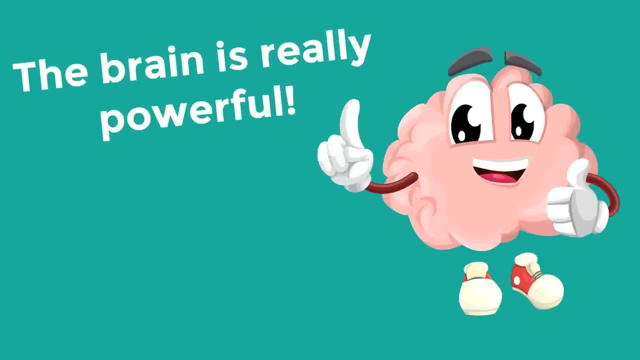 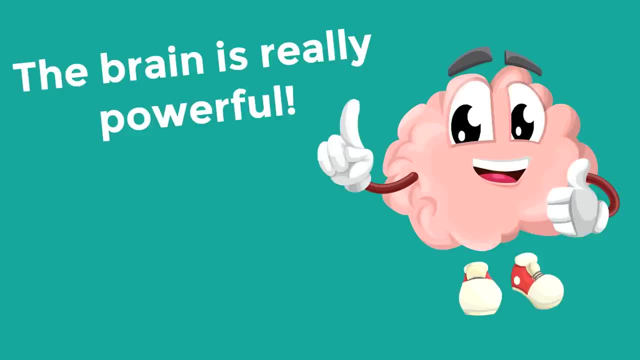 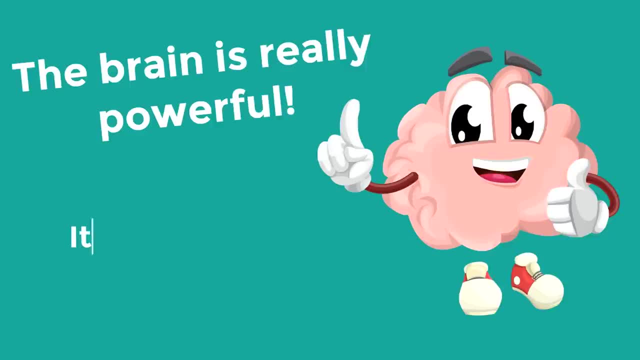 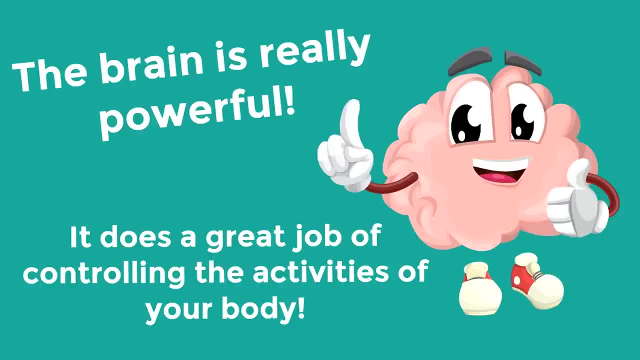 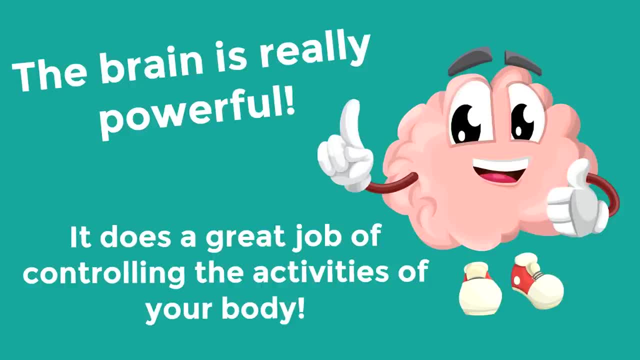 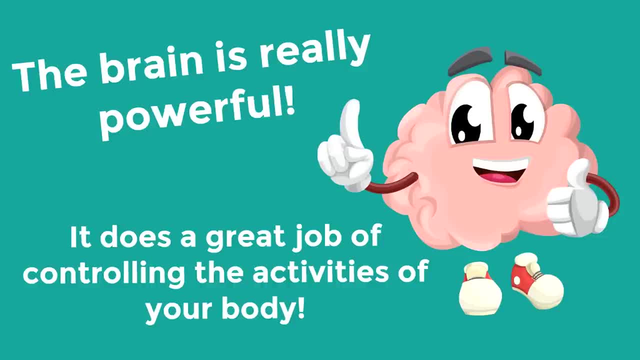 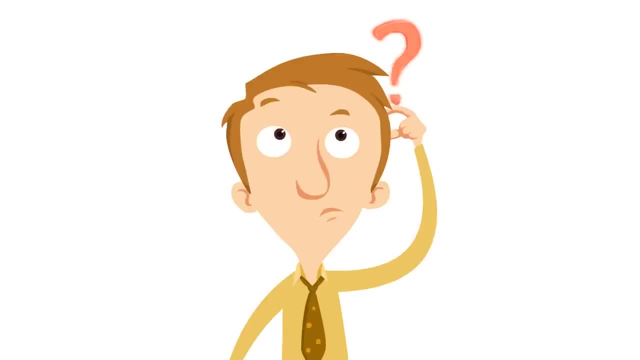 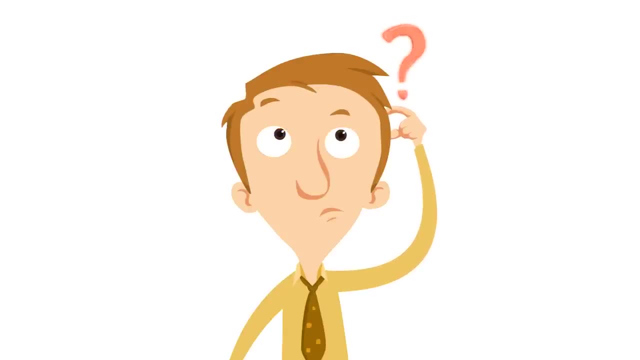 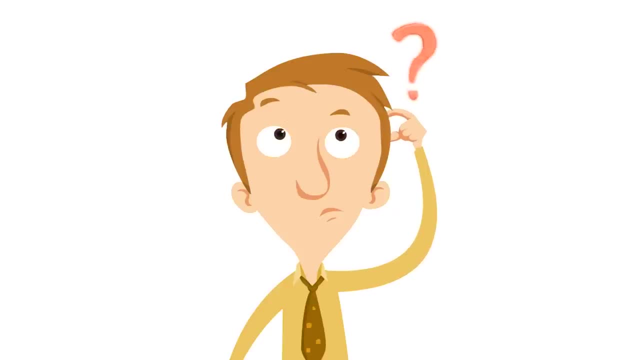 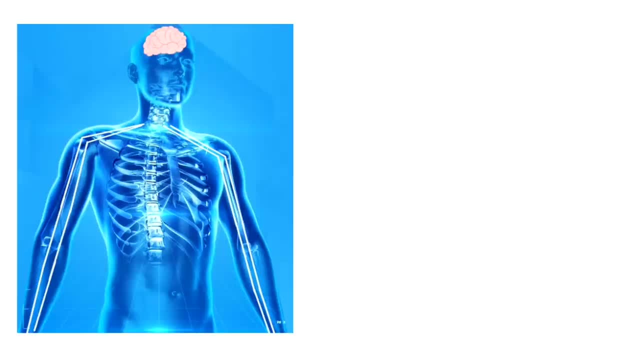 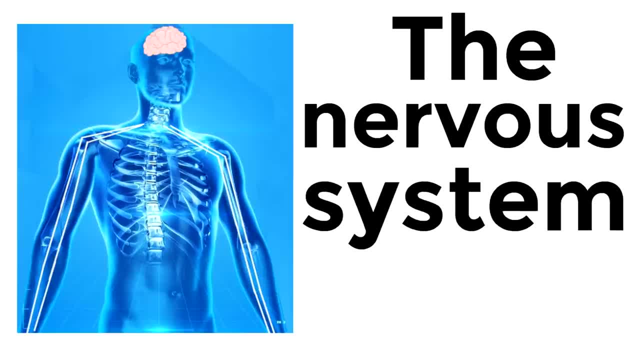 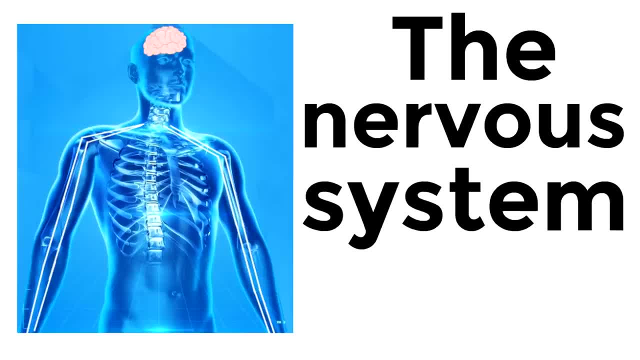 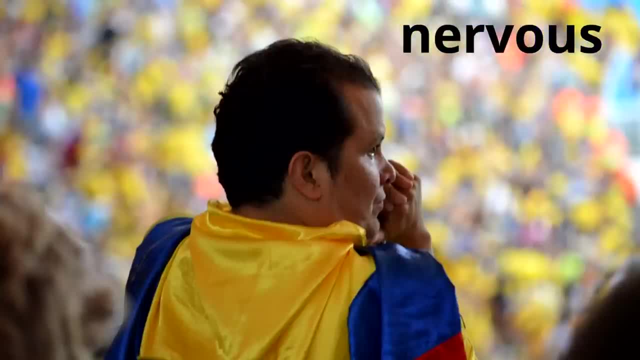 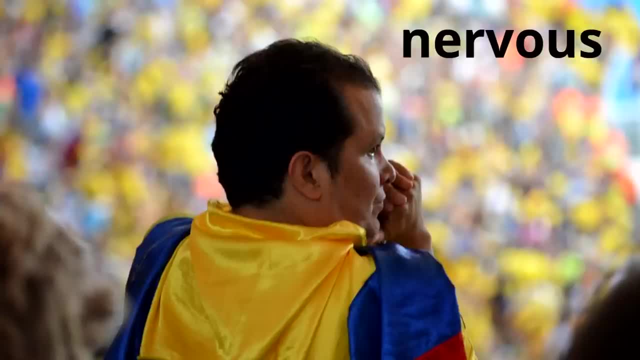 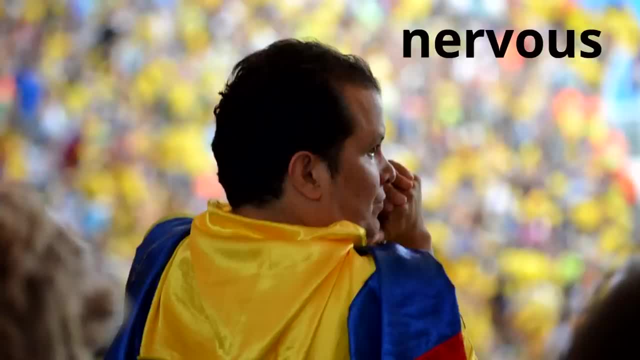 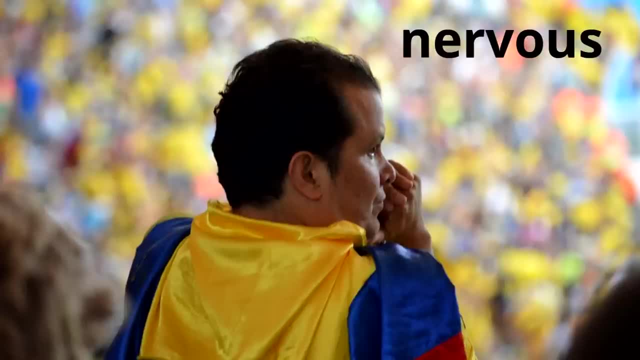 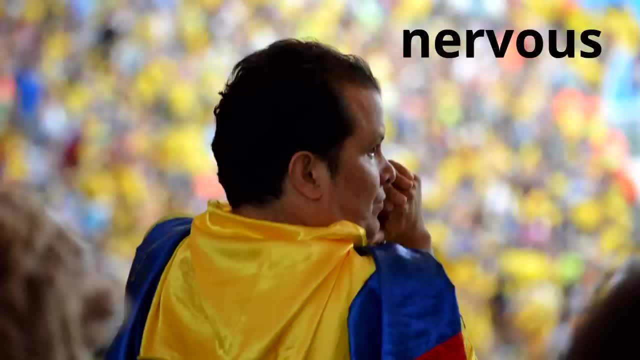 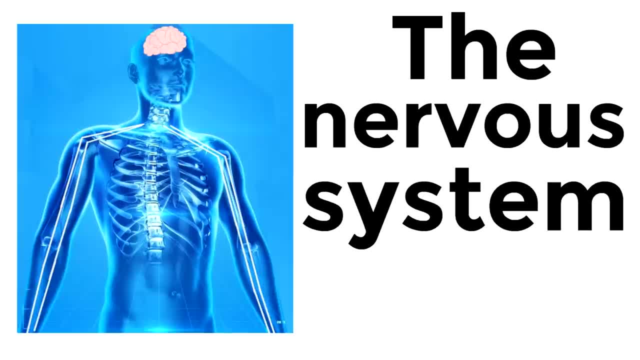 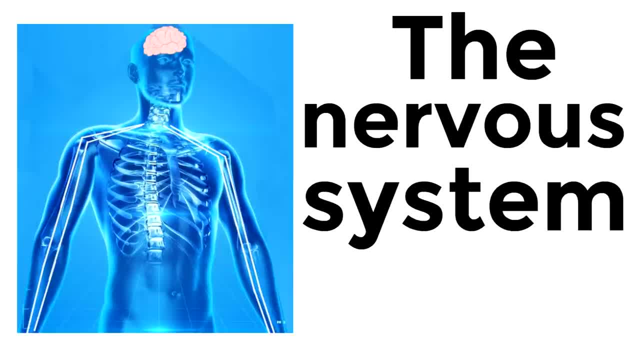 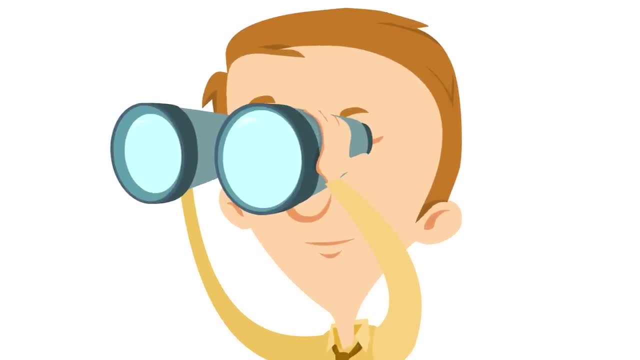 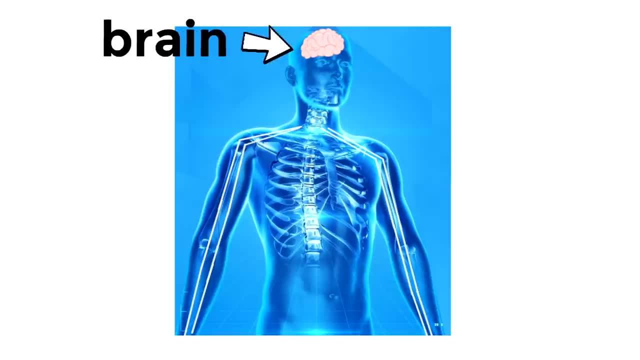 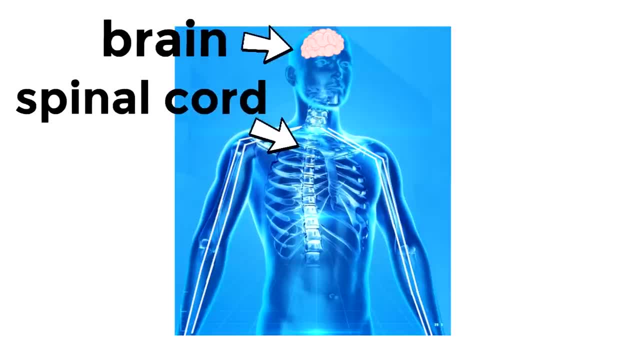 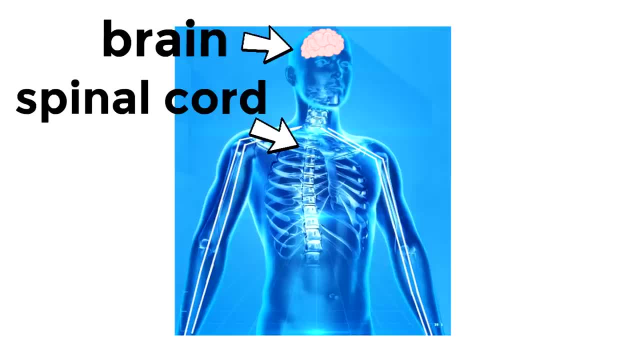 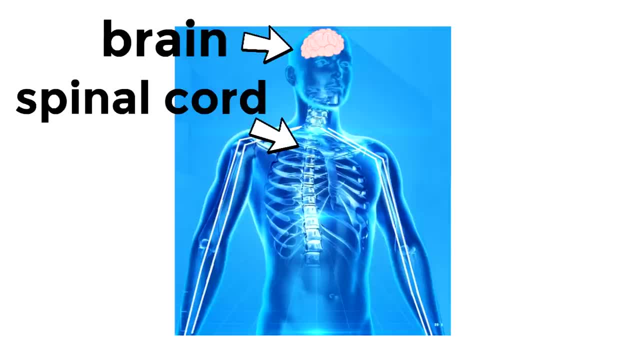 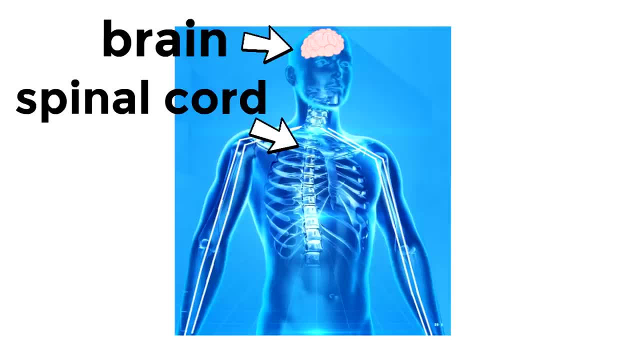 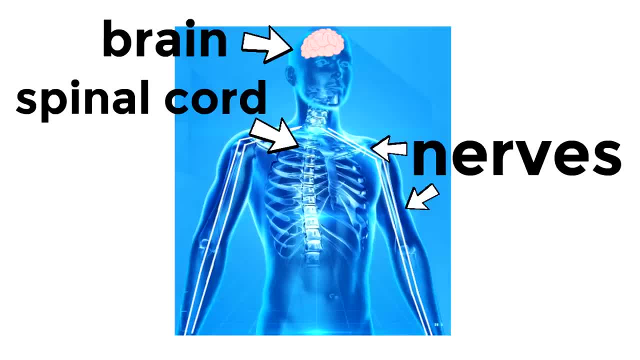 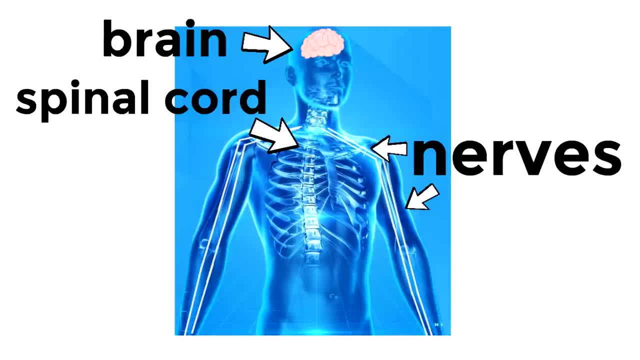 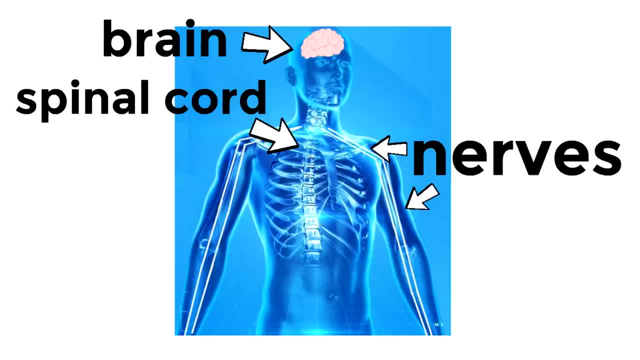 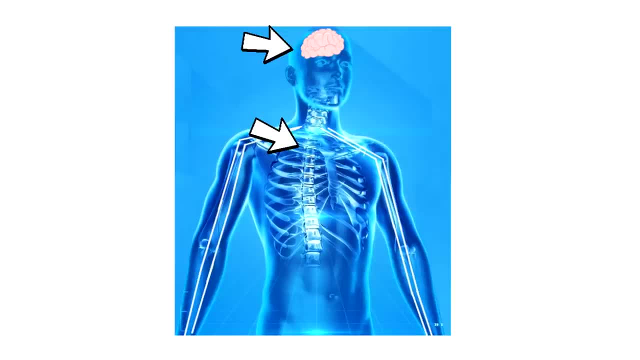 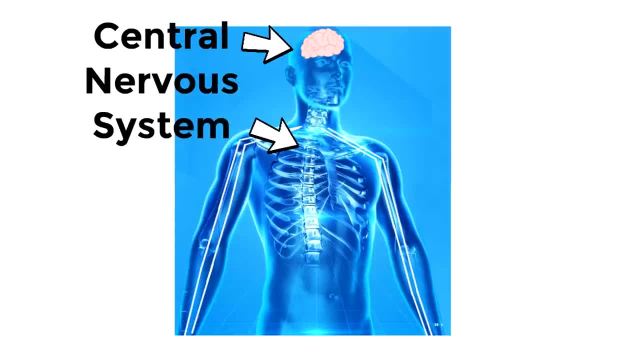 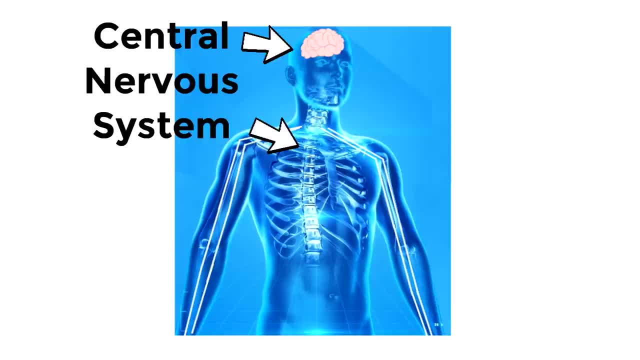 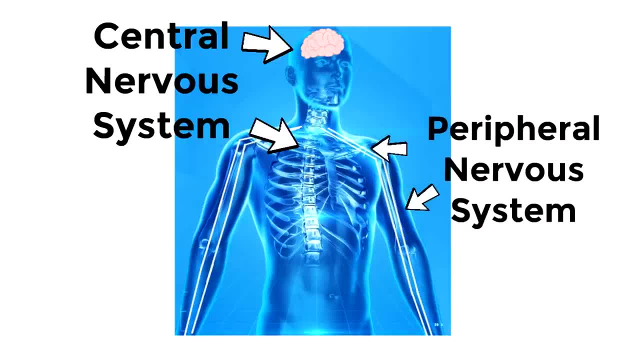 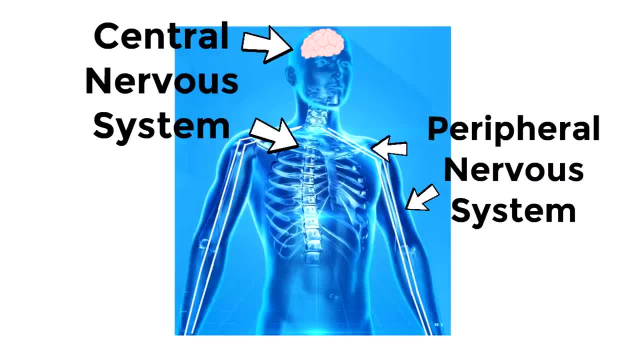 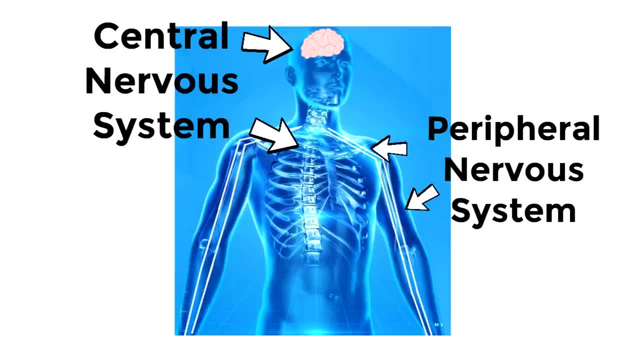 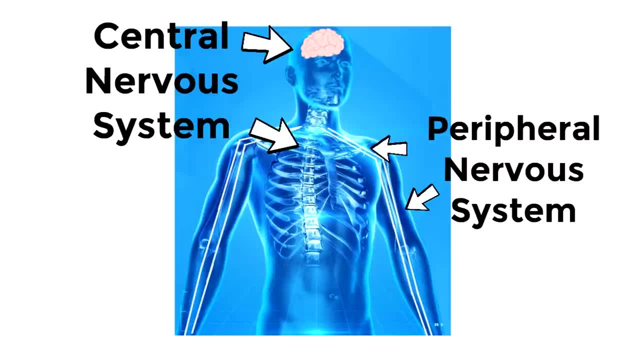 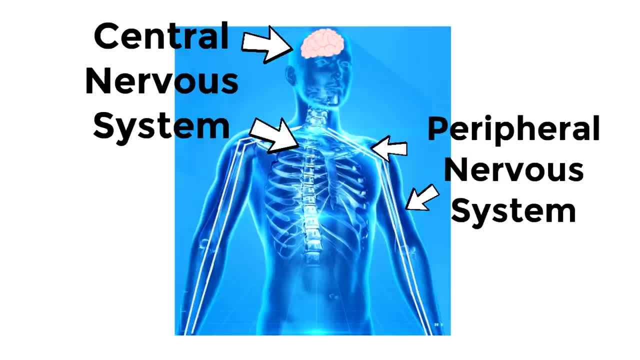 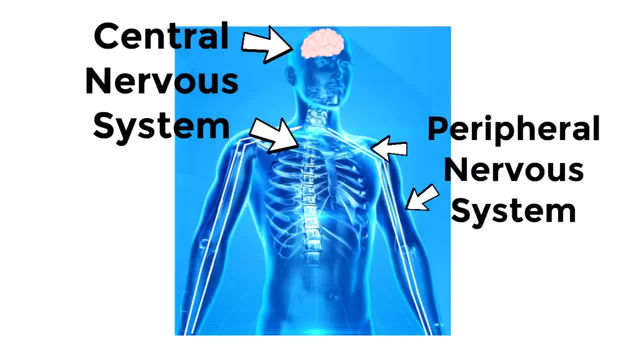 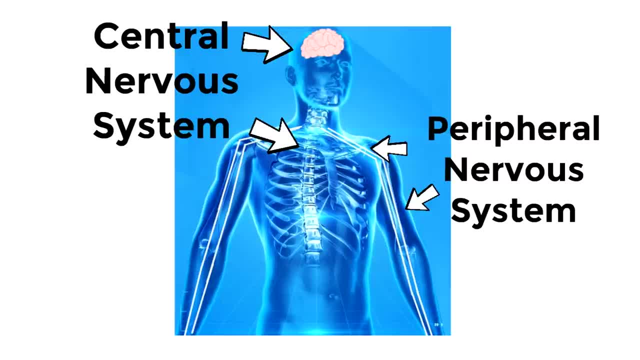 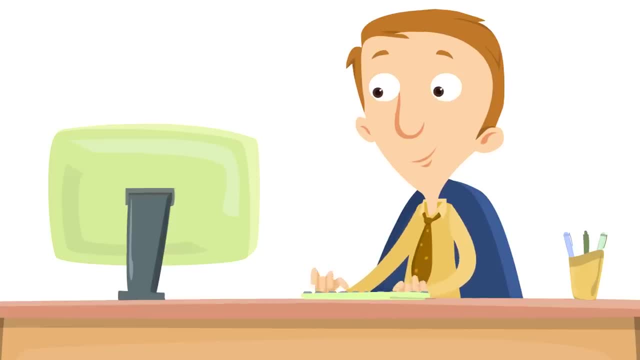 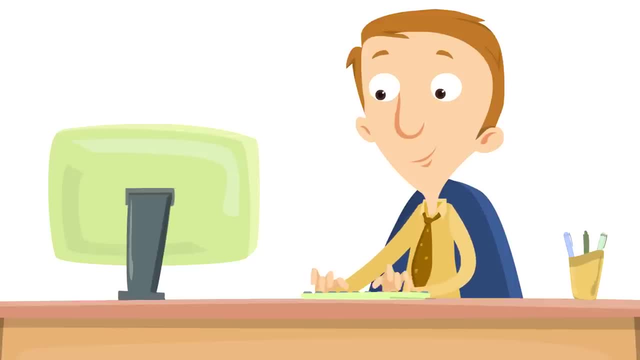 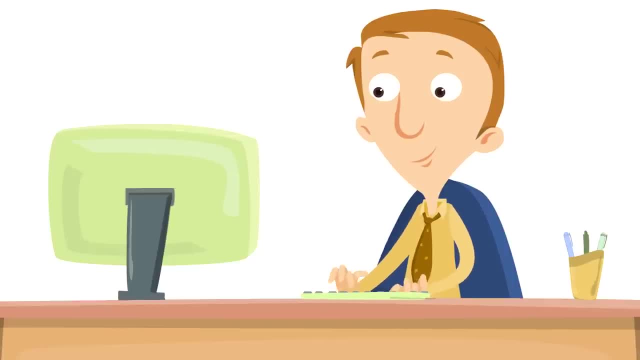 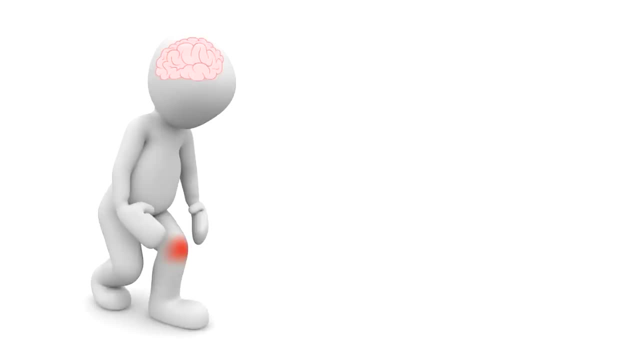 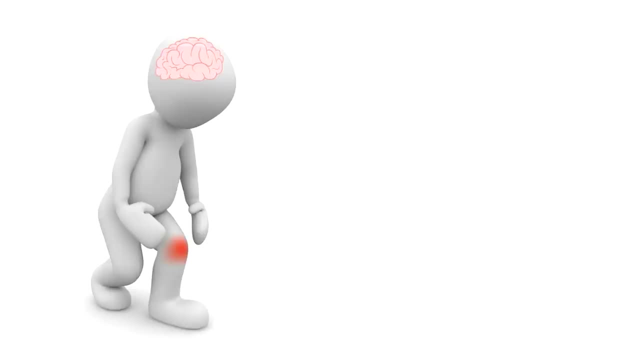 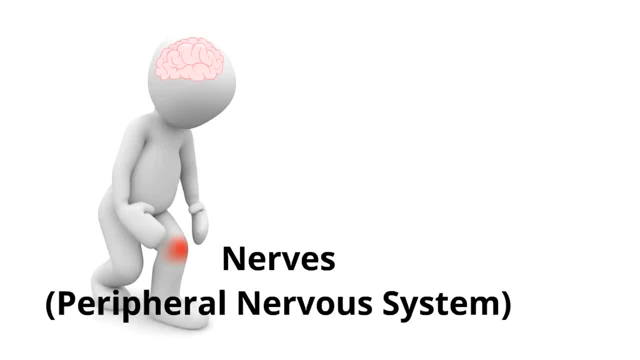 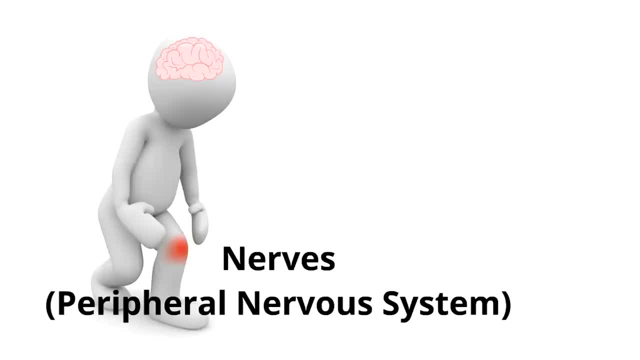 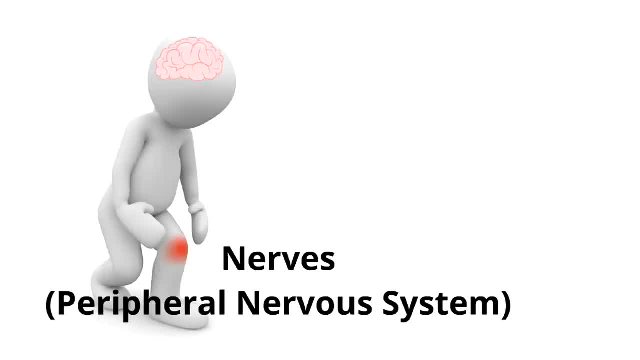 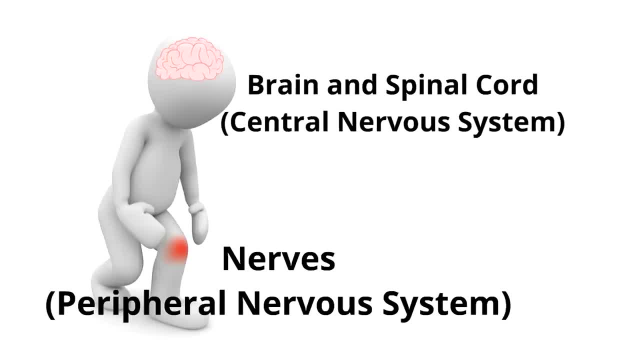 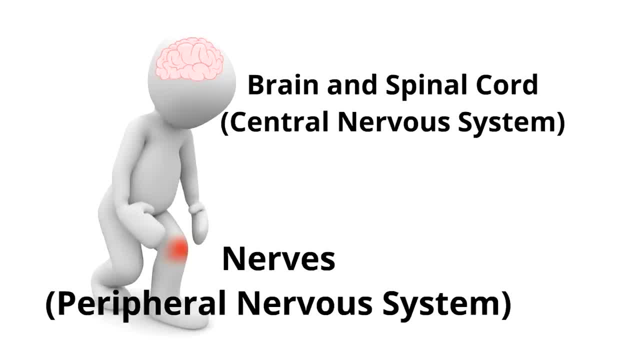 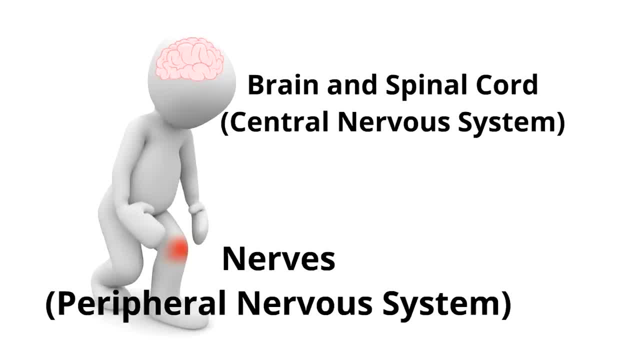 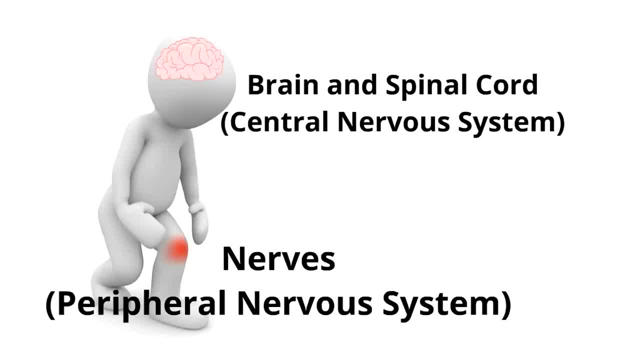 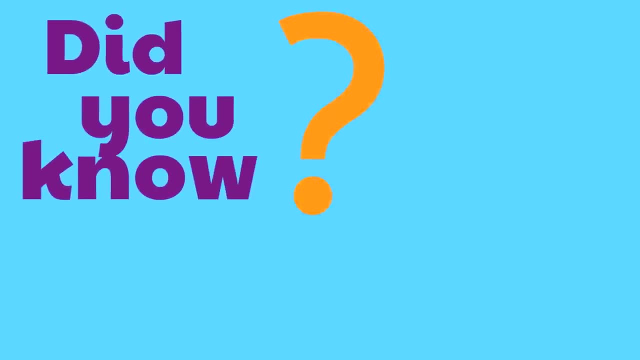 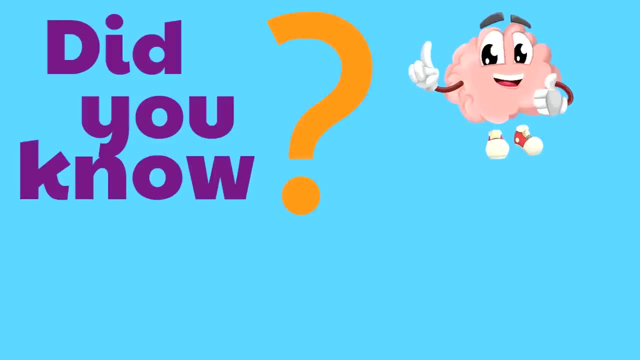 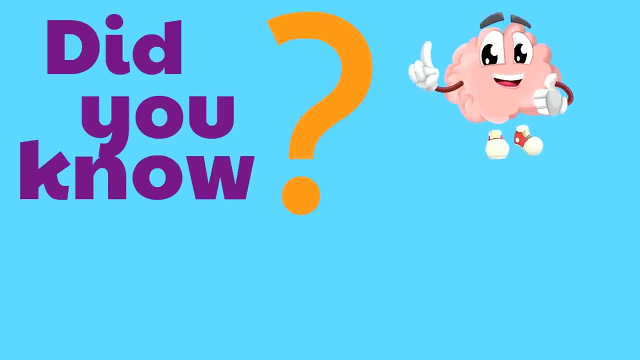 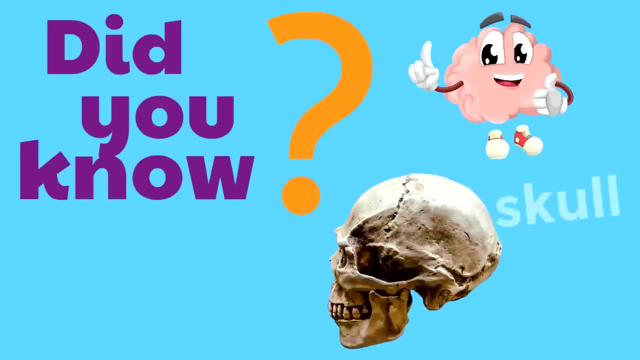 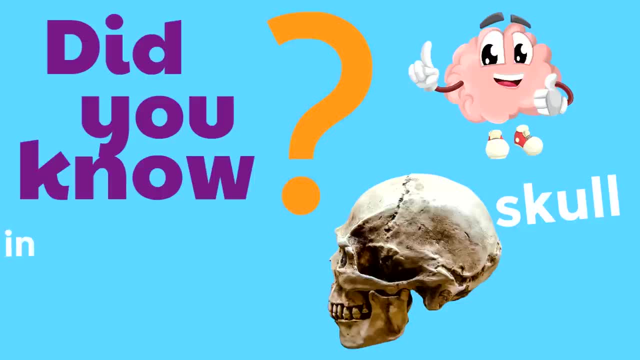 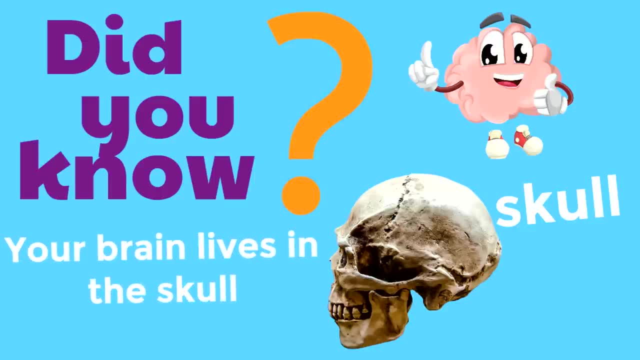 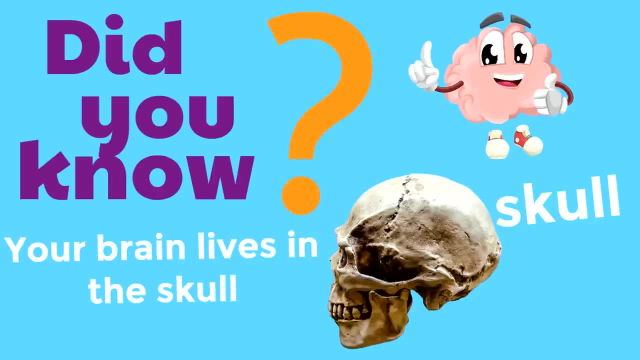 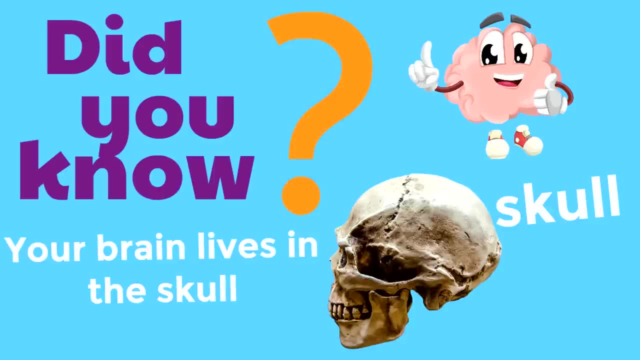 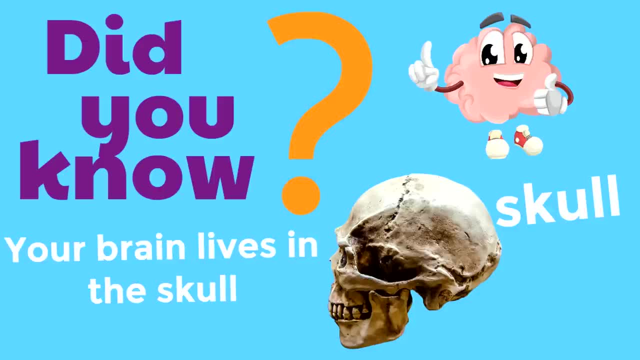 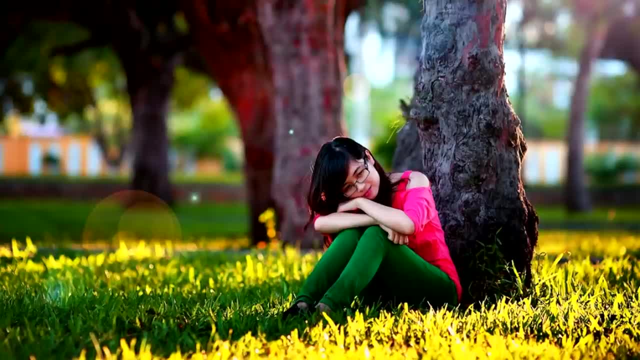 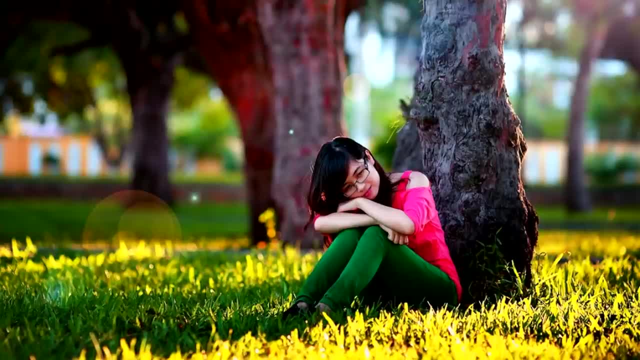 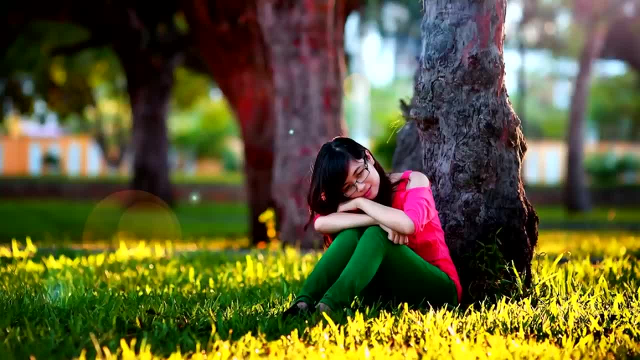 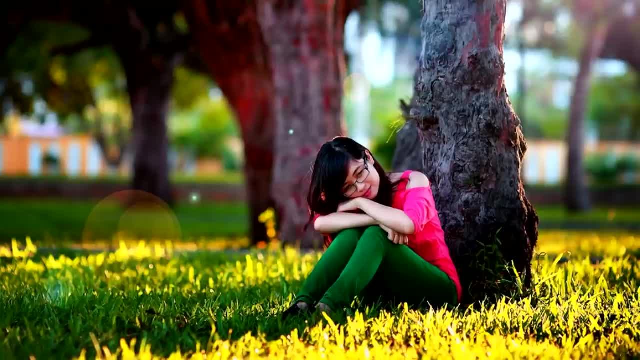 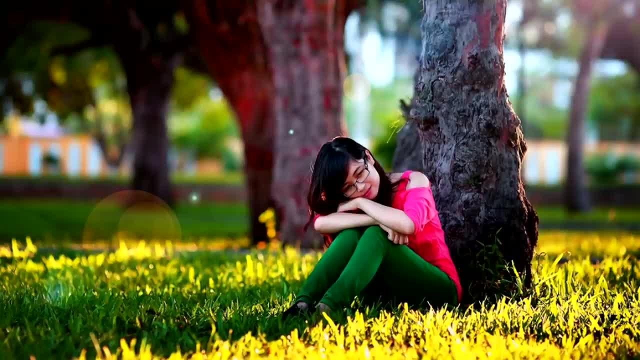 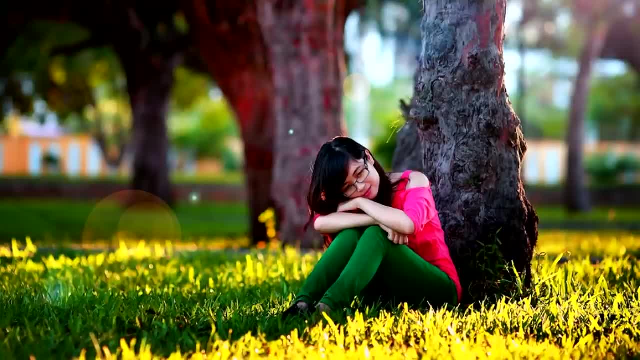 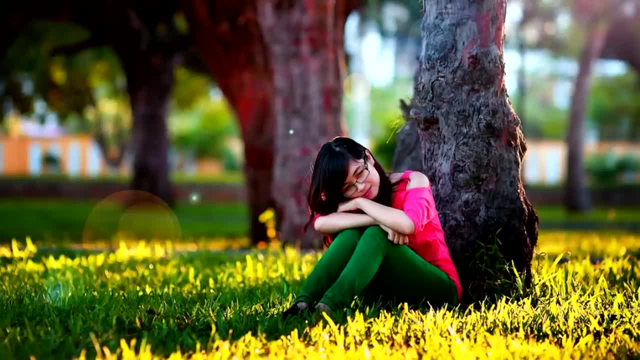 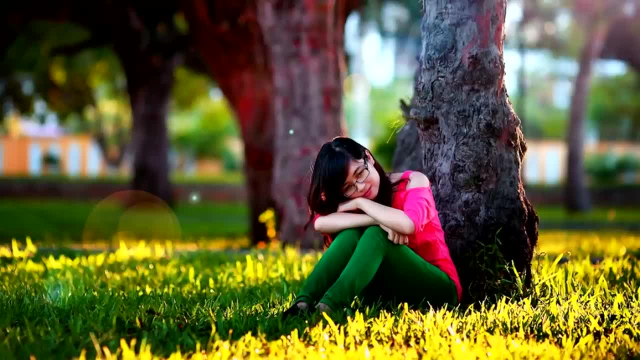 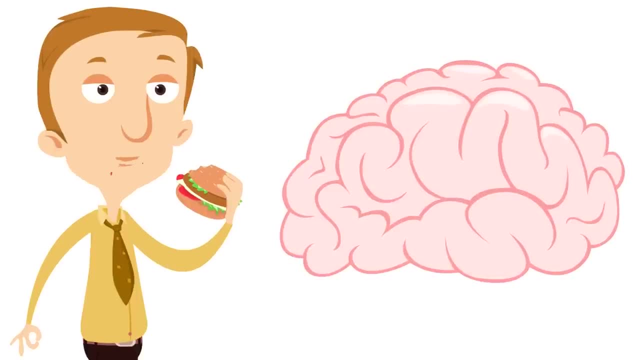 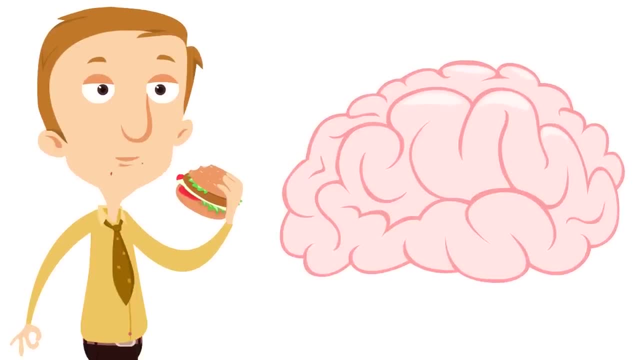 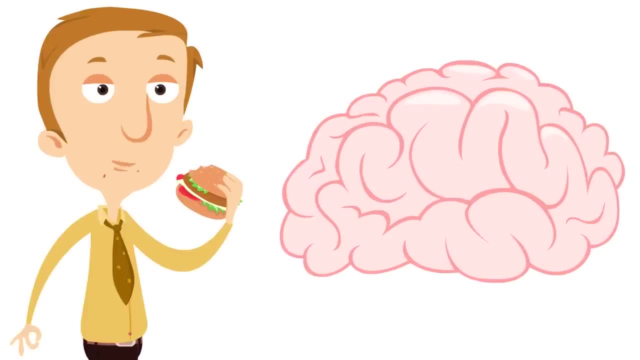 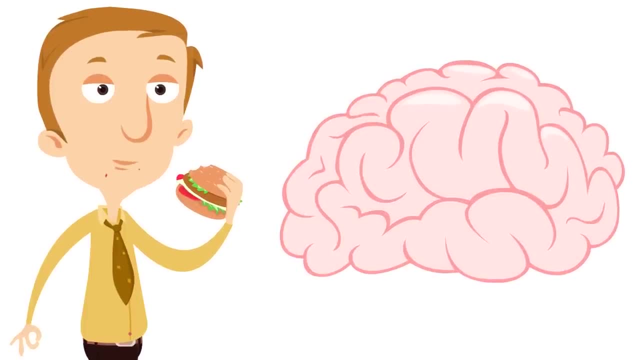 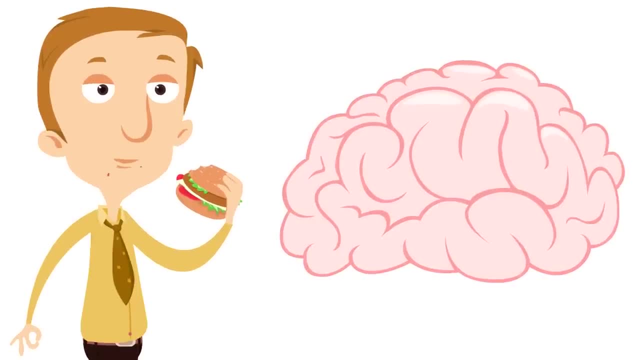 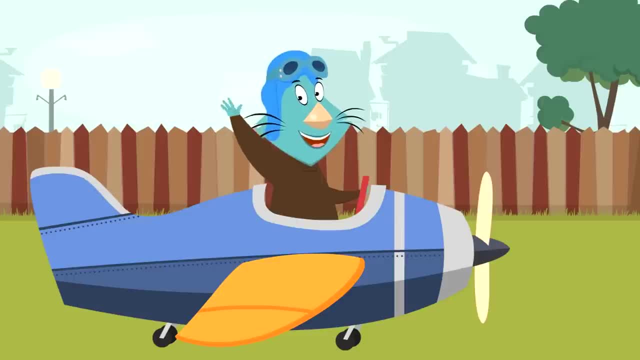 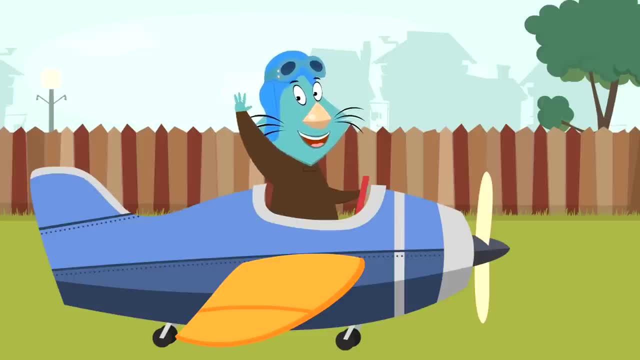 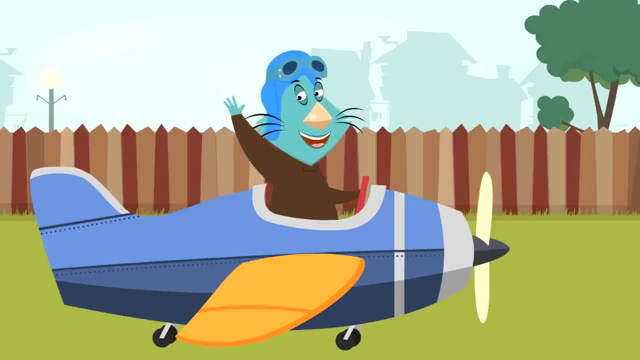 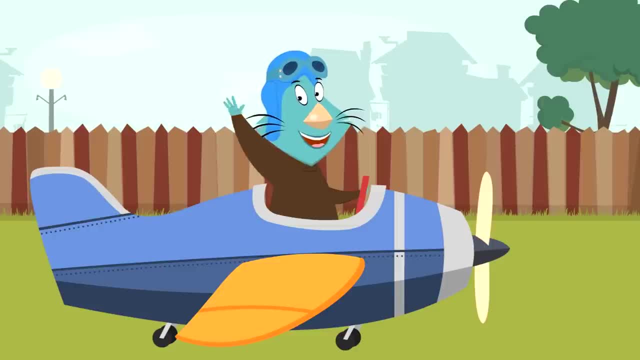 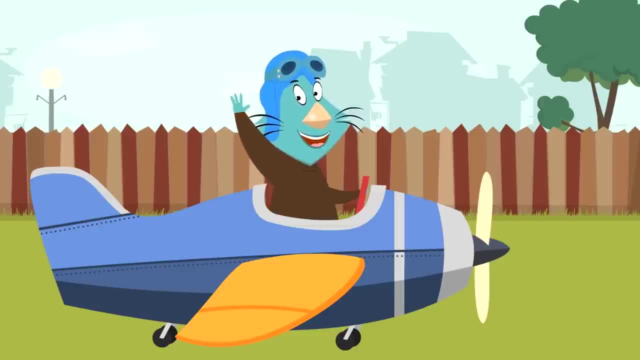 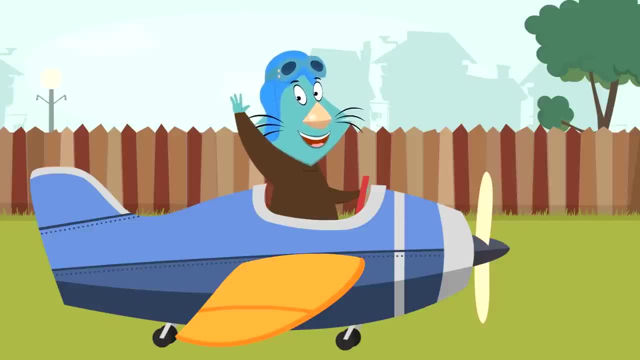 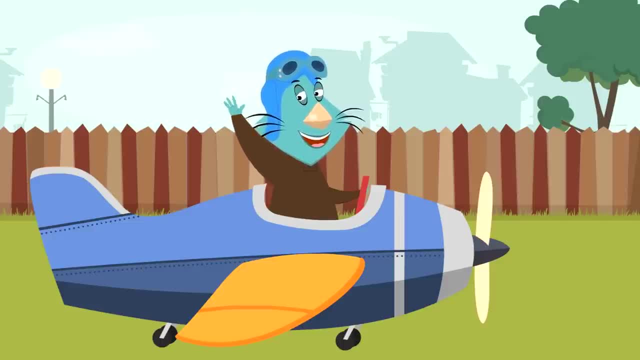 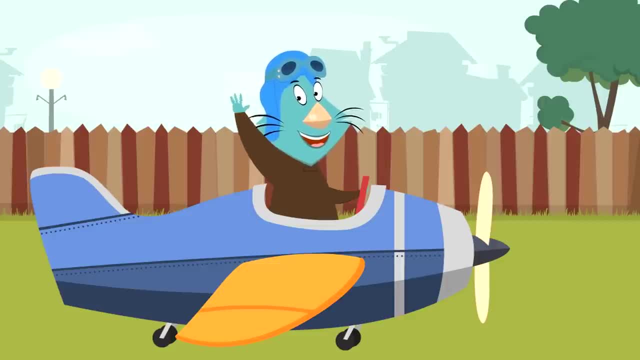 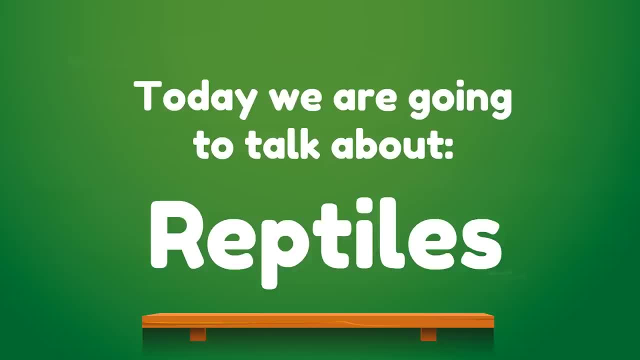 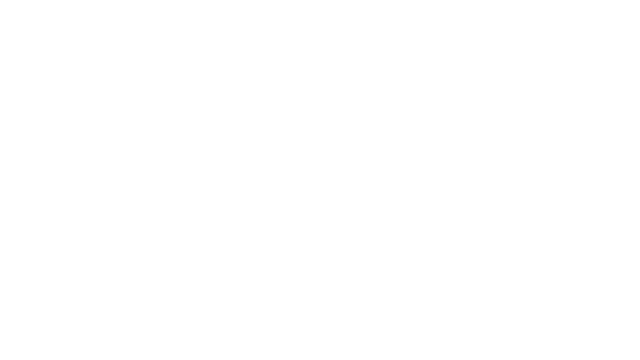 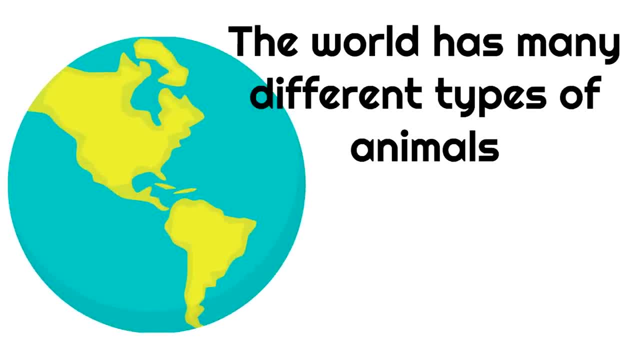 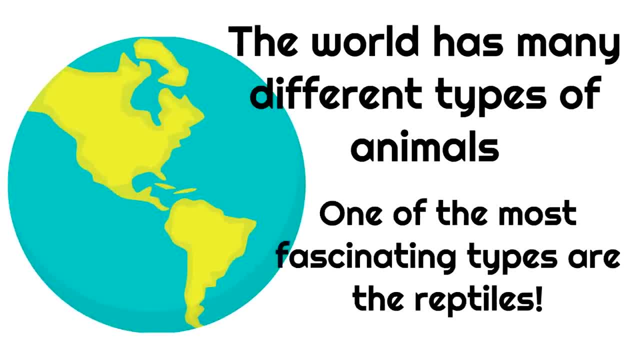 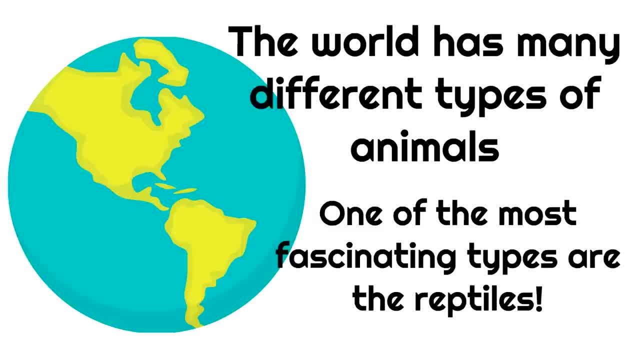 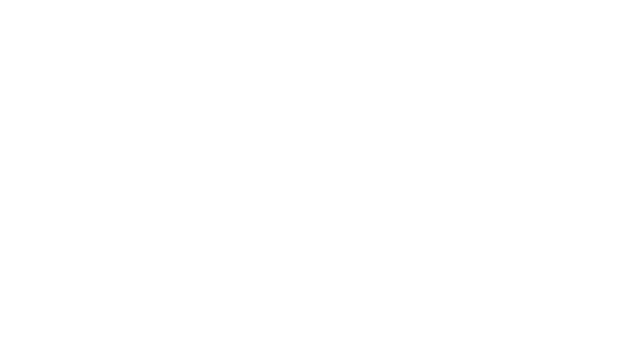 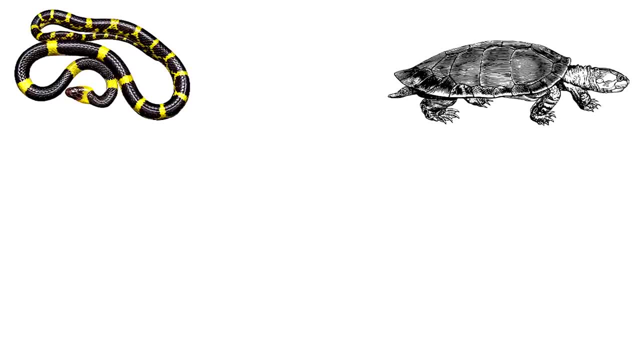 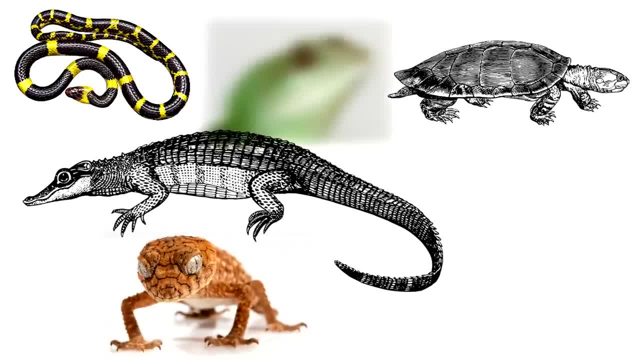 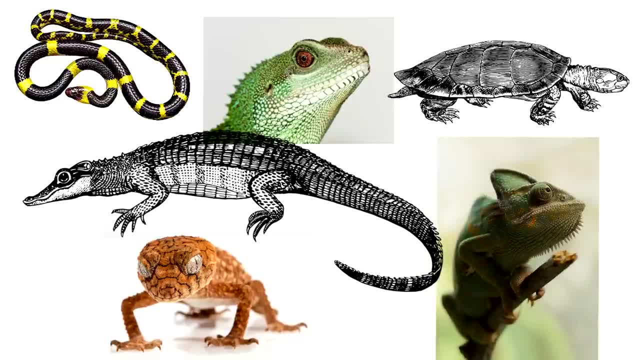 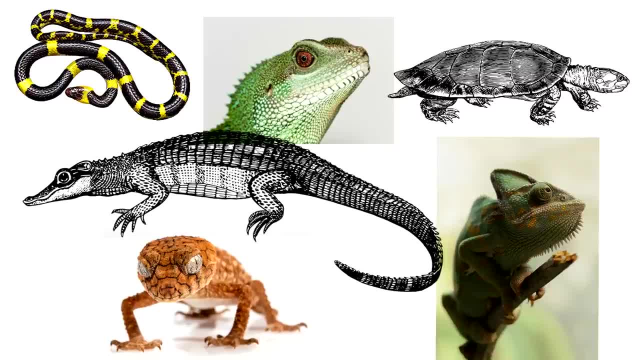 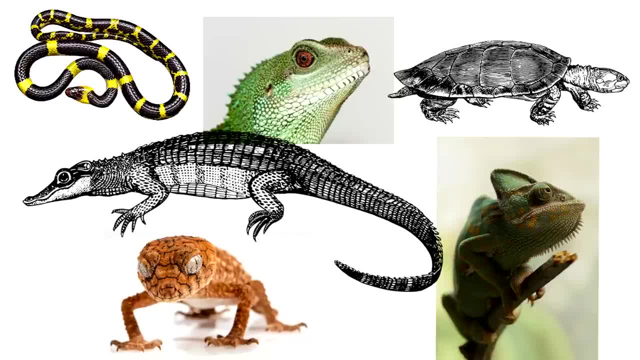 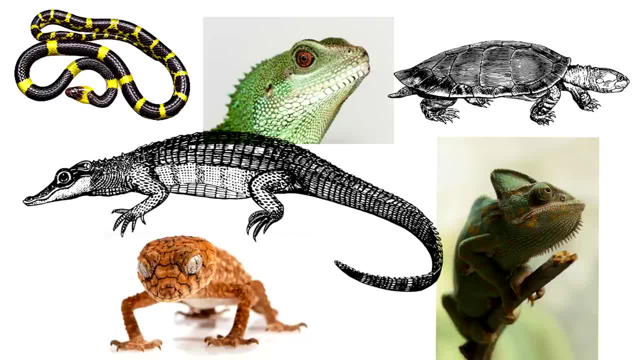 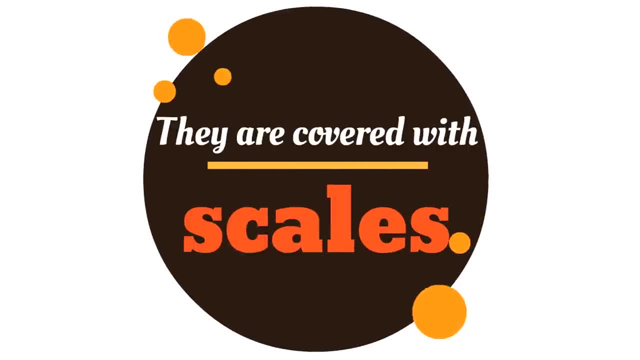 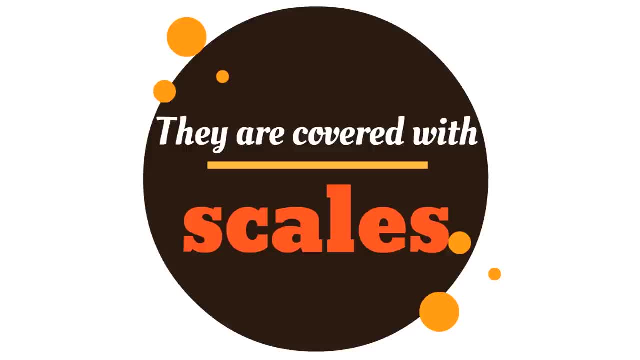 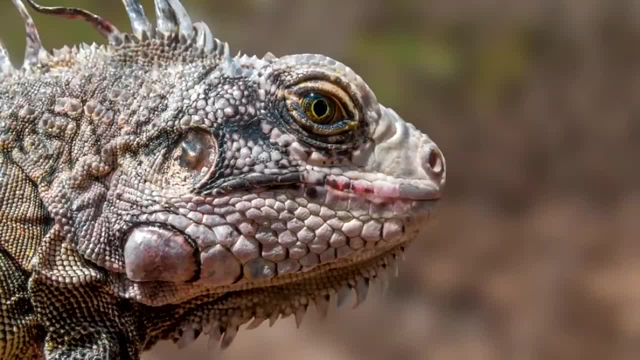 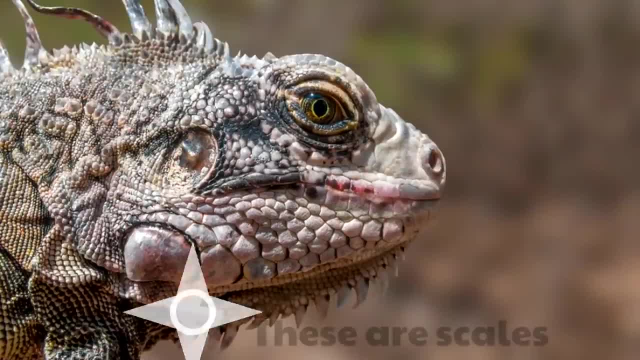 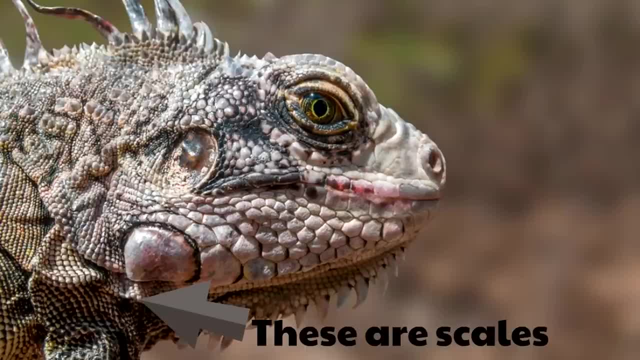 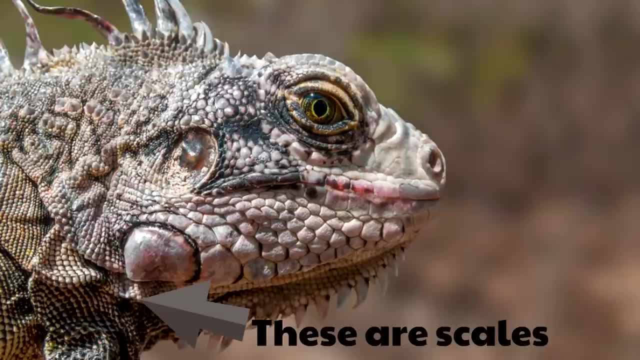 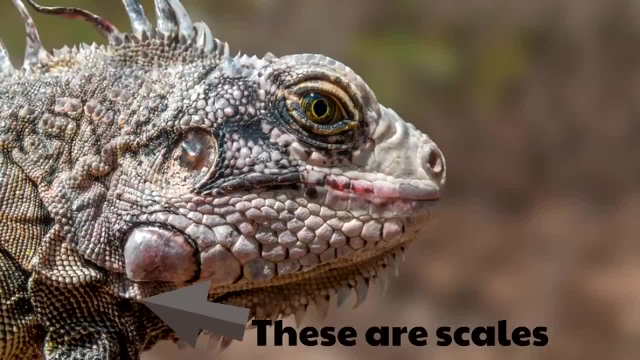 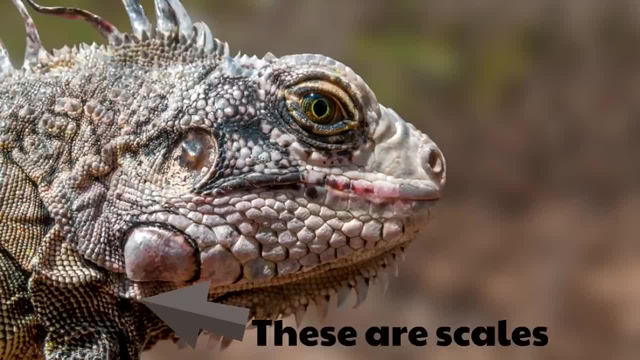 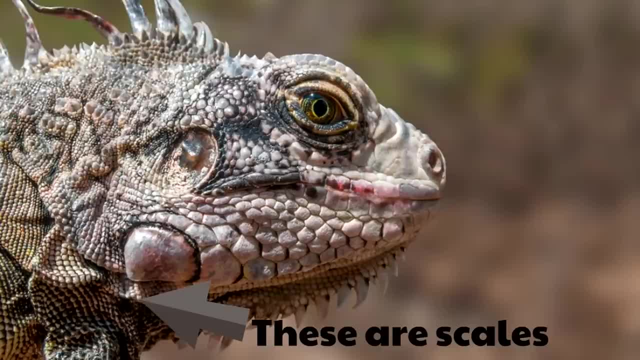 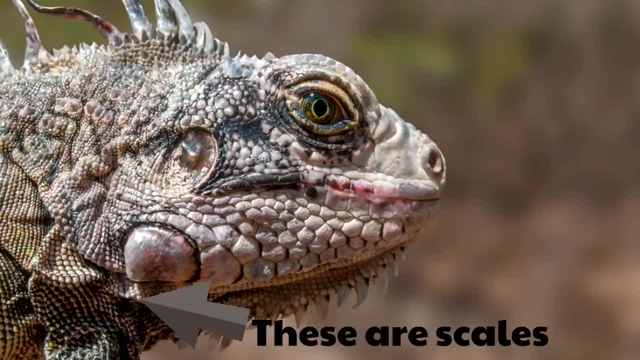 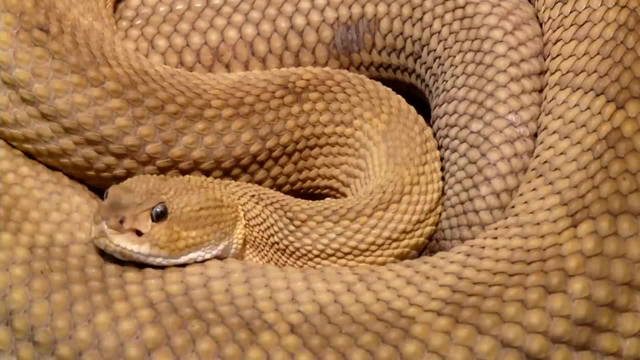 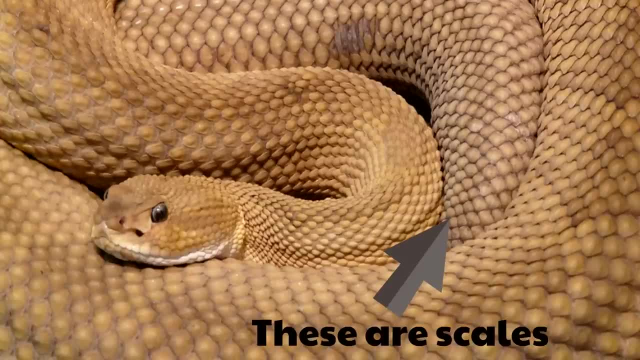 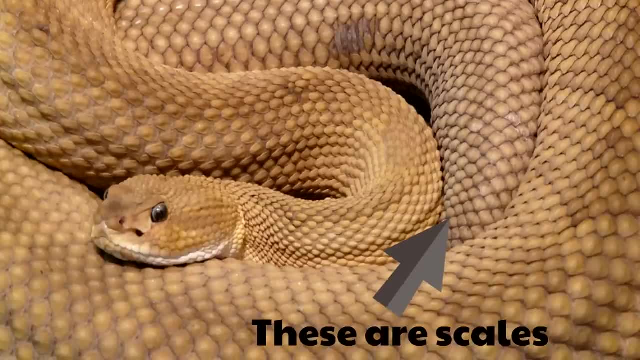 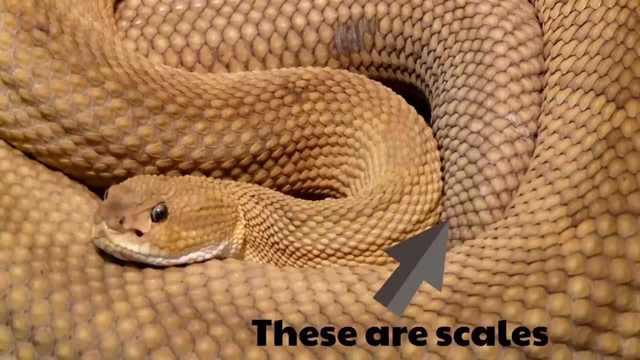 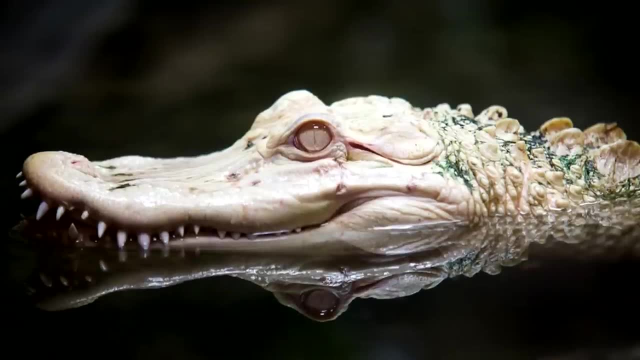 specific jobs for your body. see, the brain is a special group of tissues that do, absolutely covered with these intricate scales. Here's an interesting example of scales. This is an albino alligator, which means the alligator is very pale And you can see that this alligator is covered with scales. 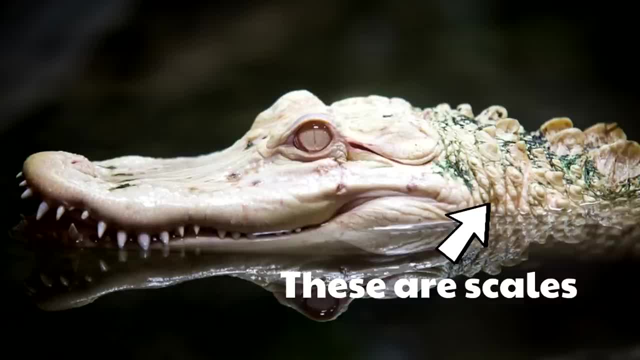 but the alligator also has these bony plates on his back. You can kind of see them there in the corner. Those are not scales, but reptiles also can have those bony plates, but this alligator is still covered with scales. 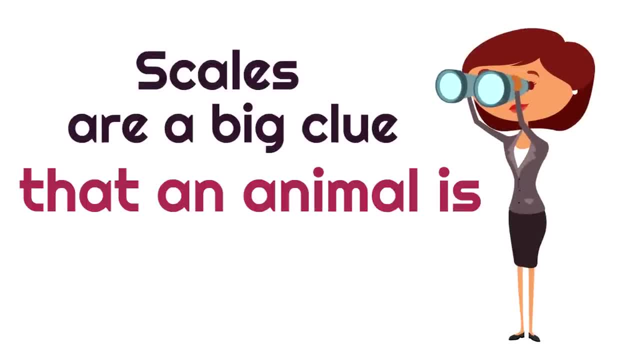 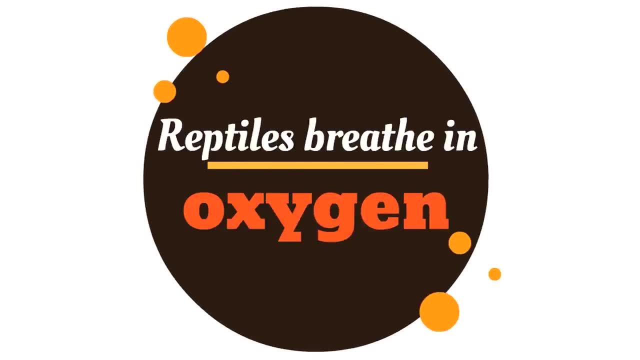 Scales are a big clue that an animal is a reptile. The second thing you need to know about reptiles is reptiles breathe in oxygen, Just like we breathe in oxygen. reptiles have to breathe in oxygen to survive Now, just like people. 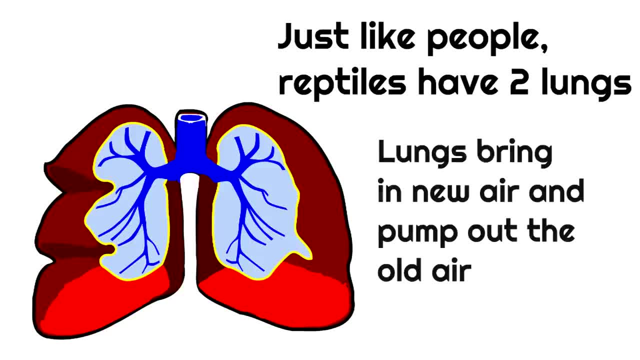 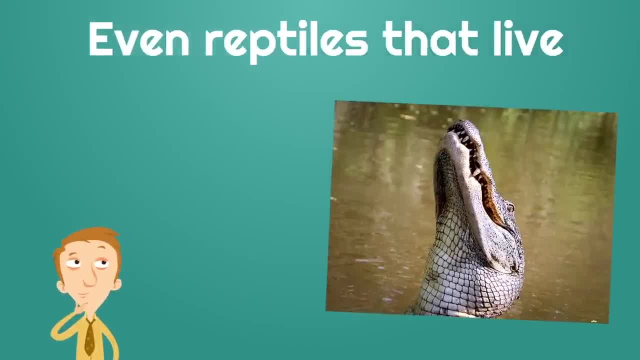 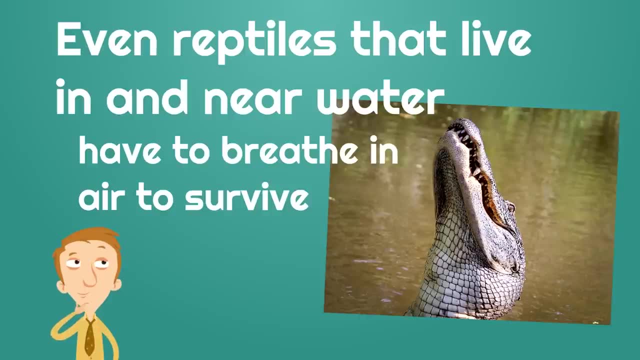 reptiles have two lungs in their body. Lungs bring in new air and pump out the old air. Even reptiles that live in and near water, like crocodiles and alligators, have to breathe in air to survive. Now, this is so fascinating. 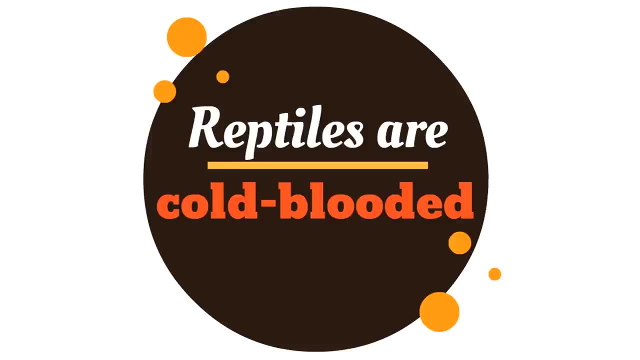 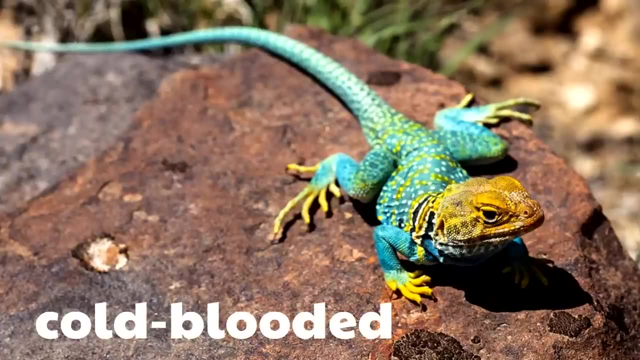 Did you know reptiles are cold-blooded. Cold-blooded means that their bodies don't keep them warm automatically. They have to have sunlight to keep them warm. Here's a picture of a lizard that's soaking in some sunlight. This is very important for this lizard. 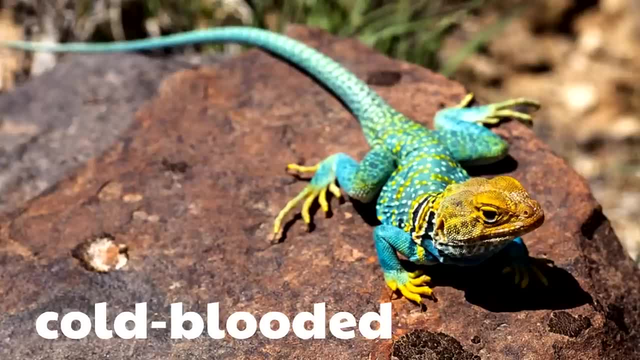 because, as with all the other reptiles, this lizard is cold-blooded. That means that the temperature of the lizard needs to have sunlight to keep it warm. It doesn't warm automatically. This lizard is cold-blooded. Here's a snake that's in the sunlight. 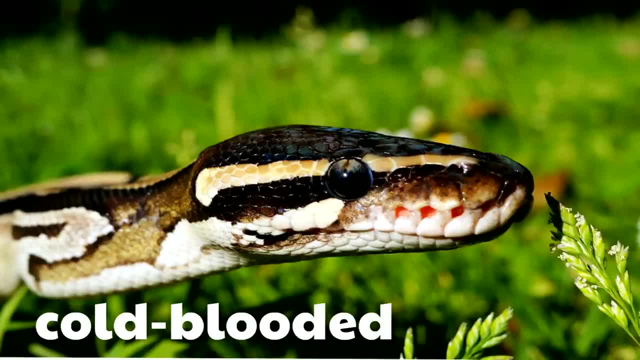 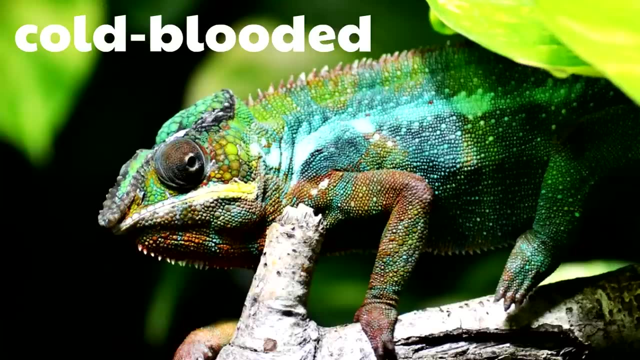 The sunlight is helping to warm the body of this snake. This doesn't happen automatically with the snake's body, because the snake is cold-blooded just like the other reptiles. Hey, here's a picture of a chameleon. Chameleons are just so cool. 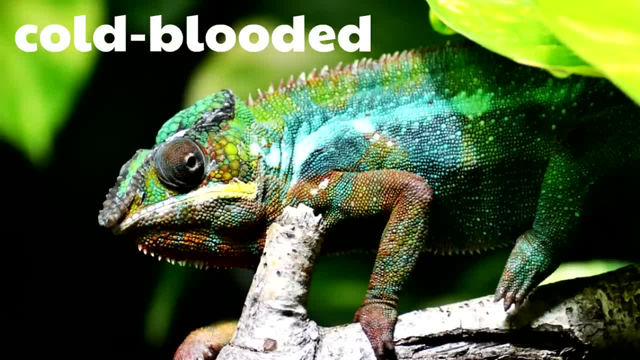 Now, of course, this chameleon is cold-blooded Because all of the reptiles are cold-blooded. If they want to get warmer, they have to go to the sunlight, because their bodies don't warm them. They're cold-blooded. 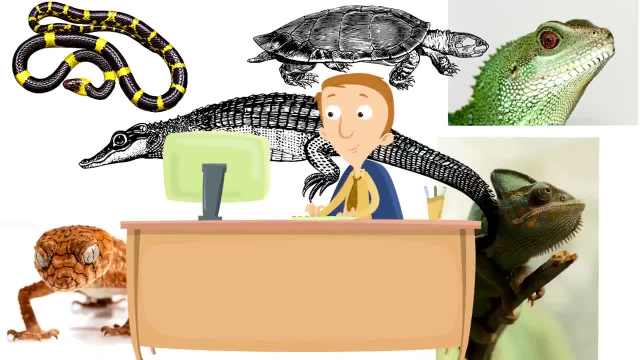 Wow, I mean right. I mean, these are incredible creatures. You know, reptiles. they're covered in these dry, waterproof scales. They breathe in oxygen with those two lungs, like we do. They're cold-blooded, which is so fascinating. 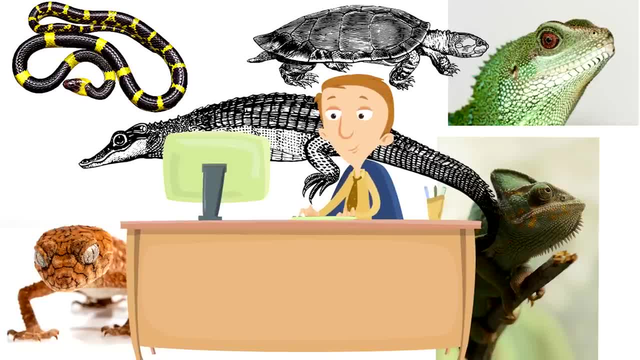 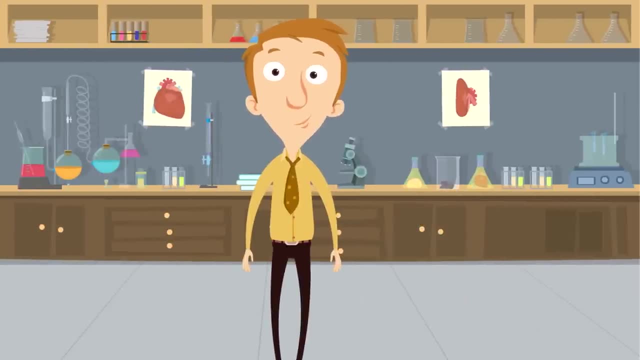 Can you imagine having to lay out in the sun if you wanted to warm your body, Instead of your body being able to do it on its own? These are fascinating creatures. Hey, do you have a favorite reptile? It's OK, You don't have to tell me. 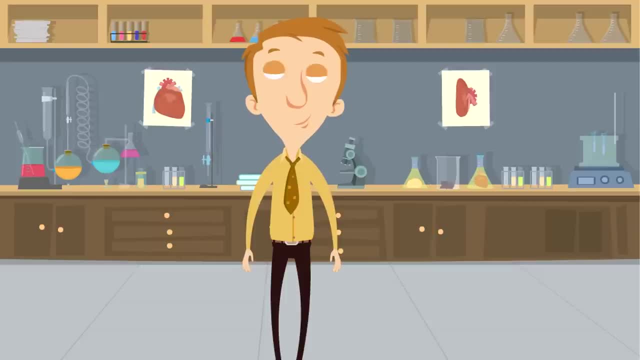 Cool, Very cool. Yeah, it's, you know, you figure snakes, turtles, crocodiles, alligators, geckos, lizards, chameleons, reptiles, reptiles are just the coolest, aren't they? 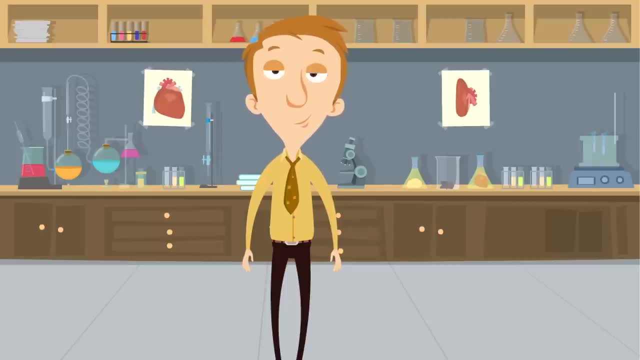 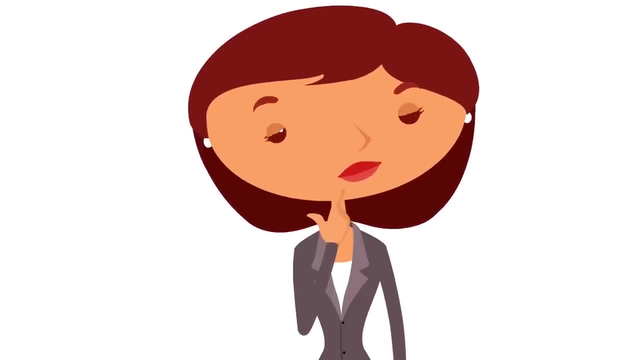 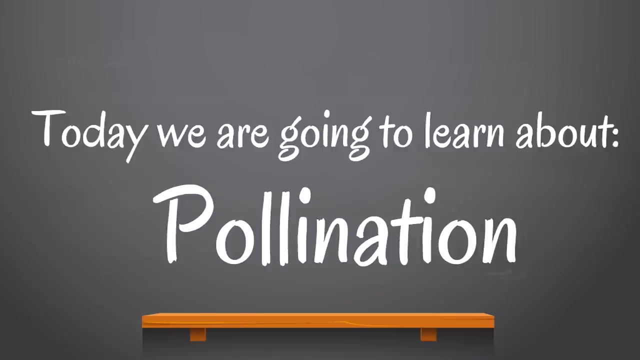 I mean, they're just absolutely amazing. Hey, when is it going to be my turn? I want to be in this compilation video too. OK, let's see I'm going to teach about pollination. Hi, look at all these beautiful flowers that I've found. 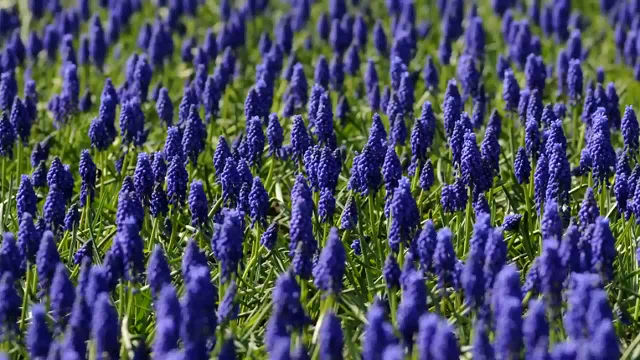 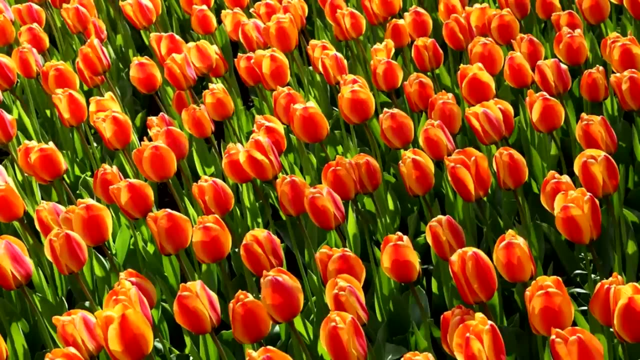 Let's look at some more. These flowers are so sweet, Pretty. Look at how blue-y, purple-y they are. They're just so beautiful. And these ones are so red and, oh, excuse me, These ones are so red and brilliant. 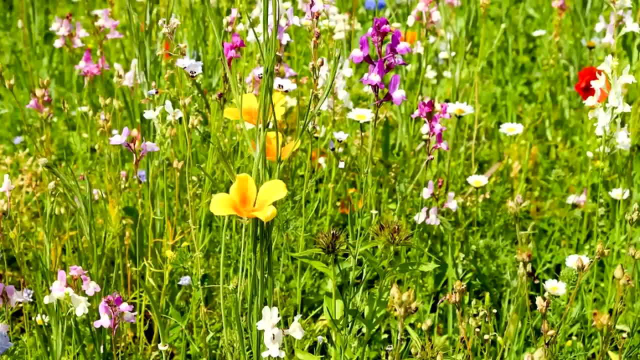 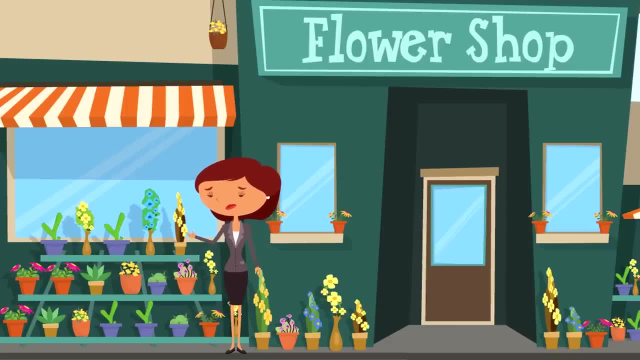 And look at all the pretty colors. It's so, it's so beautiful. I love these flowers, but all the pollen is making me sneeze And sniffily, So I think we should go back inside. All right, that's better. 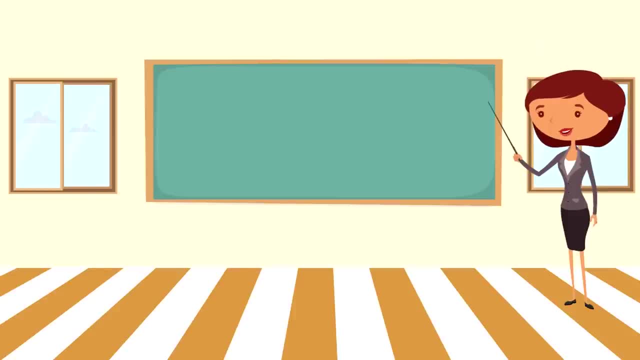 Well, flowers, they make pollen, And pollen is a fine powder. It's usually yellow and it can make you sneeze, just like me earlier. Flowers use pollen to make seeds through a process called pollination. OK, do you see these yellow feathery parts of the flower? 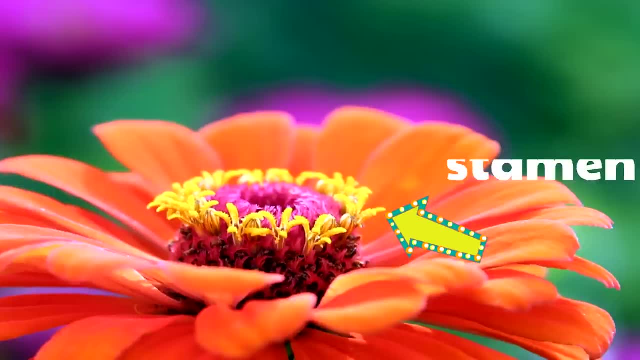 This is the flower. Oh yeah, This is the male part of the flower, called the stamen, And that is where the pollen is made. Now, this middle pink part of the flower is called the pistil, which is the female part. 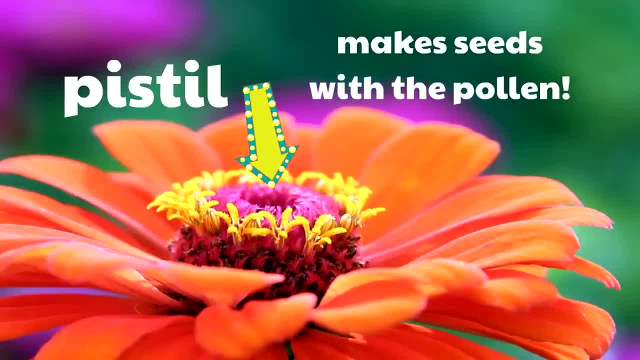 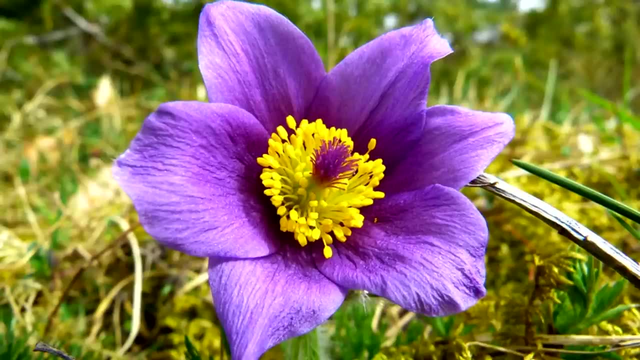 of the flower. This is where the pollen needs to go, so the flower can make seeds. Looking at this flower, do you think the yellow parts are the stamen or the pistil? Oh yeah, Yeah, That's right, That's the stamen. 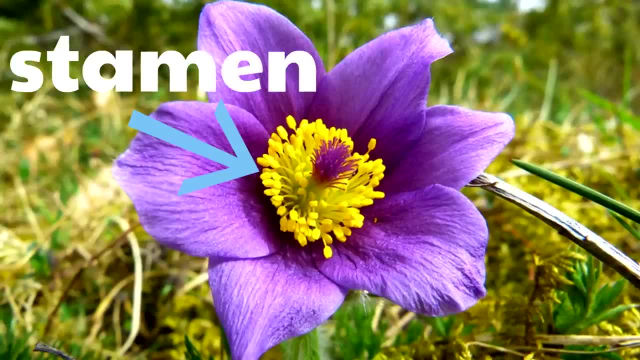 The stamen is the male part of the flower, That's the part that makes pollen. Now here's a different flower. Do you think this purple part in the middle is the stamen or the pistil? Very good, That's the pistil. 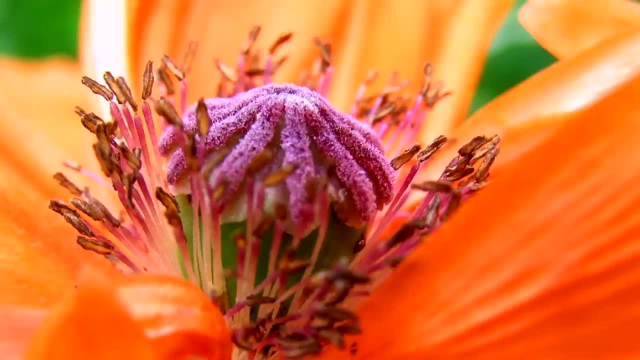 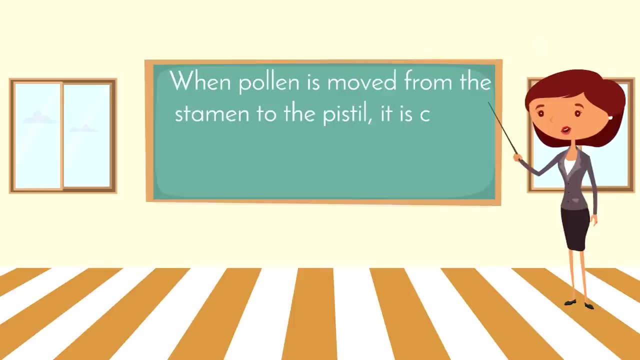 The pistil is the female part of the flower, where the pollen needs to go so that the flower can make seeds. When pollen is moved from the stamen to the pistil, it is called pollination. There are flowers that have both a stamen and a pistil, but there are some flowers that 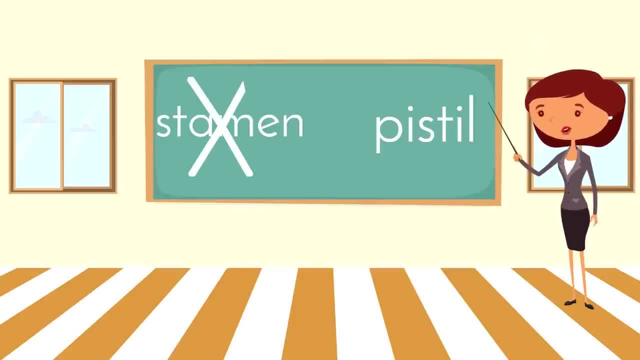 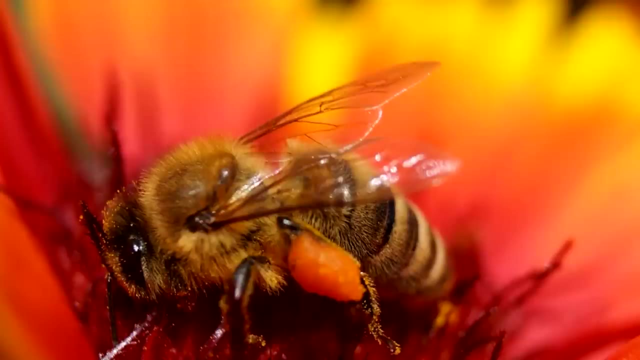 have only a pistil and there are other flowers that have only a stamen. Pollen can't move by itself, so how will it get to the pistil With the help of pollinators? Do you recognize this well-known pollinator? 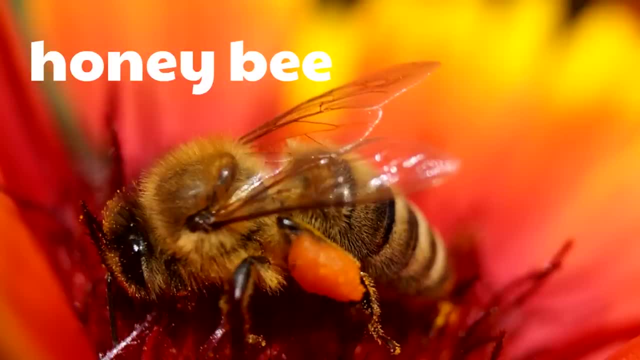 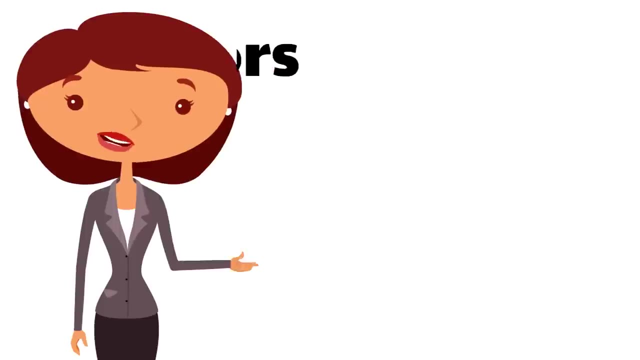 Very good, That's a honeybee. Honeybees are pollinators and you can see the yellowy-orange pollen on his leg right here. Pollinators are pollen helpers by moving the pollen to the pistil so the flower can make. 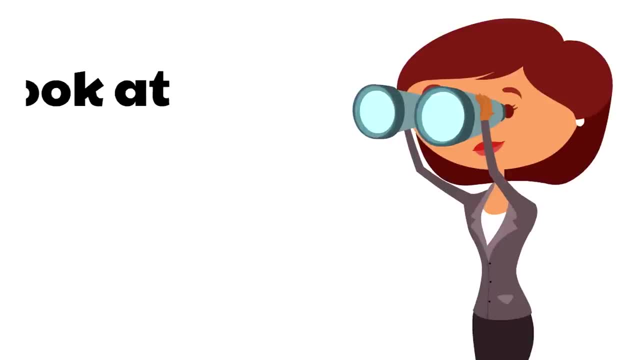 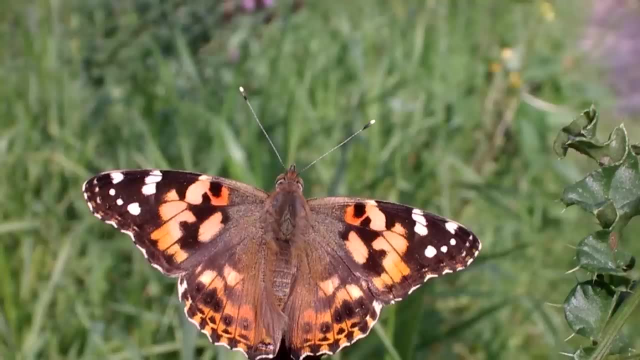 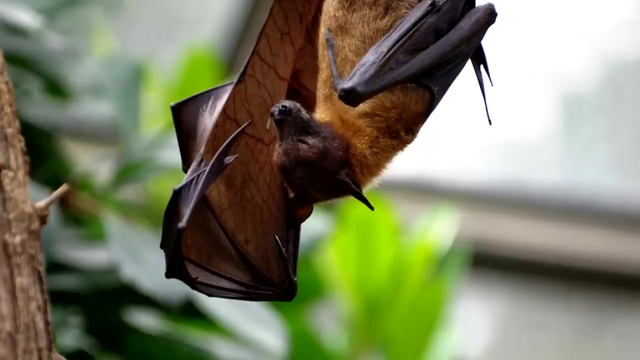 seeds. Let's look at some other pollinators. Do you know what this pollinator is called? That's right, This is a butterfly and this one is called a painted lady butterfly. Butterflies are pollinators. What kind of animal is this? 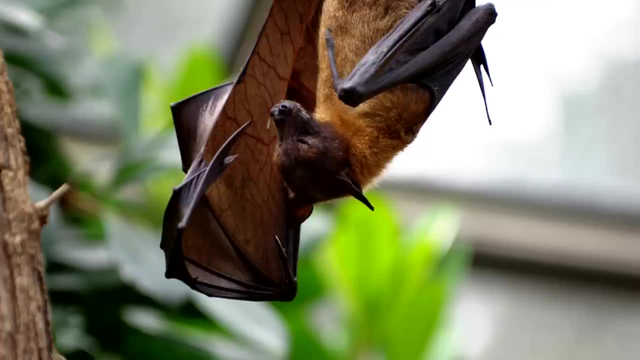 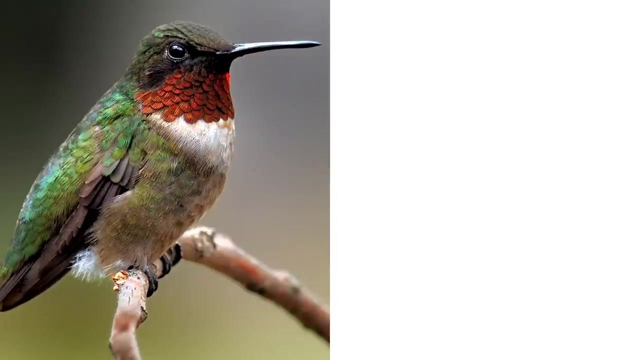 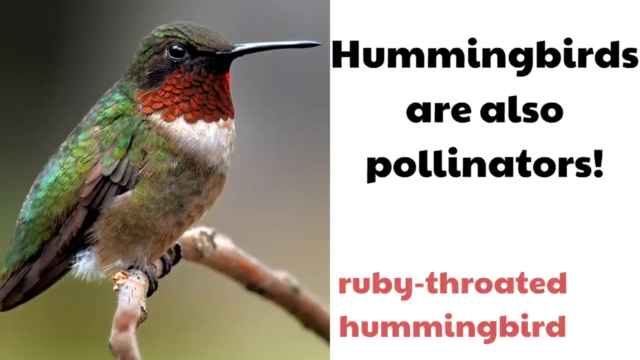 That's right, That's a bat. This is a flying fox, which is a fruit bat, and fruit bats are pollinators too. What's this little guy called Great job? This is a hummingbird. It's a ruby-throated hummingbird, and hummingbirds are also pollinators. 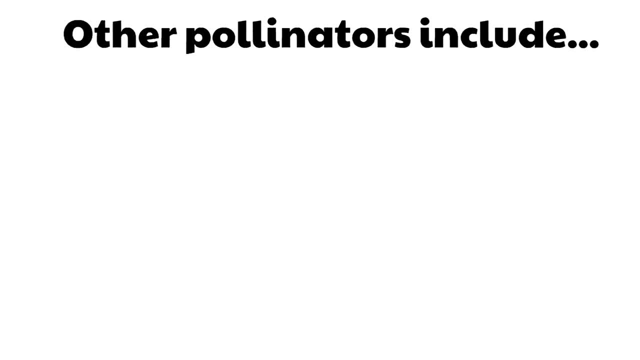 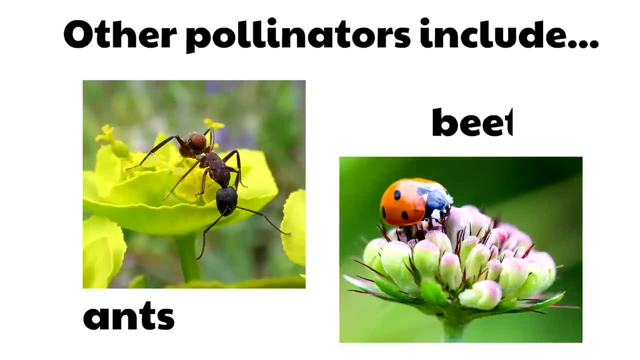 Other pollinators include wasps and moths. Ants and beetles- like this ladybug- are pollinators too. These other pollinators are bees. They're pollinators too. Other pollinators are very well known. 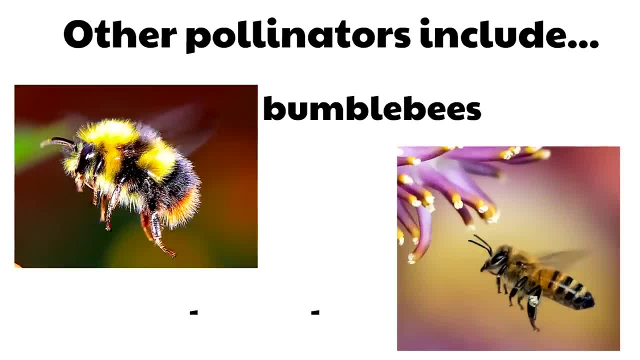 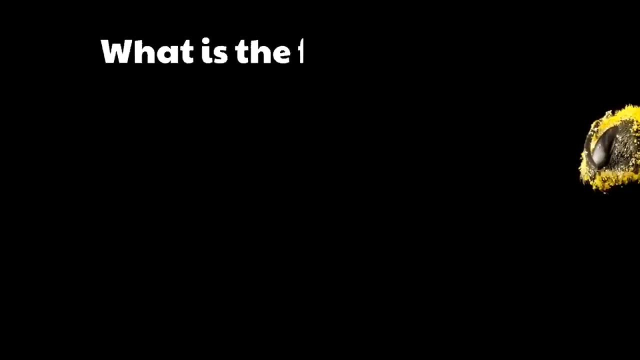 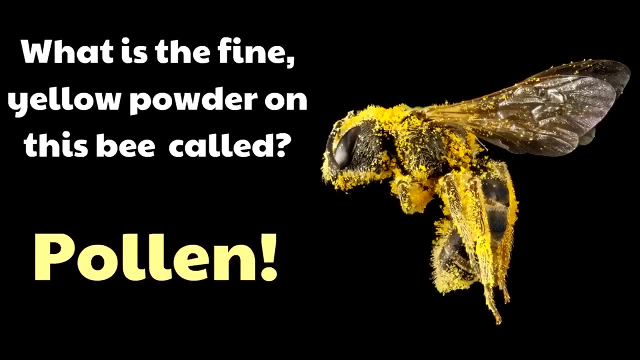 They are bumblebees and honeybees. All right, Let's review what we've learned today. What is the fine yellow powder on this bee called? That's right, It's pollen. Pollen is a fine yellow powder. This yellow part of the flower makes pollen. 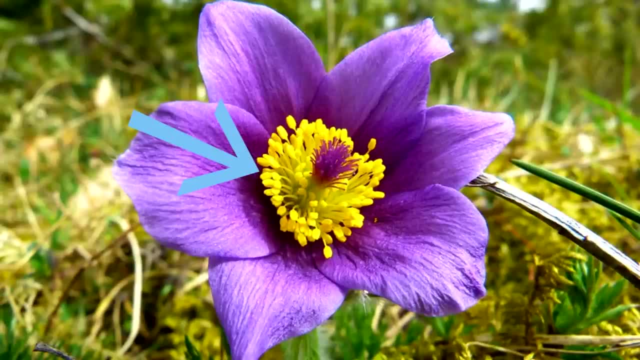 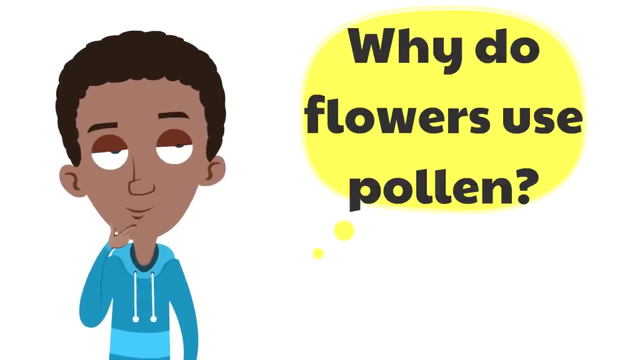 Do you remember what it's called? That's right, That's the stamen. The stamen is the male part of the flower. That's the part that makes pollen. Why do flowers use pollen? Great job, Flowers use pollen to make seeds. 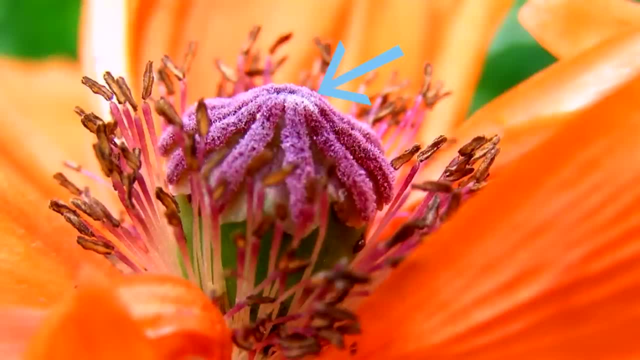 This purple part of the flower is where the pollen needs to go, so the flower can make seeds. Do you remember what it's called? Very good, That's the pistil. The pistil is the female part of the flower, where the pollen needs to go so that the flower can make seeds. What is the process called when pollen is moved from the stamen to the pistil? Great job. When pollen is moved from the stamen to the pistil, it is called pollination. What is the name of the pollen helpers? 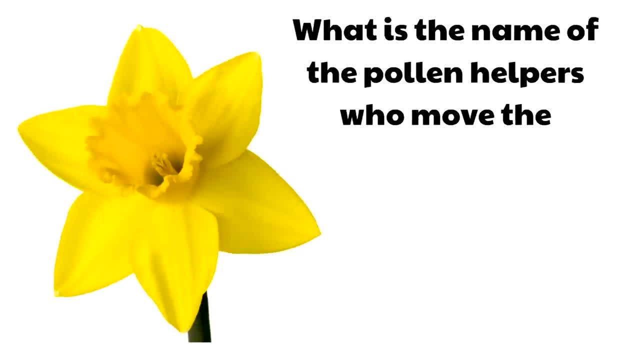 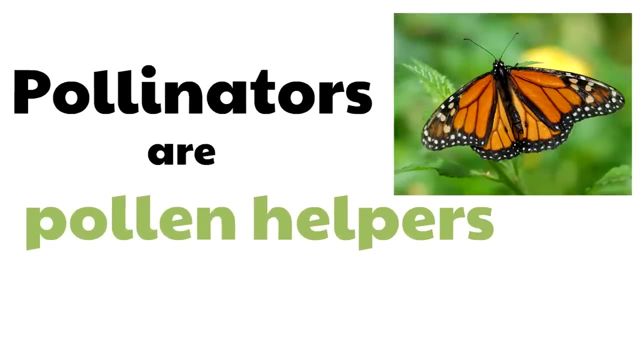 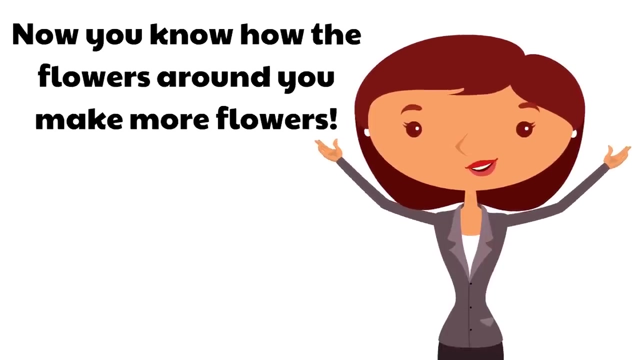 The pollen helpers are the pollen helpers who move the pollen so the flower can make seeds. That's right, They're called pollinators. Pollinators are pollen helpers by moving the pollen to the pistil so the flower can make seeds. Now you know how the flowers around you make more flowers. 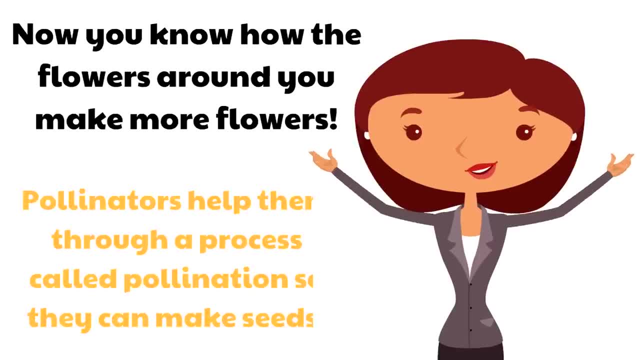 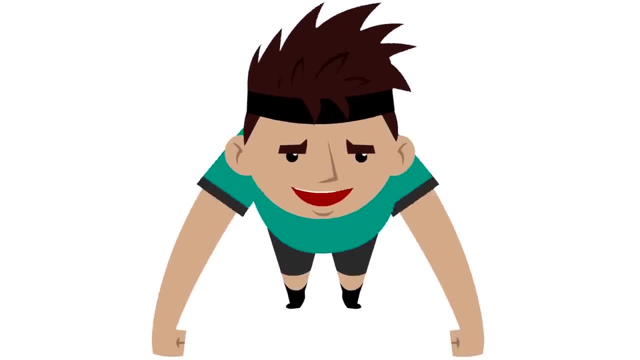 Pollinators, help them through a process called pollination so they can make seeds. You have been doing a great job, just like Mike, who's doing these push-ups. You know he knows it's important to stay fit and to exercise and to stay healthy and you're. 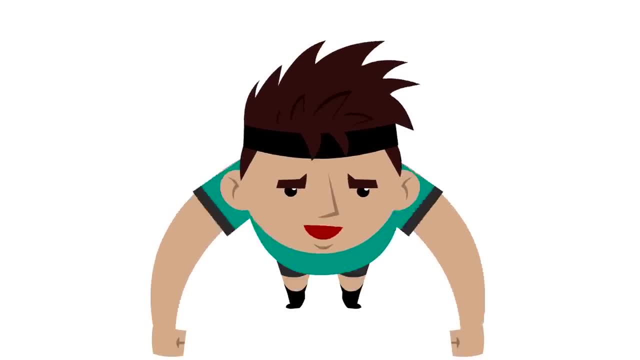 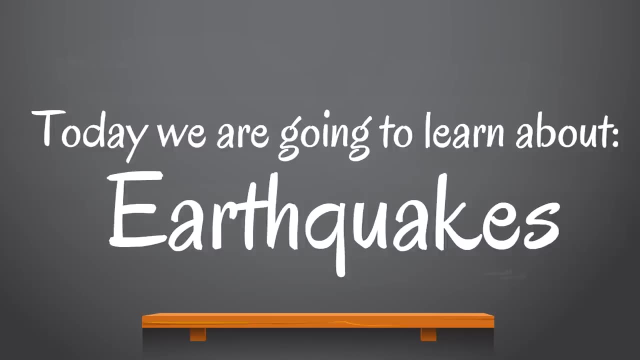 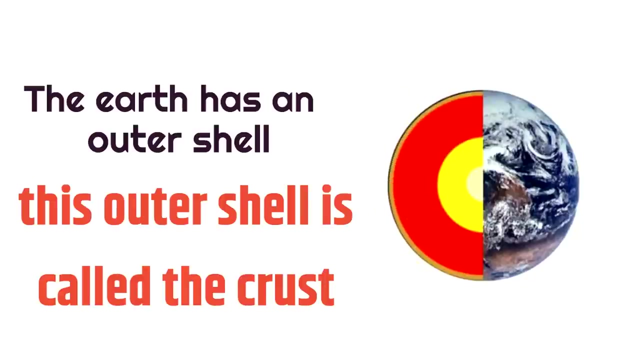 like exercising your mind right now, which is super cool. Next, we are going to learn about earthquakes, Earthquakes, Earthquakes, Earthquakes, Earthquakes, Earthquakes, Earthquakes. So the first thing we need to understand is: the Earth has an outer shell, isn't that? 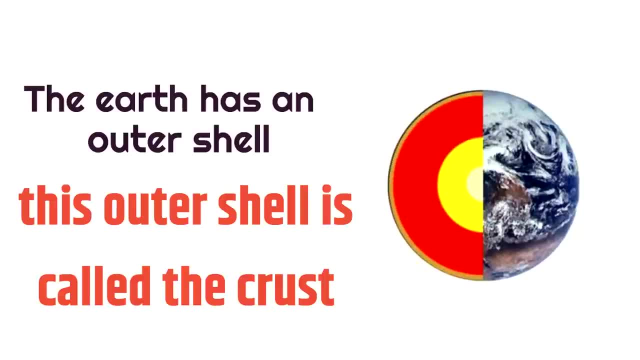 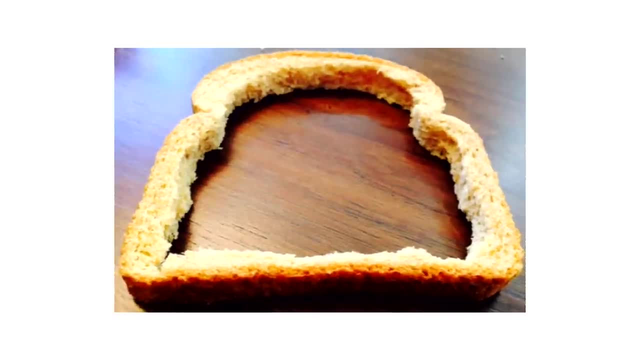 interesting. This outer shell is called the crust Crust, you know, like bread crust. I hope you enjoy bread crust, by the way, because you can't eat the crust of the Earth, but I hope that you're eating the bread crust, you know. 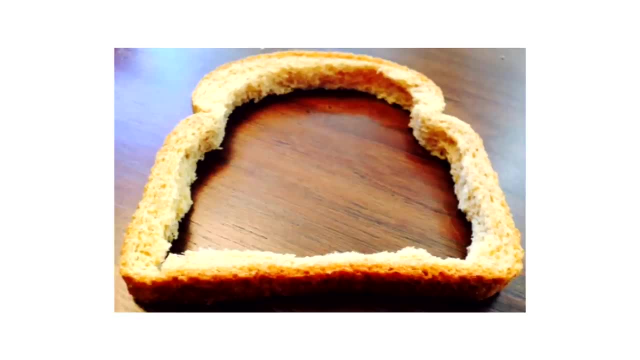 It's still yummy. It's on the outside, In fact. it's really healthy. It's really great. Okay, let's get back to the crust of the Earth. You know you don't eat the Earth's crust. hopefully you eat this kind of crust. okay, the surface of the earth is part of. 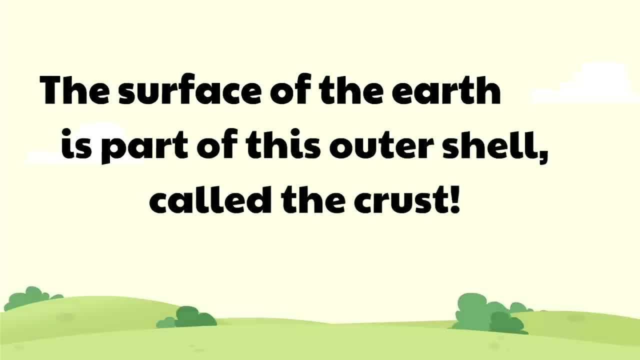 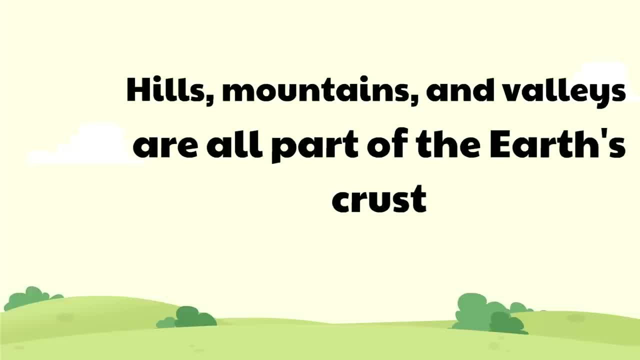 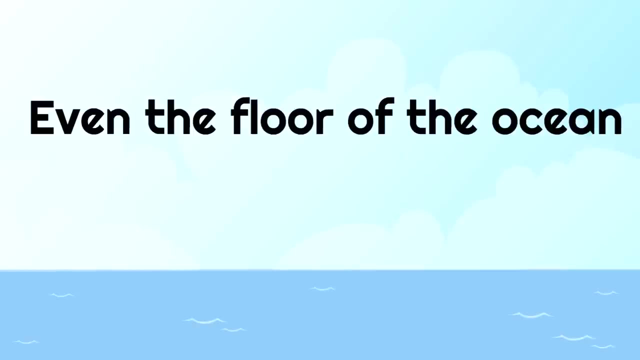 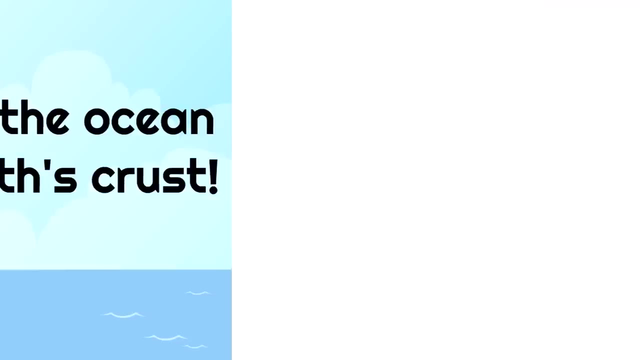 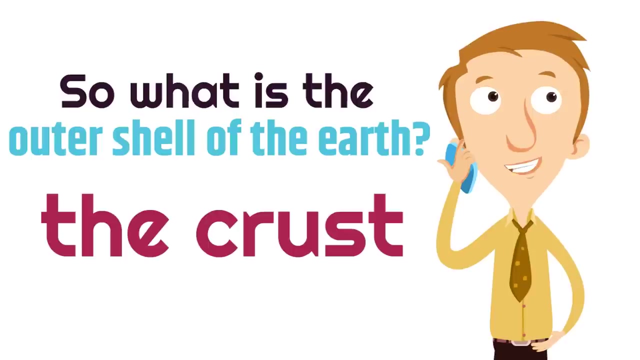 this outer shell. remember, the outer shell is called the crust. this means that hills, mountains and valleys are all part of the Earth's crust. that means even the floor of the ocean is part of the Earth's crust. so what is the outer shell of the earth? yeah, the crust. and you know it's fascinating. the crust has 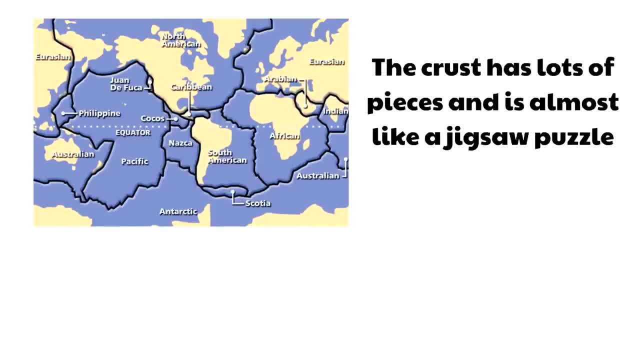 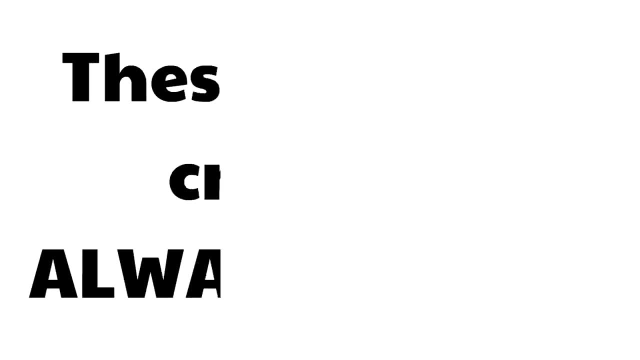 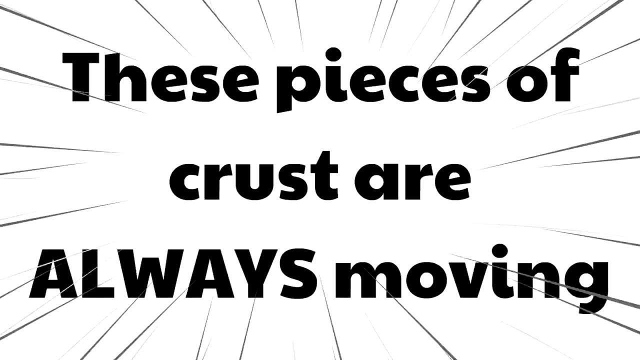 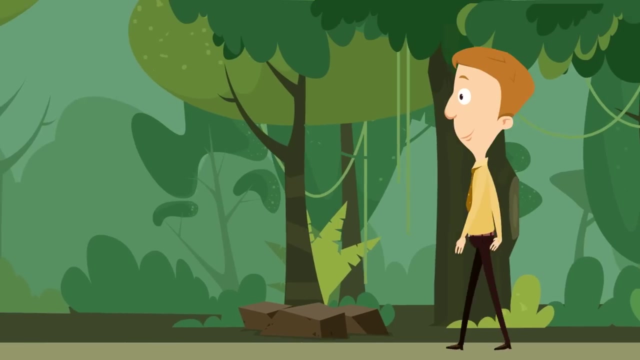 lots of pieces and is almost like a jigsaw puzzle, and you might not realize this, but these pieces of crust are always moving. in fact, they're moving right now. the pieces of crust that are below you right now are moving. they're always moving. now, usually the crust moves slowly. it doesn't move very fast. 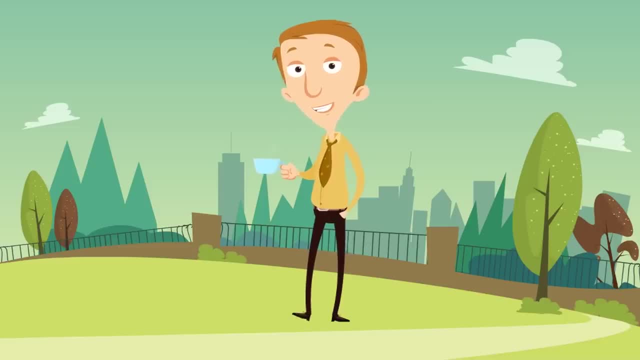 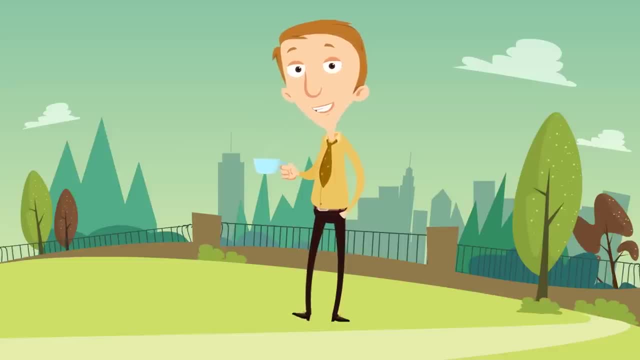 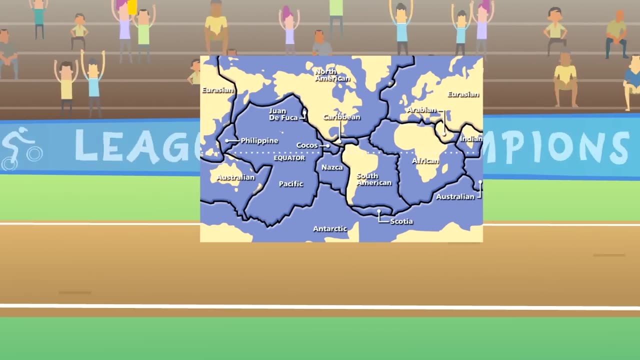 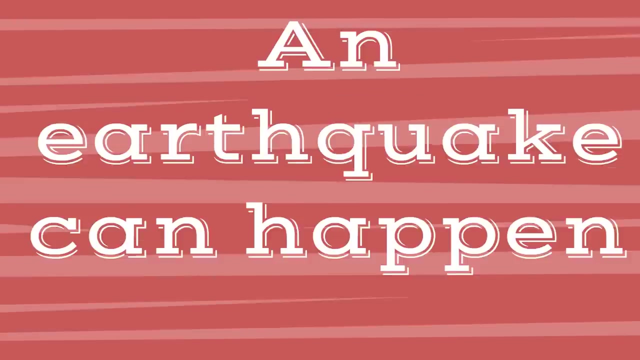 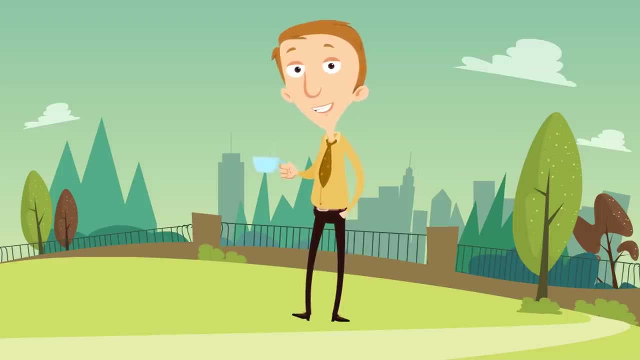 feel it. sometimes, however, the pieces of crust can move really fast. they can move quickly. when the pieces of crust are moving quickly, an earthquake can happen. so, when the pieces of crust move slowly, you don't feel it, but when the pieces of crust move quickly you could have an earthquake. 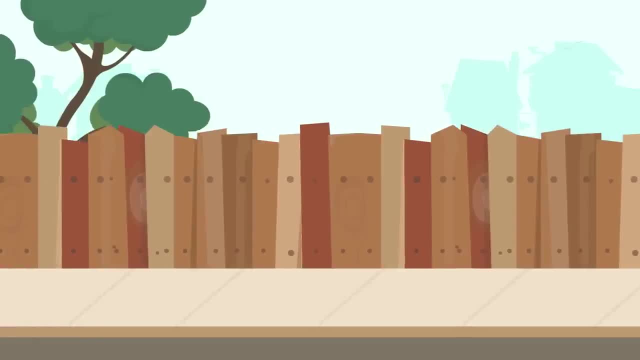 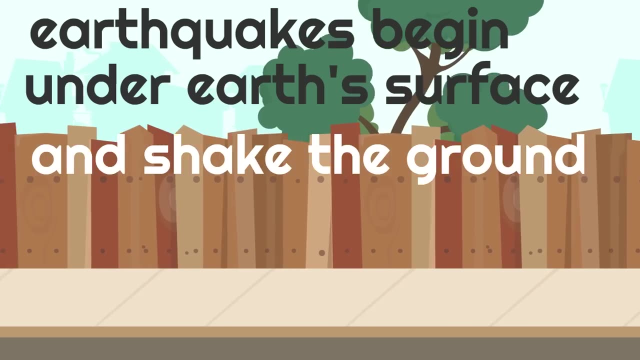 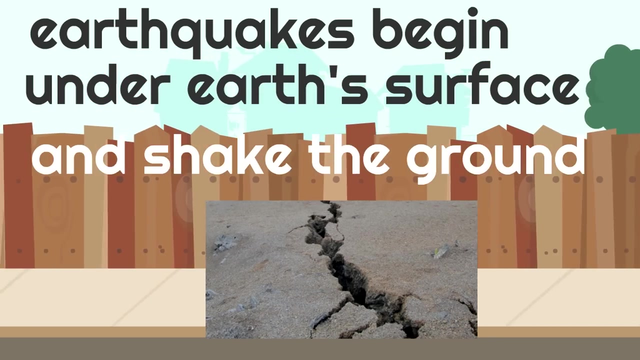 earthquakes begin under Earth's surface and shake the ground. here's a picture of something that can happen when there's an earthquake. do you see the massive cracks in the ground? this is from an earthquake. the earthquake began under the Earth's surface, it shook the ground and it caused this crack. oh my goodness, look at that. 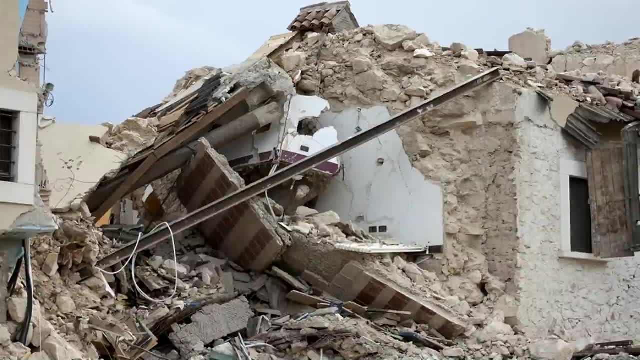 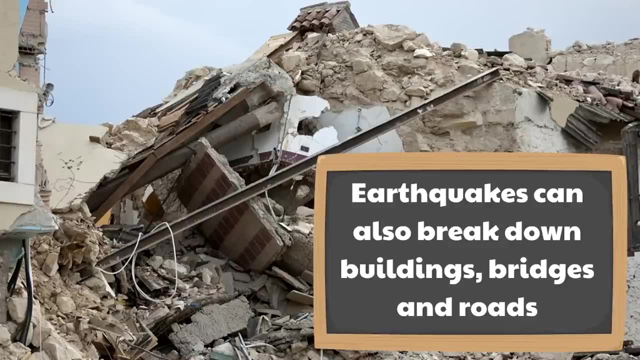 that Michelle's fist theruck shot, but this time we're good. I'm sure you can see that highMy goodness. look at this picture that shows damage from an earthquake. the earthquakes can also break down buildings, bridges and roads. they don't just caused cracks in the ground, they break all kinds of things. 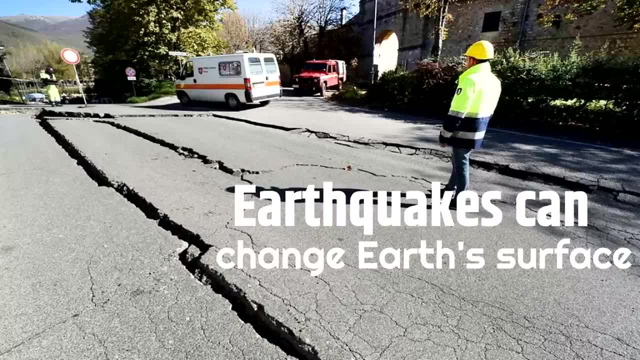 around us. earthquakes are so powerful they can change ordeals and roads. they don't just cause cracks in the ground, they break all kinds of things around us. earthquakes are so powerful they can change Earth's surface. well, Her digital now are seeingsu low Desert earthquake alarm signals are so powerful that people may wonder where these Shooter power staggering profiles of Earth's surface disease may be. things worried about Nichtew correctly, the projects to reduce the numbers so much further based on opportunities in the weather. 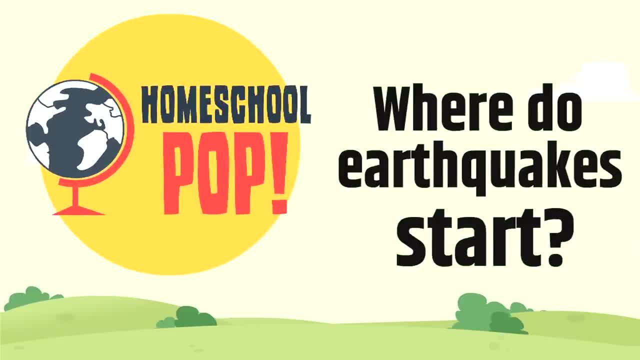 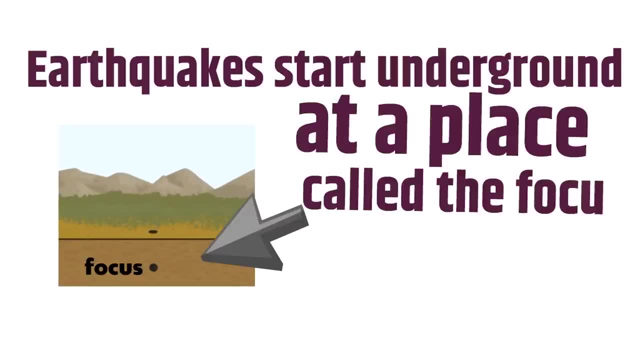 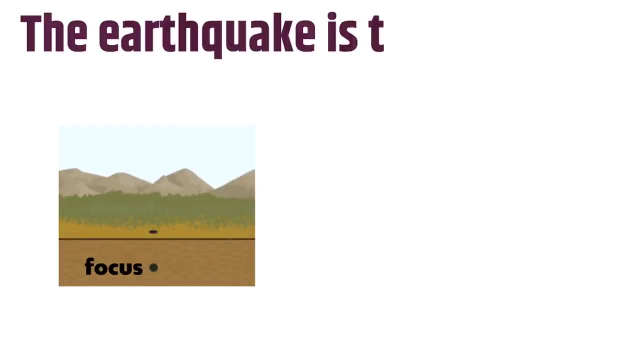 do earthquakes start? earthquakes start underground at a place called the focus. you could see it here on the picture. that's a weird name for it. I know it's called a focus, we don't know why, but that's just the way it is. it's called the focus where the earthquake starts. the earthquake is the strongest at the 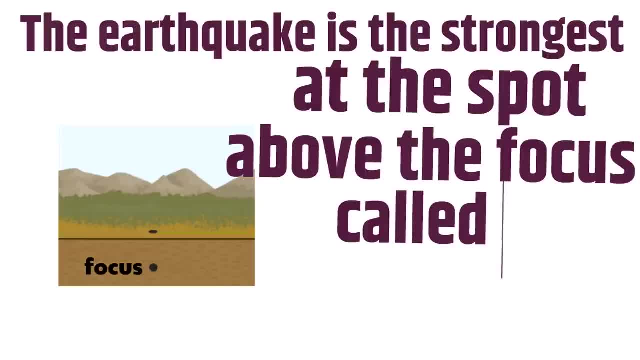 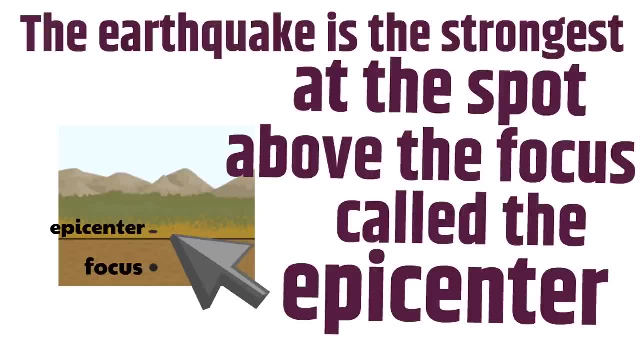 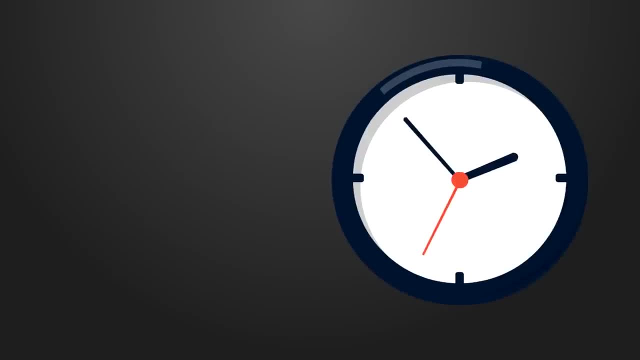 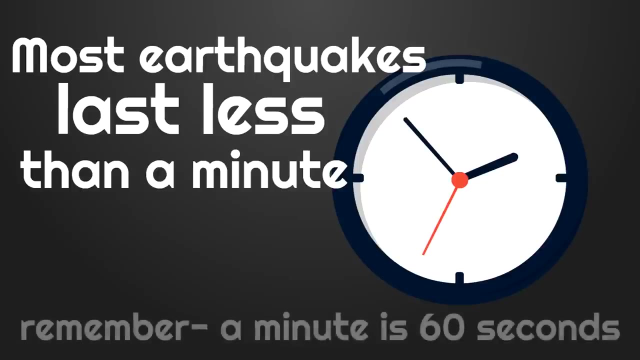 spot above the focus called the epicenter. you can see from the picture. it's directly above. when an earthquake happens, you don't want to be anywhere near the epicenter. while earthquakes are very powerful, they don't last that long. in fact, most earthquakes last less than a minute. remember: a minute is 60 seconds, it's not. 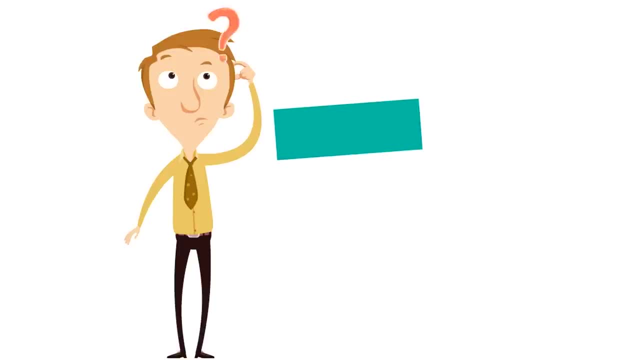 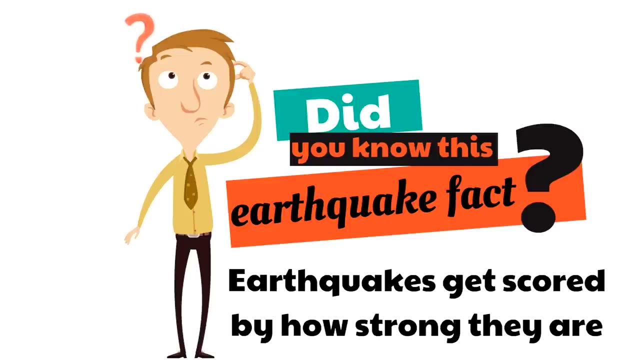 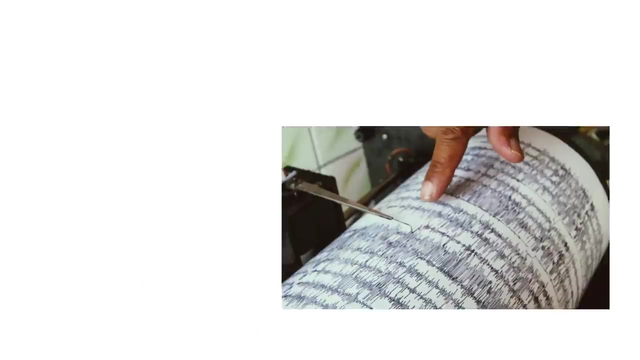 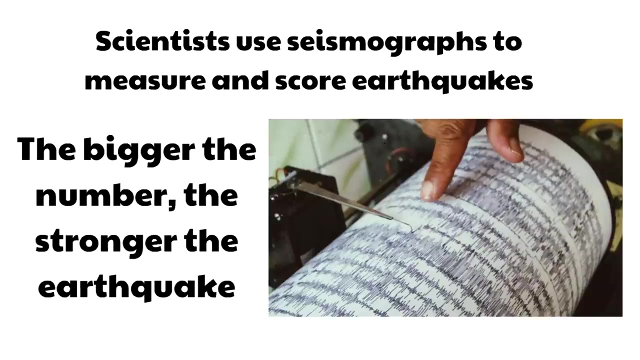 too long. and did you know this earthquake fact: earthquakes get scored by how strong they are. that's pretty neat. earthquakes get their own score, their own number. scientists use seismographs to measure and score earthquakes. the bigger the number, the stronger the earthquake. so here are some common earthquake scores. a: 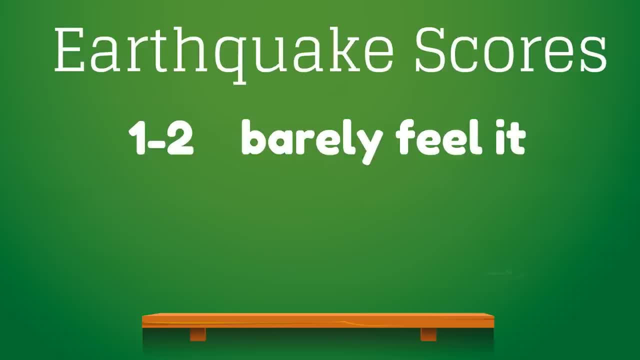 one or two earthquake, you barely feel it. the three to six range of earthquakes: they're going to be some damage. but 7 plus any number, that's seven or higher for an earthquake score, that's a massive earthquake and there's going to be tons of damage. 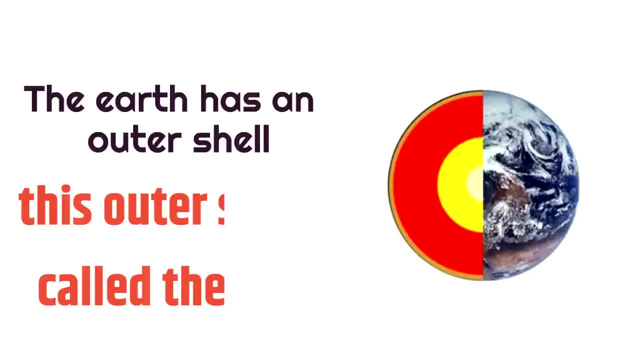 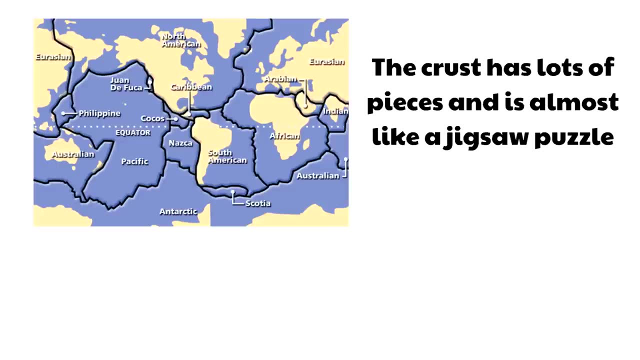 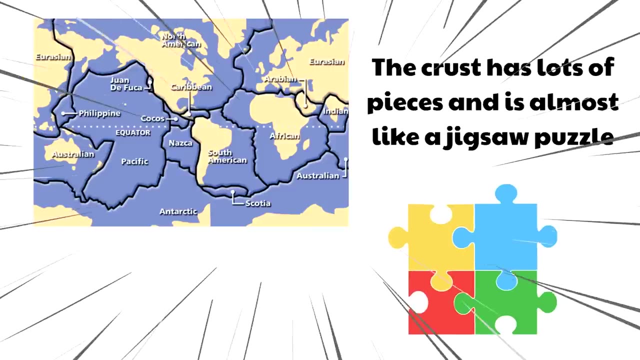 remember, the earth has an outer shell and this outer shell is called the crust. the crust has lots of pieces and it's almost like a jigsaw puzzle and all the pieces are always moving. but if they move too fast that can cause an earthquake in an earthquake. 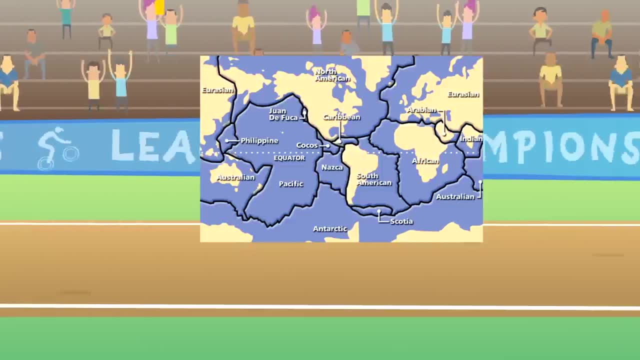 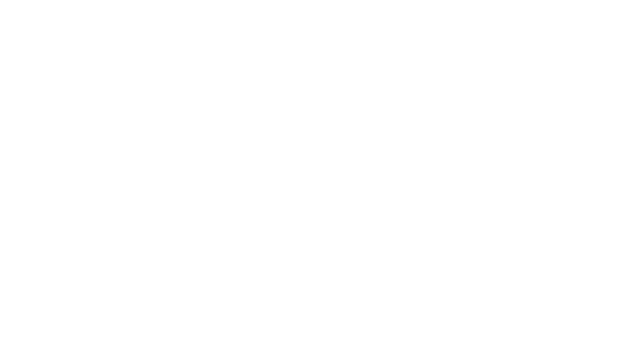 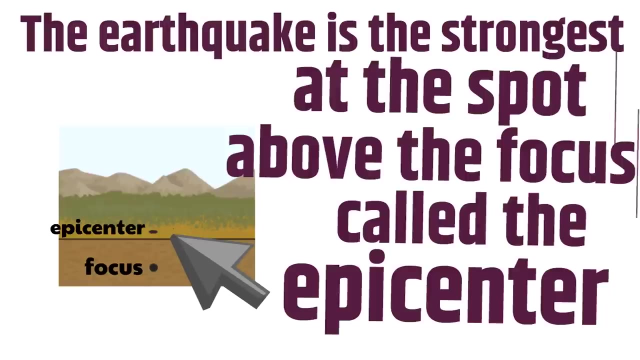 changes the earth's surface and can damage roads, bridges, buildings and even crack up the earth. and remember the earthquake is the strongest at the spot above the focus called the epicenter. you don't want to be anywhere near the epicenter if an earthquake was to happen. 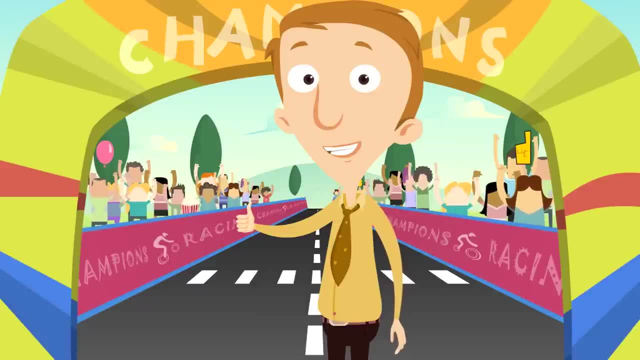 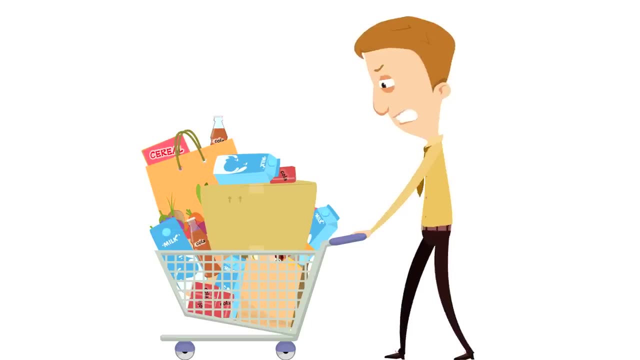 thanks for learning about earthquakes with us, a powerful way that earth's surface changes. oh, this is such a heavy cart. oh, my goodness. oh, it's hard work. you know, a lot of times learning can be hard work too, but we hope that these videos are really helpful, make learning fun, so that learning is hard like pushing this cart. 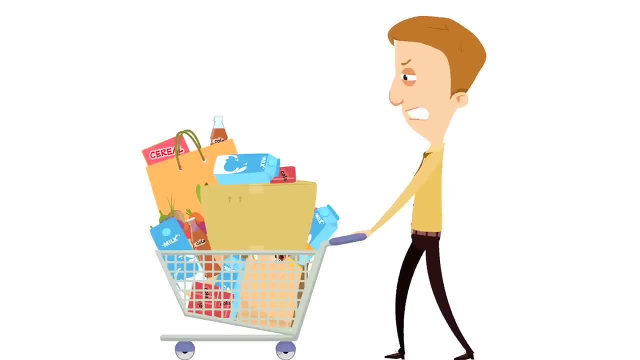 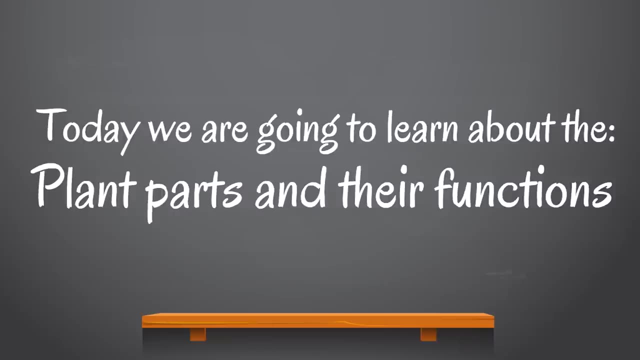 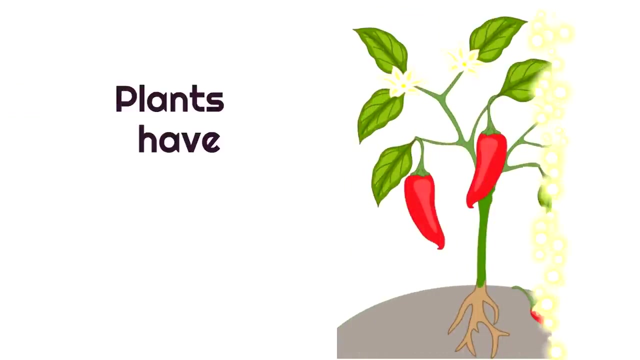 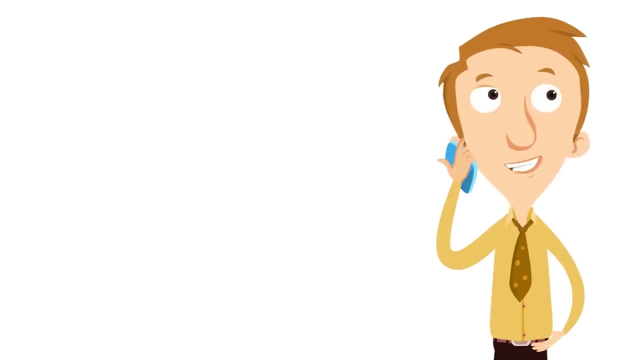 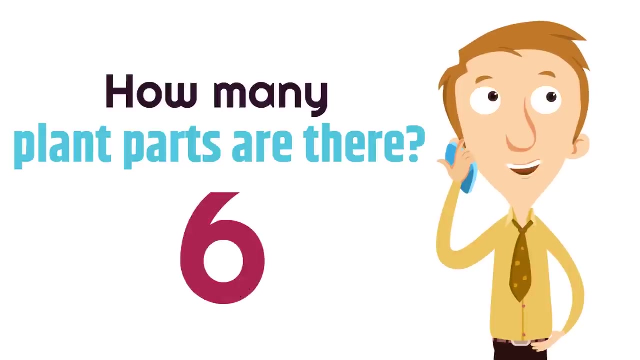 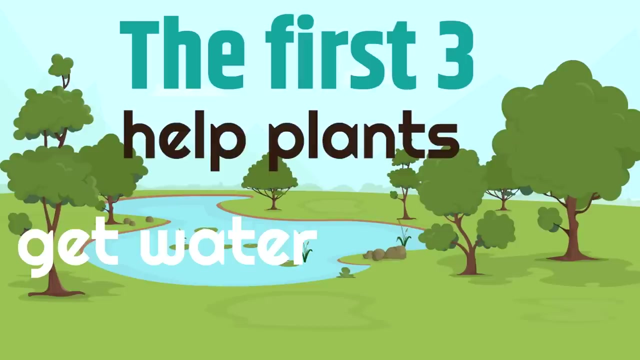 oh, my goodness, all right, what's the next thing we should learn about? let's learn about the plant parts and their functions. okay, so plants have six parts. alright, so how many plants parts are there? yeah, six, there are six parts. plant parts: The first three help plants get water, make food and grow. 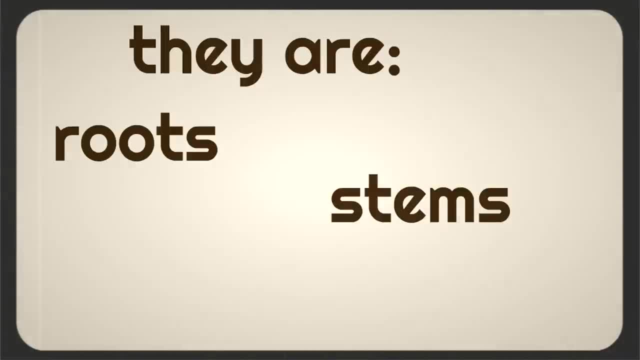 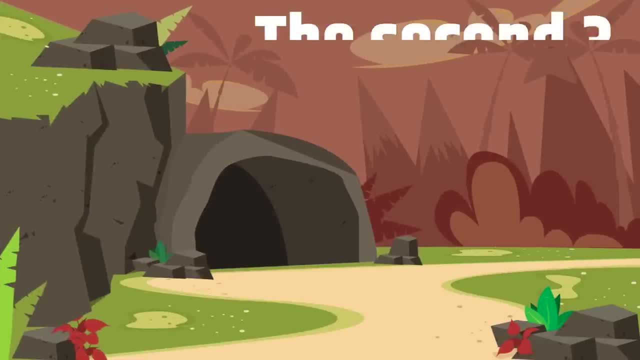 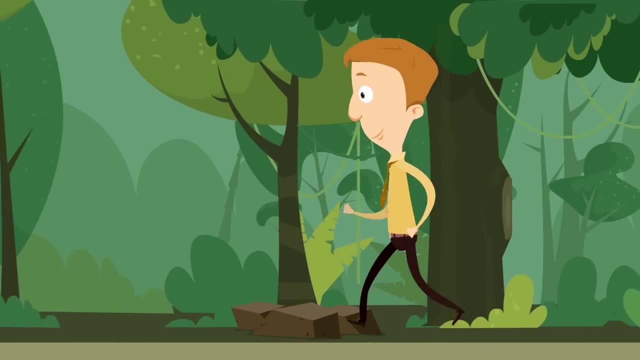 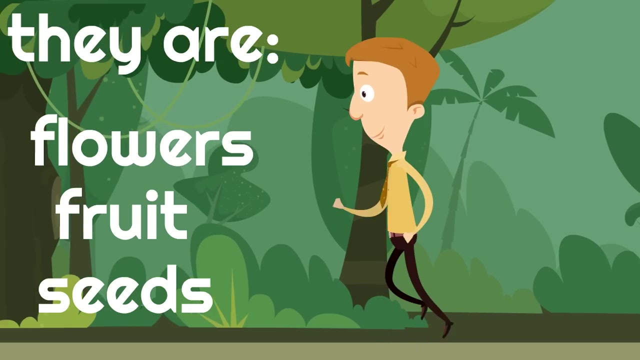 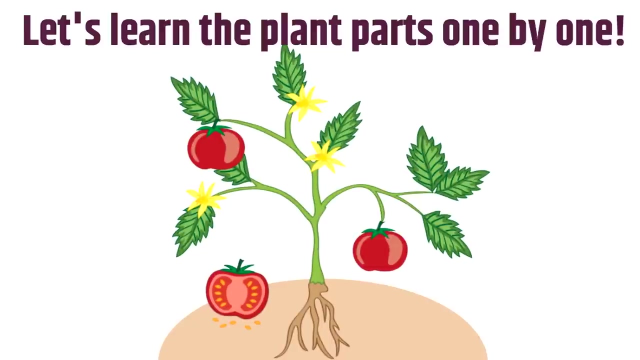 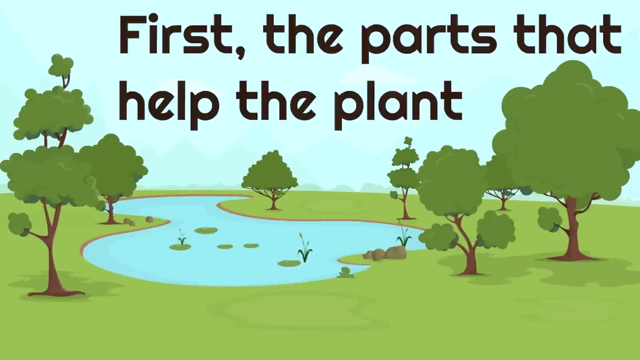 They are roots, stems and leaves. The second three help plants grow new plants. They are flowers, fruit and seeds. So let's learn the plant parts one by one. First, the parts that help the plant get water, Make food and grow. 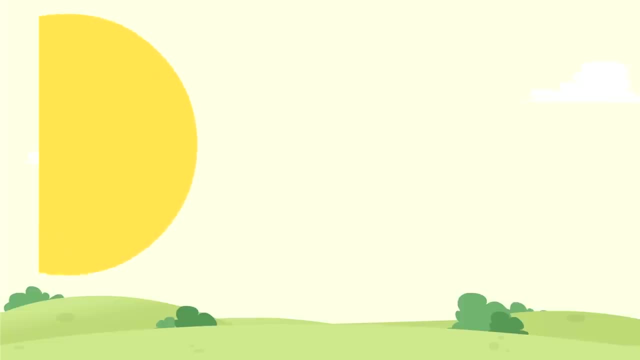 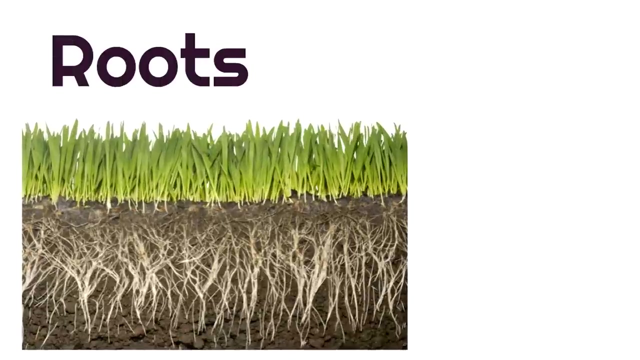 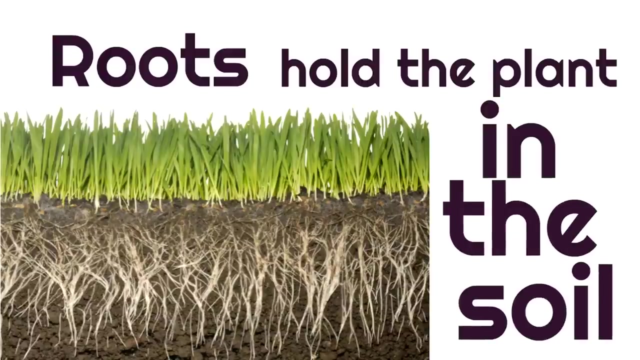 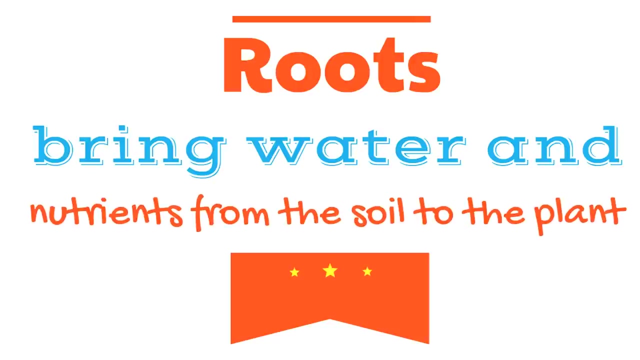 Okay, so the first plant part we're going to look at today are the roots. Roots have a special job. You see. roots hold the plant in the soil. The soil is the dirt in the ground, Then roots bring water and nutrients from the soil to the plants. 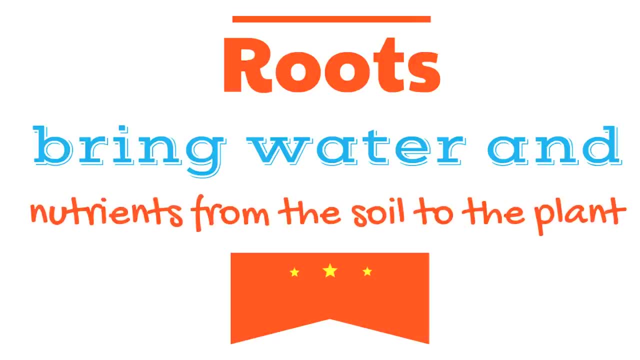 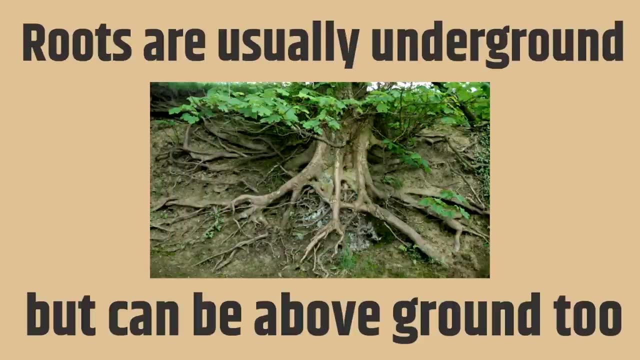 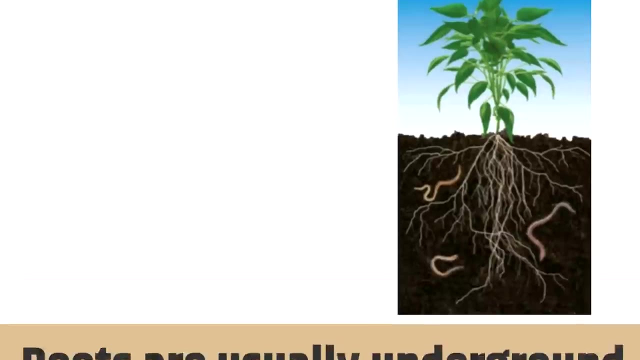 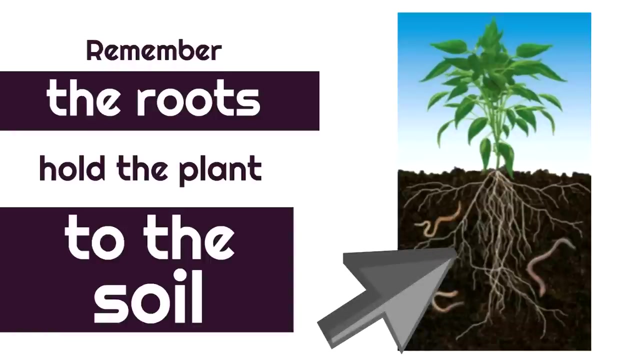 The roots are usually underground, but can be above ground too. Have you ever seen a tree that looks like this, where the roots are above ground? Remember, the roots hold the plant to the soil. Okay, so now we're going to look at the second part of a plant. 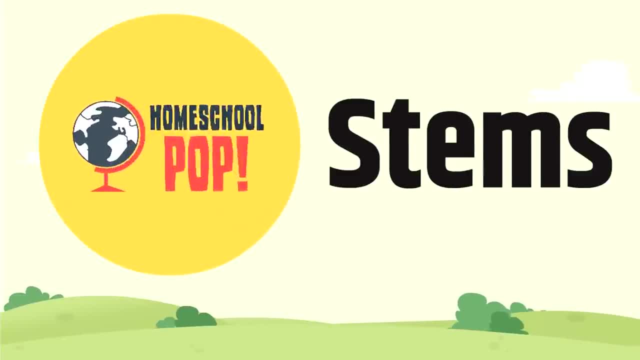 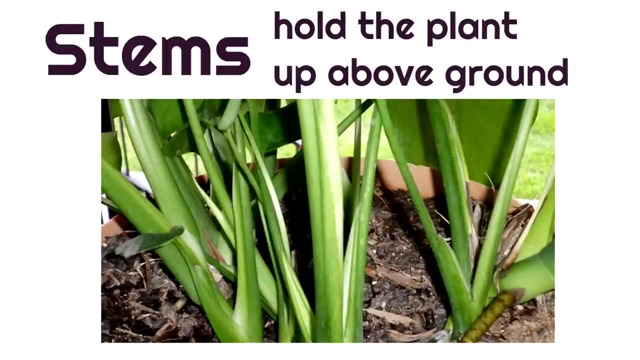 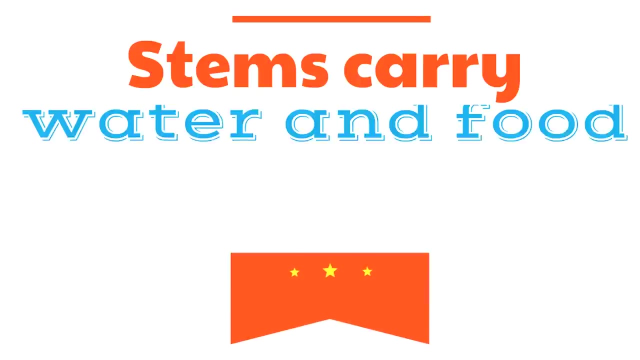 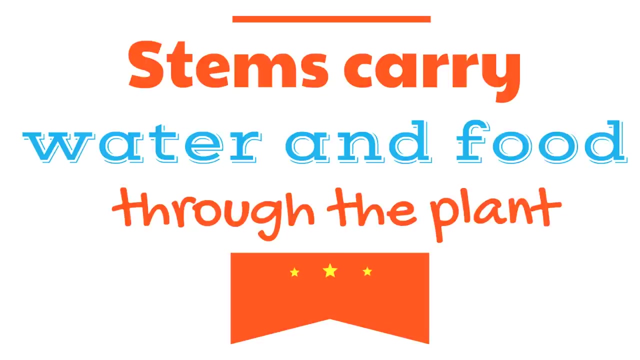 The roots hold the plant in the soil. The roots hold the plant in the soil, Which are the stems. Now, the stems hold the plant up above ground. The stems carry water and food through the plant. Stems are the delivery system of the plant. 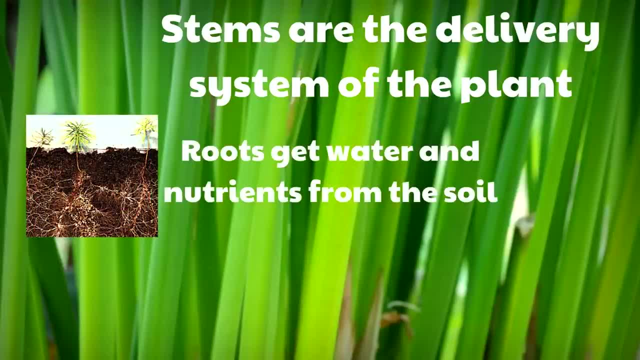 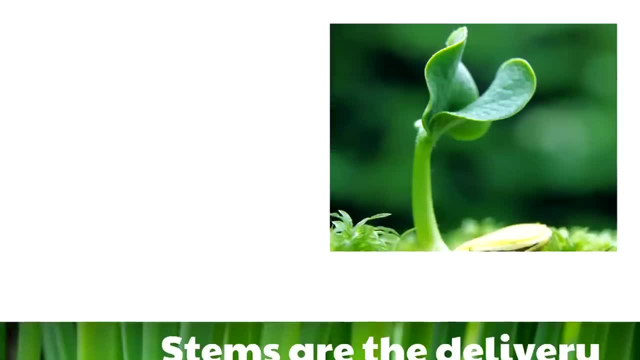 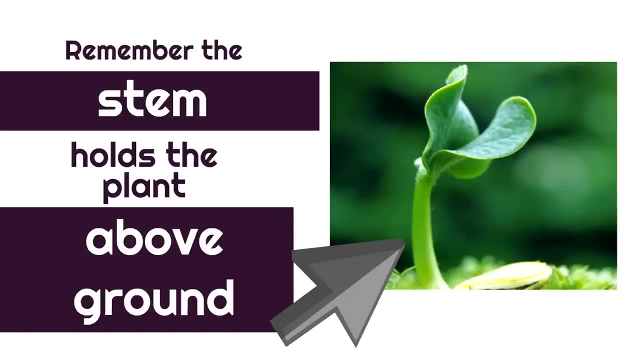 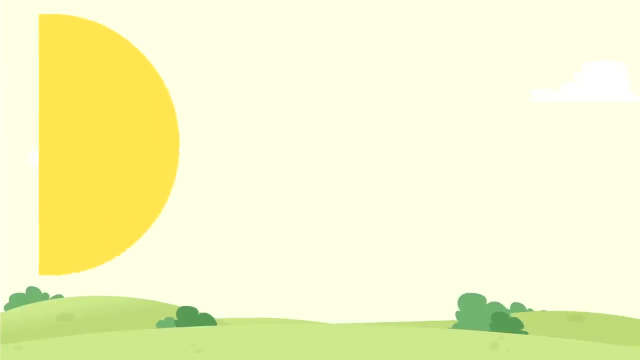 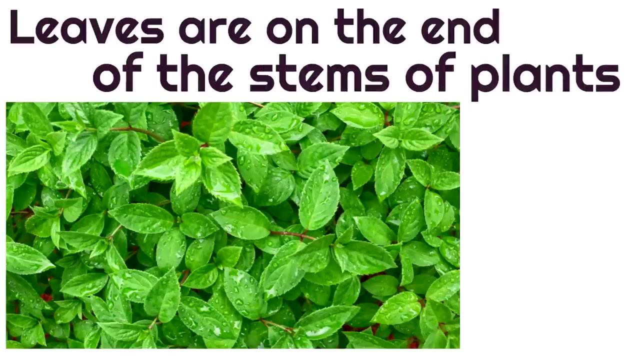 Roots get water and nutrients from the soil and the stems carry the water and nutrients throughout the plant. Remember, the stem holds the plant above ground. The next part of the plant we're going to learn today are leaves. The leaves are on the end of the stems of plants. 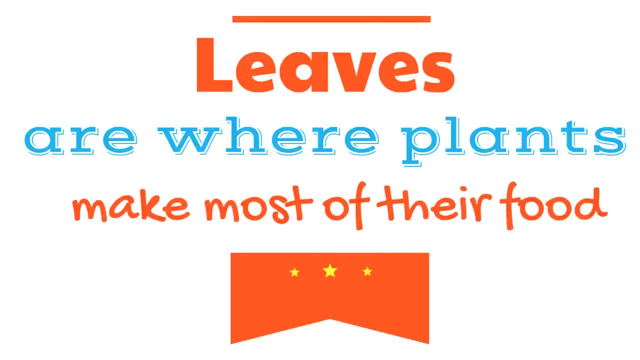 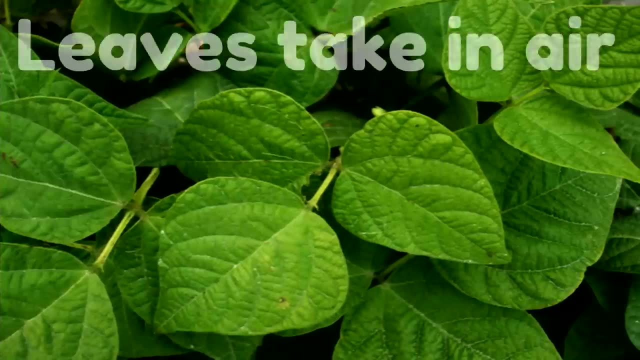 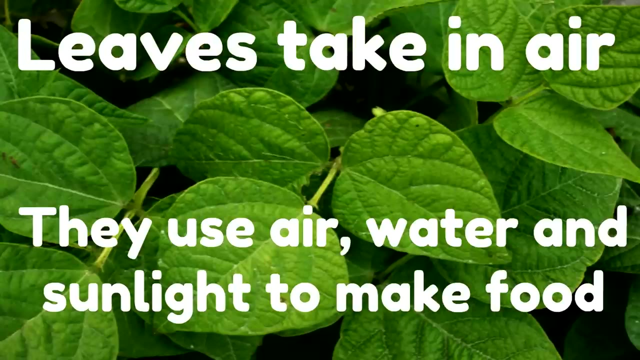 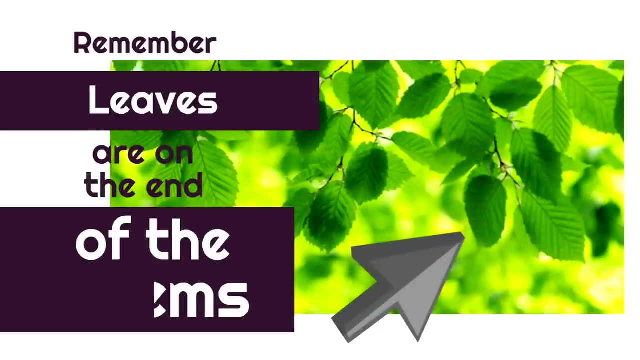 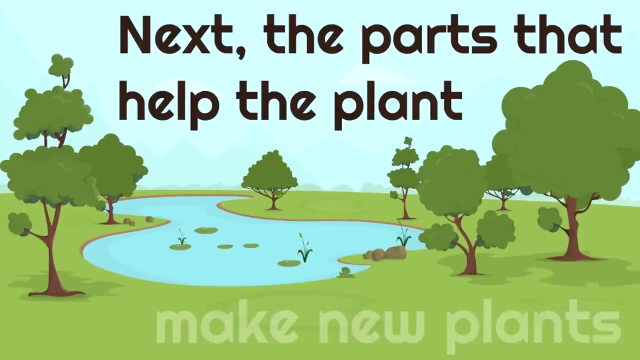 And this is interesting- leaves are where plants make most of their food. Leaves take in air and they use air, water and sunlight to make food. Remember, leaves are on the end of the stems. Okay, so next, the parts that help the plant make new plants. 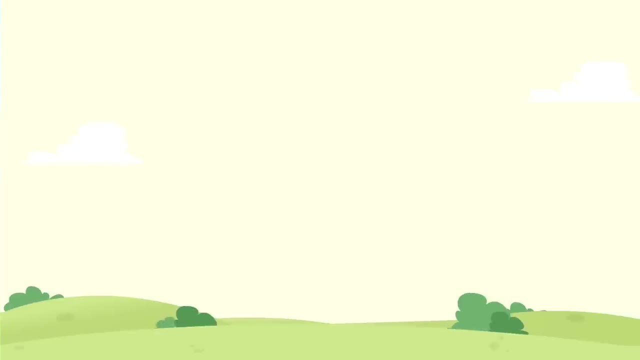 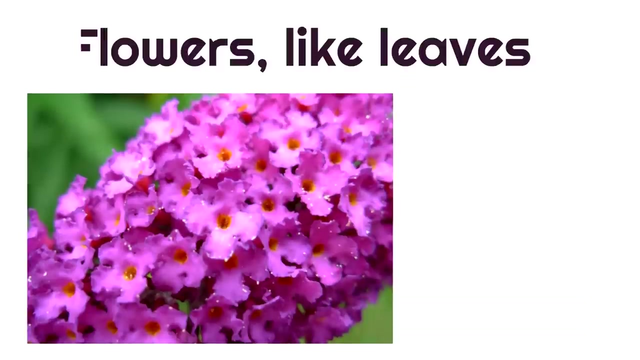 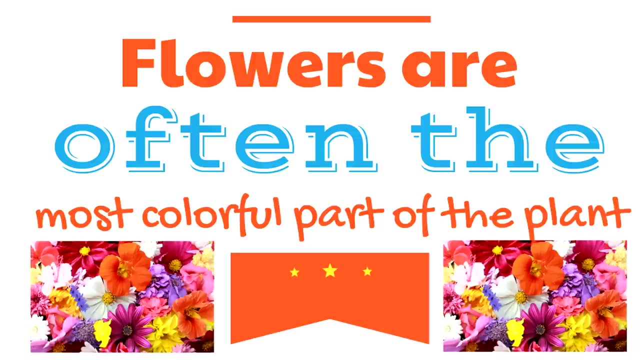 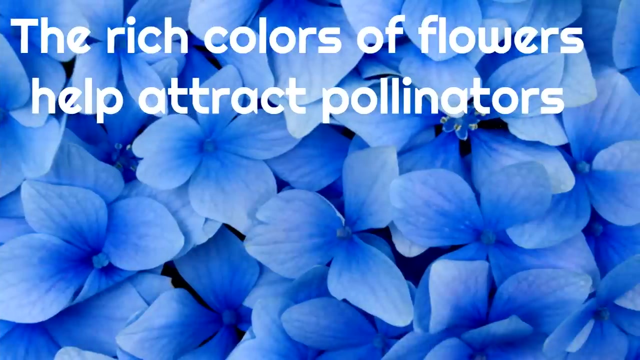 The next part we're going to look at are flowers. Flowers, like leaves, grow on the end of the stems. Flowers are often the most colorful part of the plant. Okay, now, this is awesome. The rich colors of flowers help attract pollinators. 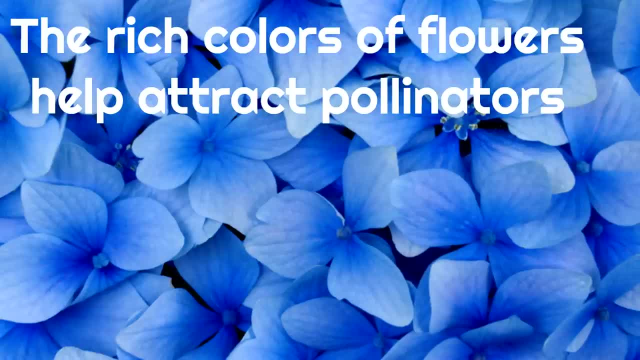 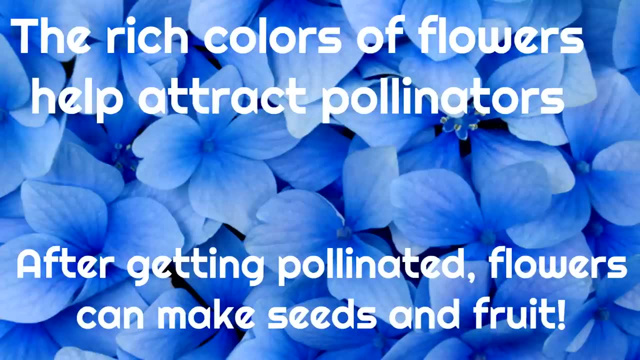 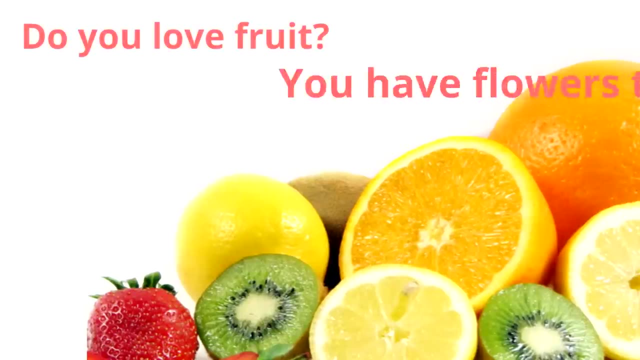 That's why they're beautiful. The beauty has a purpose. After getting pollinated, flowers can make seeds and fruit. Do you love fruit? Yes, fruit is awesome. You have flowers to thank for that. Flowers make fruit, so the next time you're eating an amazing piece of fruit. 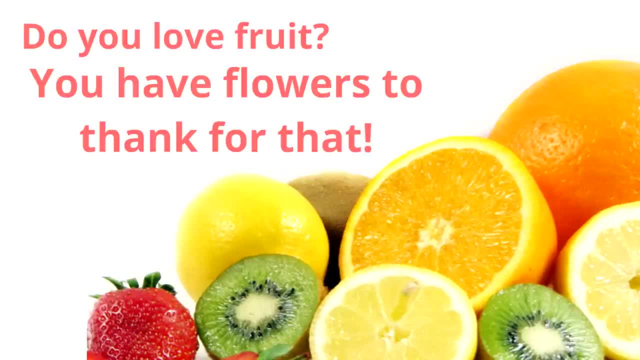 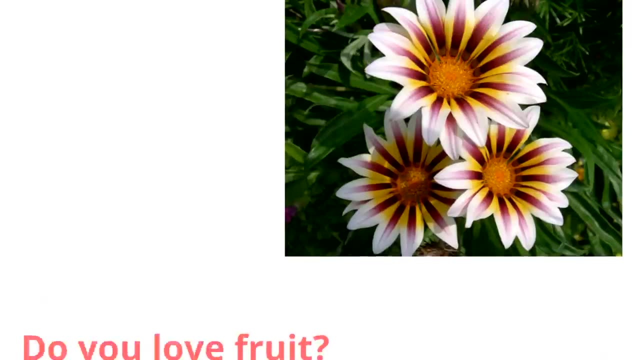 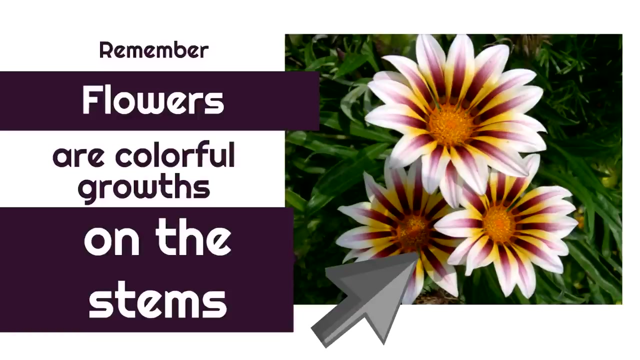 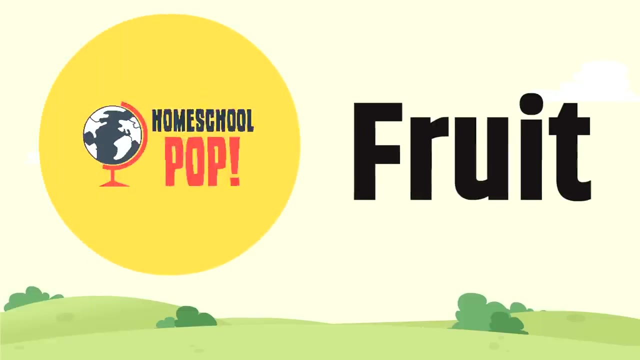 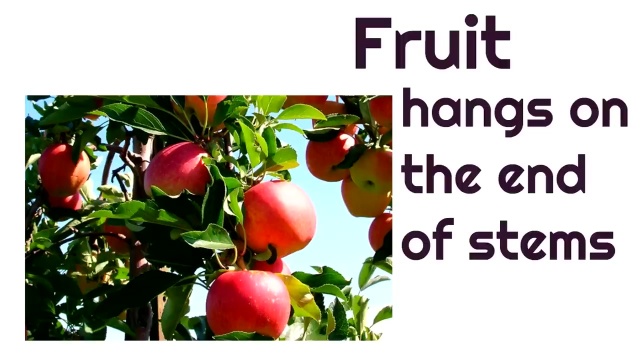 just think to yourself. thank you flowers, Thank you flowers, Thank you flowers. Remember, flowers are the colorful growths on trees, the stems. the next part of the plant we're going to learn about is the fruit. all right now, where on the plant is the fruit? fruit hangs on the end of stems. 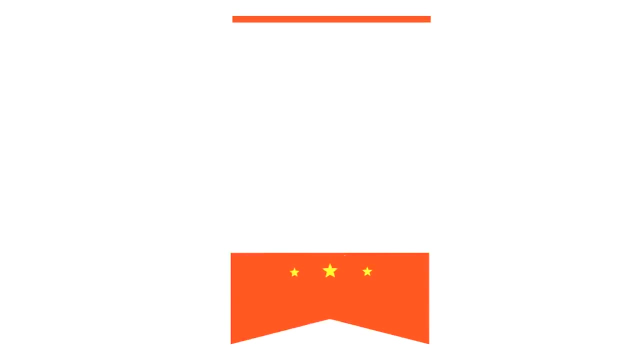 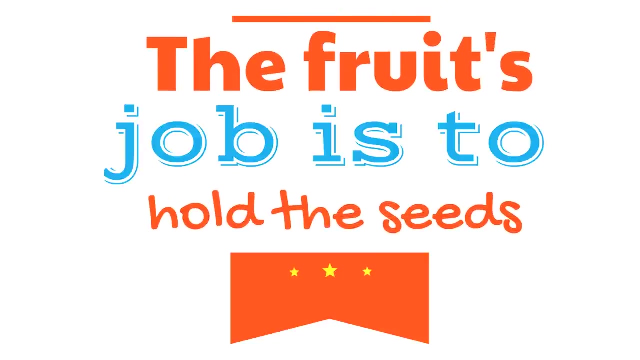 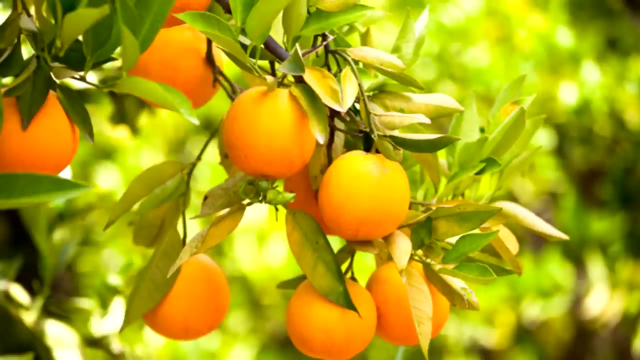 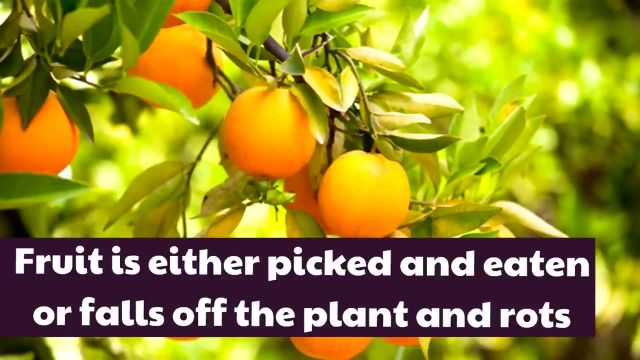 now you might be wondering: what's the fruit's job? what does the fruit do? well, the fruit's job is to hold the seeds. the fruit is just a delicious seed holder. now, either one of two things happens to fruit: fruit is either picked and eaten, or it falls off the plant and rots. 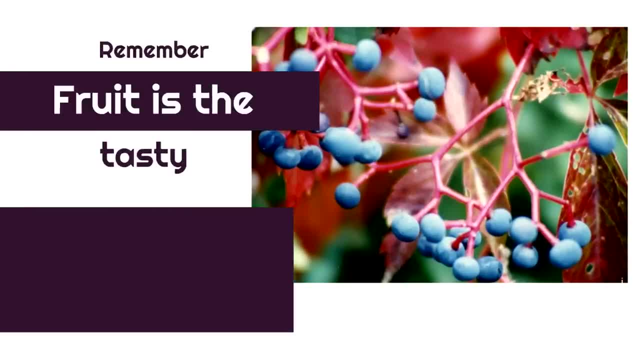 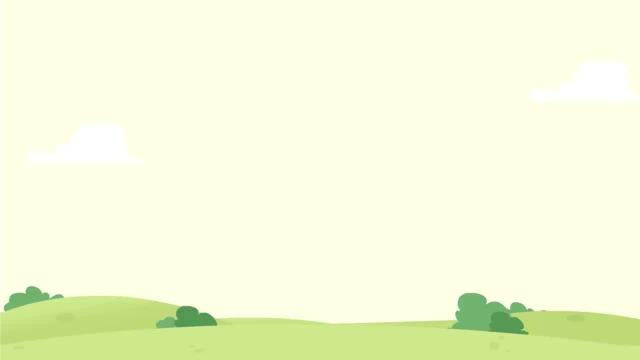 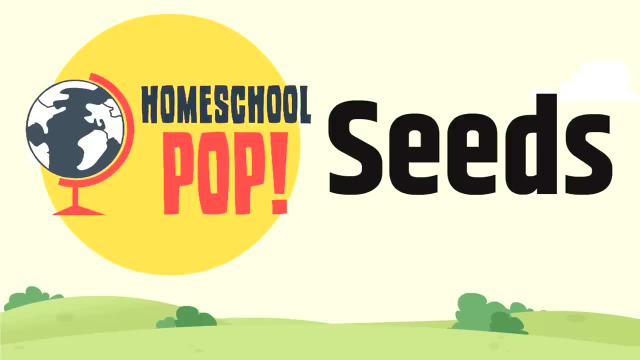 remember fruit is the tasty stuff on the stems. it will bear fruit come to mind. fruit is just a delicious thing to eat. okay, the last part of the plant that we're going to learn today are the seeds- seed. so where are the seeds of the plant? seeds hide inside of the fruit. 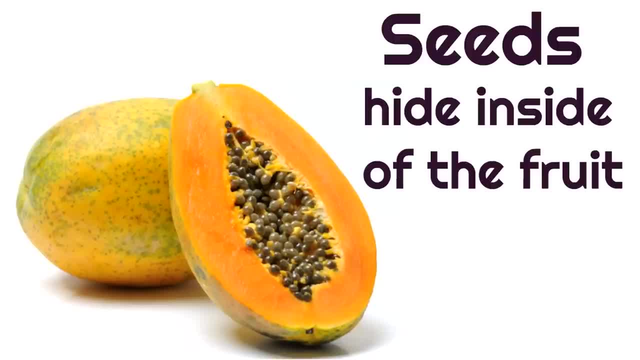 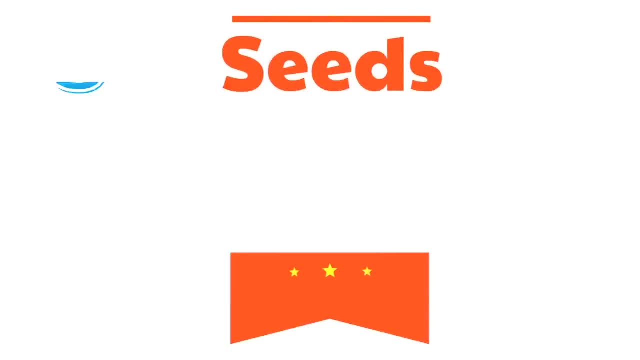 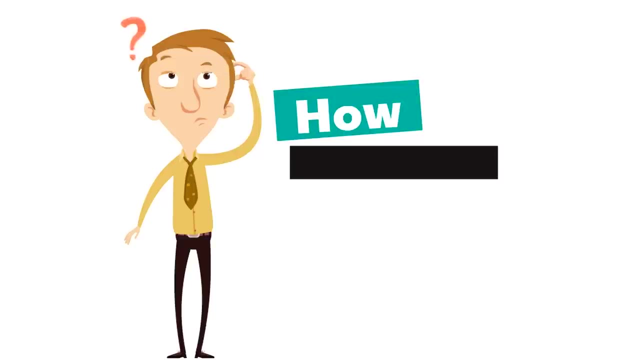 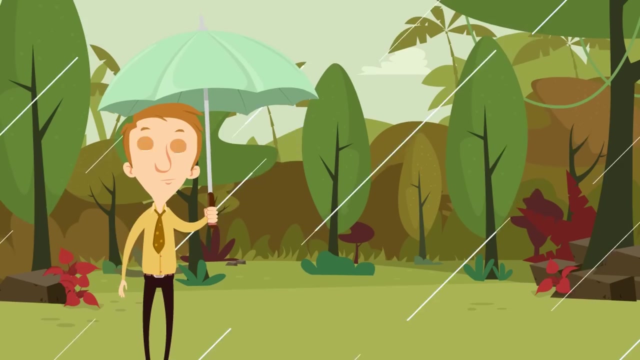 seed, seeds, seed, seed, seed. now the seeds have an incredible job. you see, seeds grow into new plants. seeds grow into new plants. seeds grow into new plants. Okay, you might be wondering: well, how does that work? Well, here's one way. When animals eat fruit, they eat the seeds. 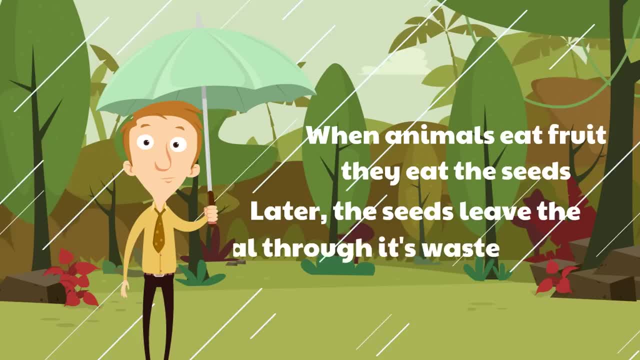 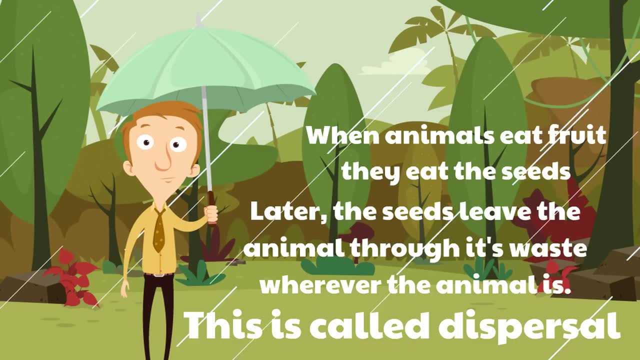 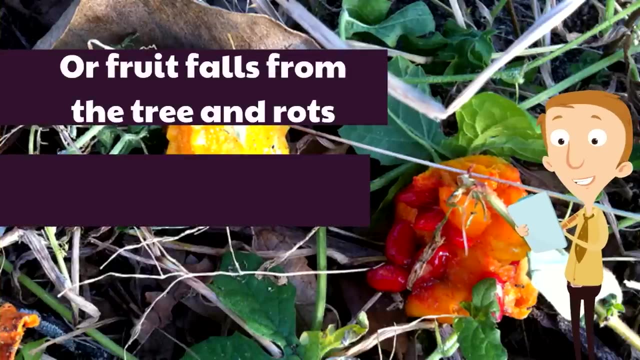 Later the seeds leave the animal through its waste, wherever the animal is. This is called dispersal, Or fruit falls from the tree and rots. The word rots means dies. the fruit dies, it rots. The seeds fall out and can make a new plant. 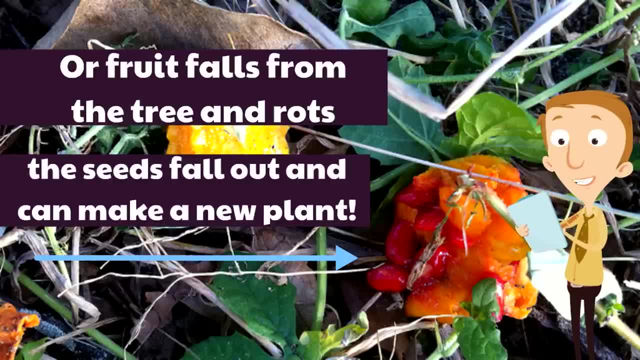 The first way, called dispersal, takes the seed to another place, so it plants a new plant in a new place. When a fruit falls and rots, it plants a new plant nearby the original plant. Remember, seeds live inside Of the fruit. Hey, it looked like you were doing a good job, paying attention, learning about the 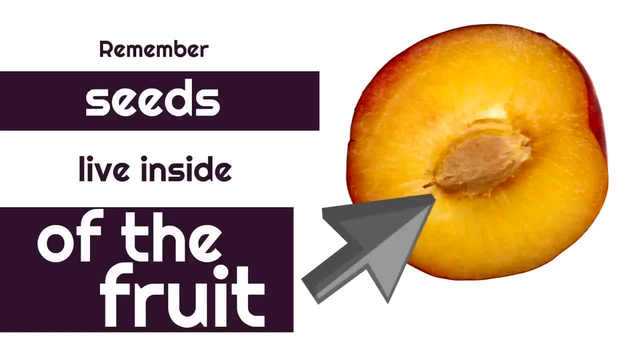 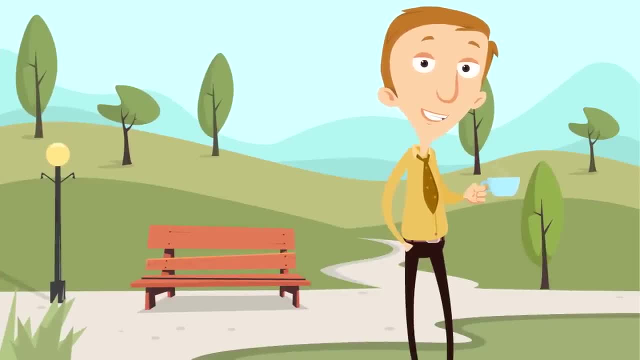 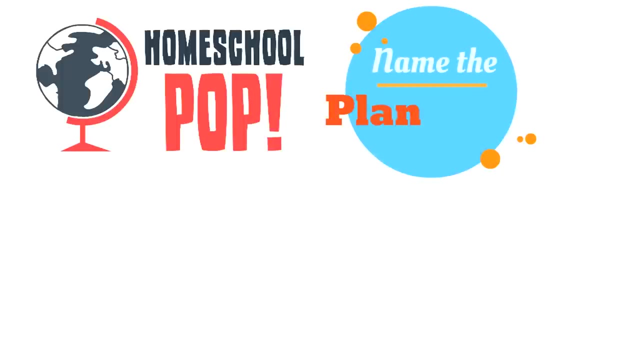 plant parts. And now we want to see how much you learned. We're going to play a game called name the plant part. We're going to show you a plant part And then you go ahead And tell us which plant part it is. 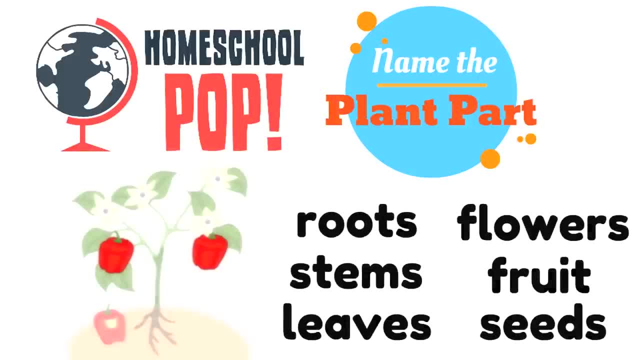 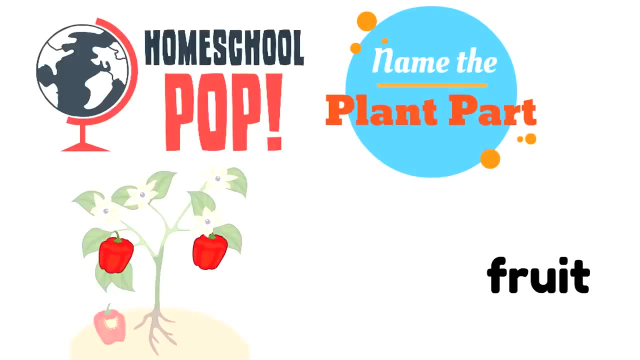 All right, hope you're ready, because here we go. Look at this picture of a plant. Which plant part is colored in? Uh huh, the fruit. The fruit of this plant. Great job, Here's the next one. What plant part is colored in? 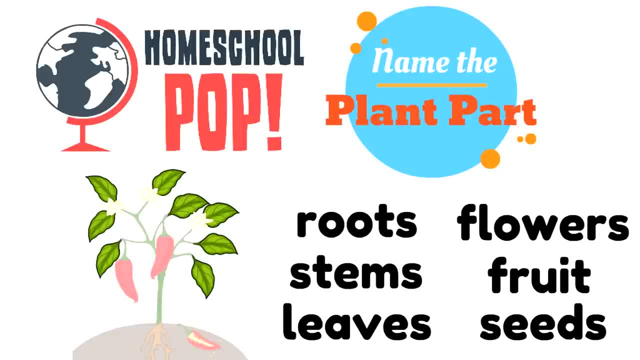 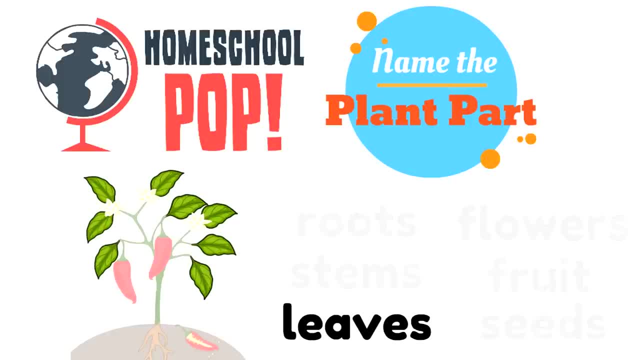 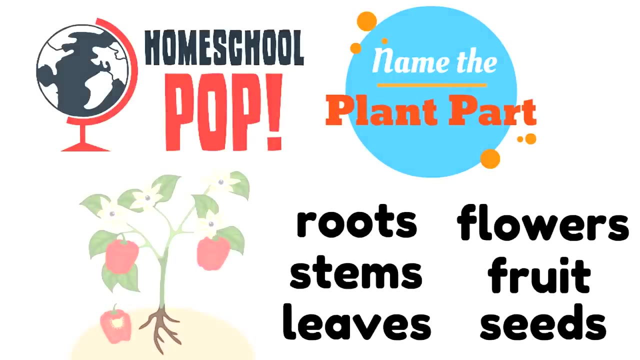 Yeah, the leaves. The leaves are colored in. Great job, All right, it's time for this one. It's colored brown. Which plant part is this? Uh huh, the roots. Awesome. Okay, let's try this one. 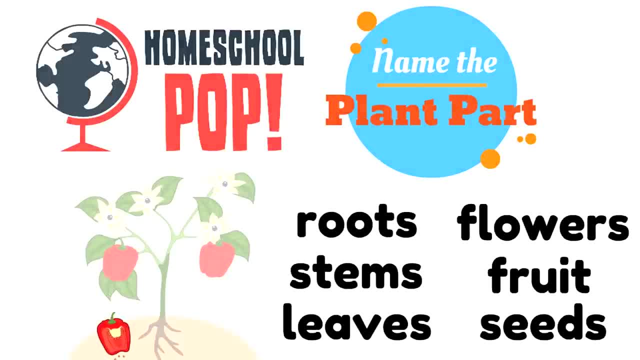 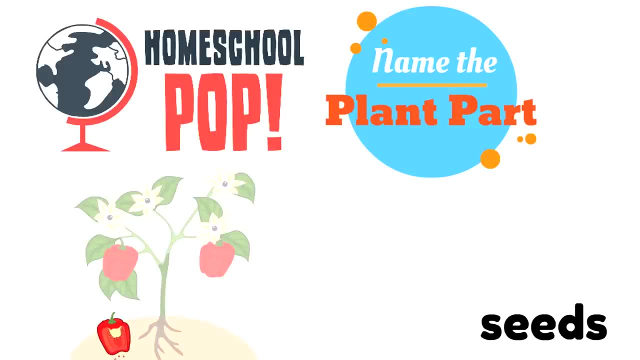 What part of the plant is colored in? Do you see it there on the bottom? What is that? Yeah, what part is that? Yes, the seeds. Let's try this one. Look at the picture. Could you name the plant part? 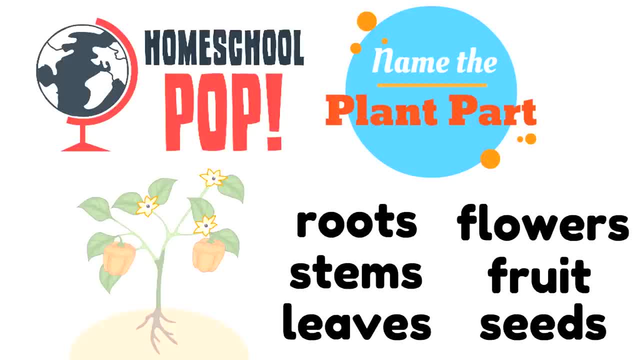 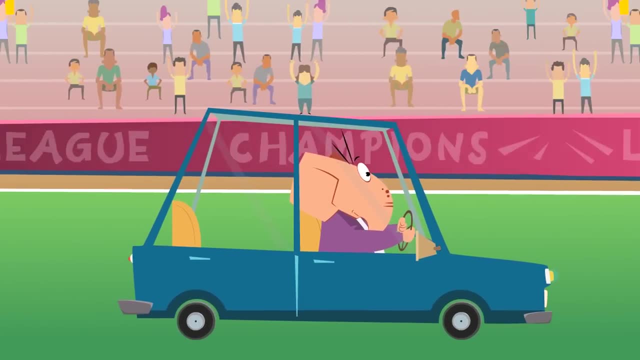 Which plant part is that? You can see it's outlined in green. You can see it's outlined in color. Yeah, the flowers, Awesome job. Hey, well, okay, first of all, elephants don't drive. Okay, elephants can't get a driver's license. and he's driving on the grass. 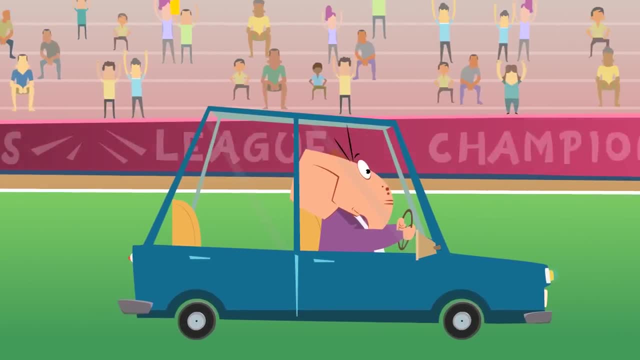 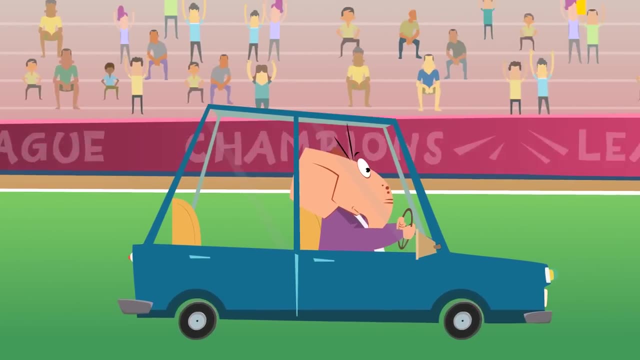 He's driving on the grass. You're going to ruin the lawn. Okay, what's going on here? All right, this is out of hand. Okay, elephant, I don't want to tell you what you can do and what you can't do, but you can't drive. 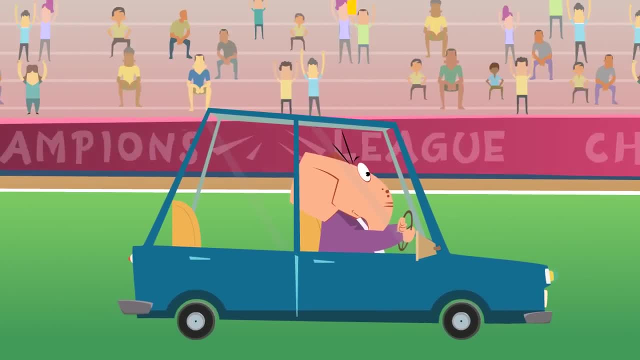 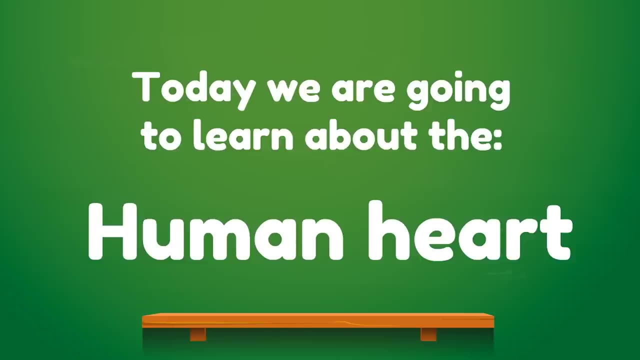 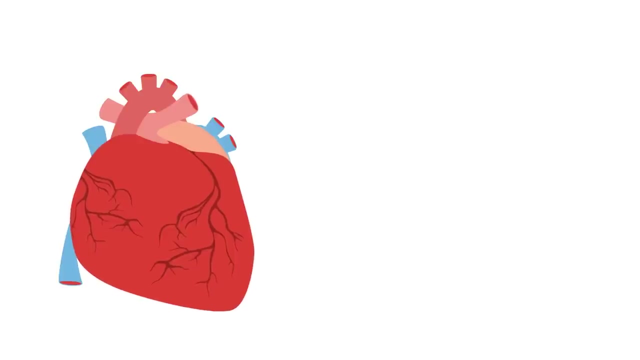 All right, Oh my goodness, All right. next we are going to learn about the human heart, the different parts of your heart, how it works, how it functions. We're going to have such a great time, Okay, well, let's start here. 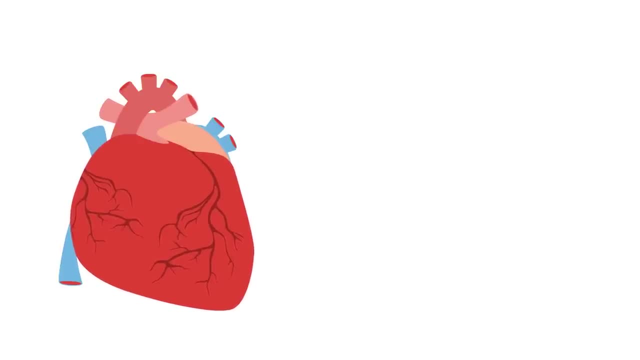 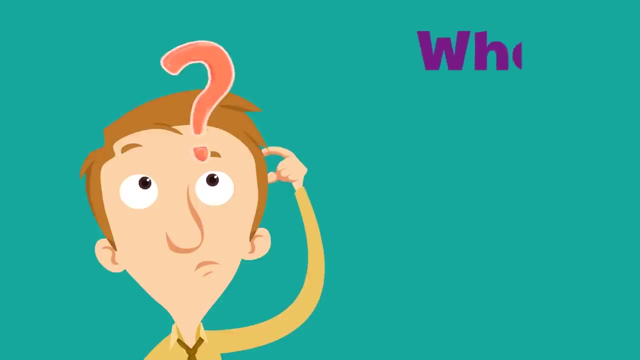 What is the heart? That's a great question. What is the heart? What is the heart? Well, the heart is an organ of your body. Yeah, that's right, The heart is an organ of your body. Okay, so what is an organ? 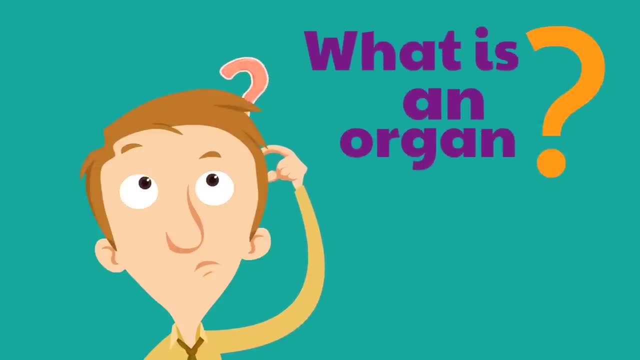 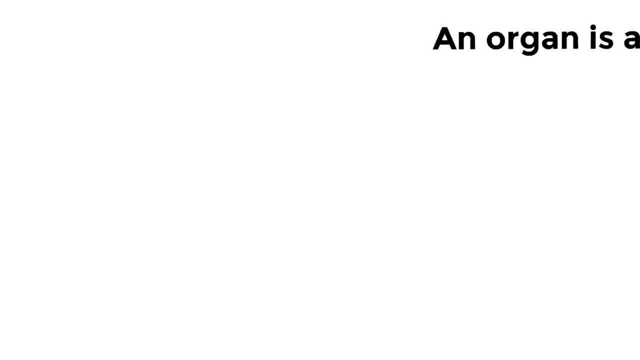 Yeah, we have to know that, to know what a heart is. If the heart is an organ of the body, what is an organ? It's interesting. An organ is a special group of tissues that do specific jobs for your body. How about your brain? 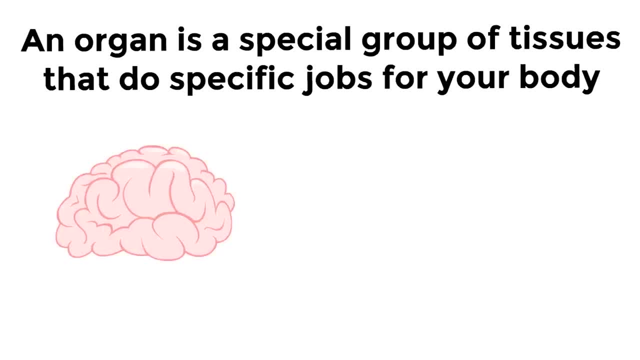 There's a special group of tissue inside your body, Like your brain. Your brain is an organ. It's a special group of tissues that does a specific job for your body. An eyeball, as an organ too, It's a special group of tissues that does a specific job for your body. 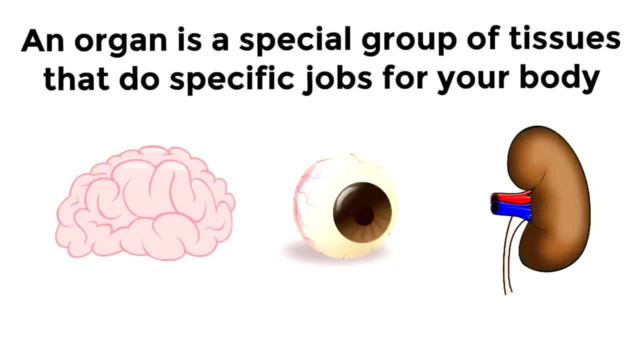 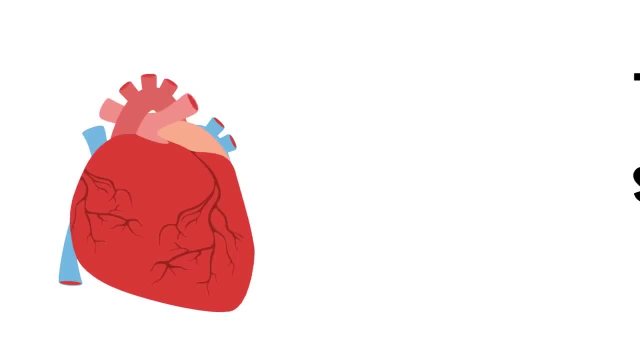 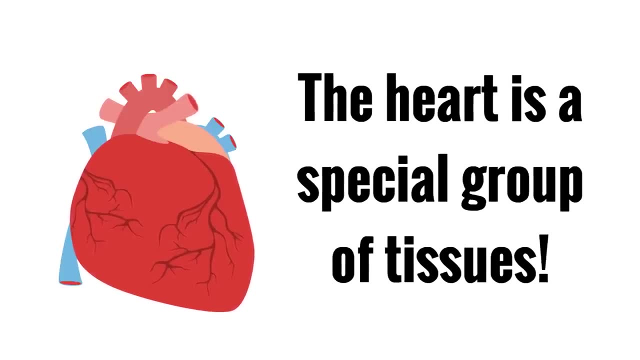 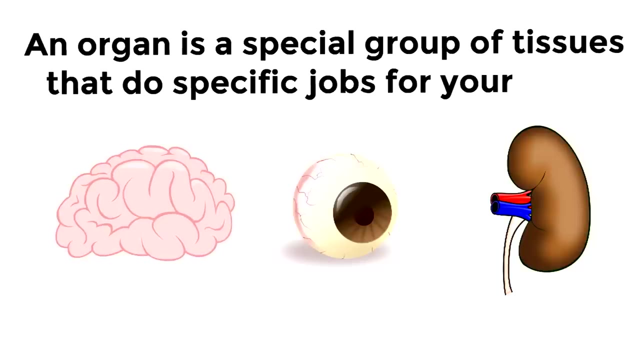 And how about a kidney? A kidney is an organ, a specific job for your body. so we know the heart is a special group of tissues, don't we? because it's an organ and an organ is a special group of tissues. but that's not all, remember. an organ is a special group of tissues that do. 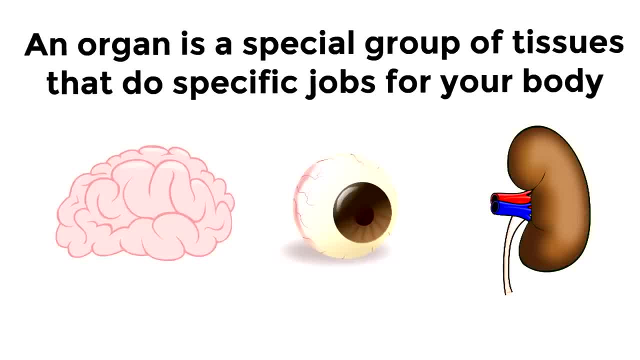 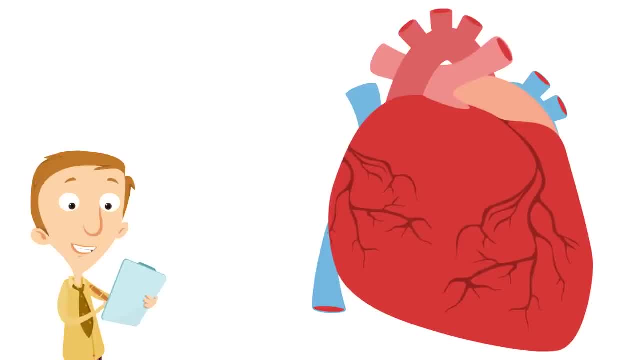 specific jobs for your body. they do different jobs, they have tasks to do. so what does the heart do? well, we could see it's moving, isn't it? the heart is constantly moving, Wow. so what does the heart do for your body? that's a really good question. why am I asking you that question? why am I not just telling you: 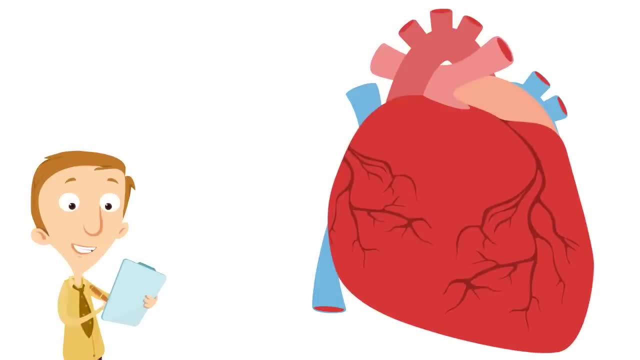 the answer. all right, let's tell you. well, here it is: the heart pumps blood through the body. that amazing. the heart pumps blood through the body. your heart is a big pump and it's pumping blood through your body. as you're watching this video right now, you're watching homeschool pop. you're having a great time and even 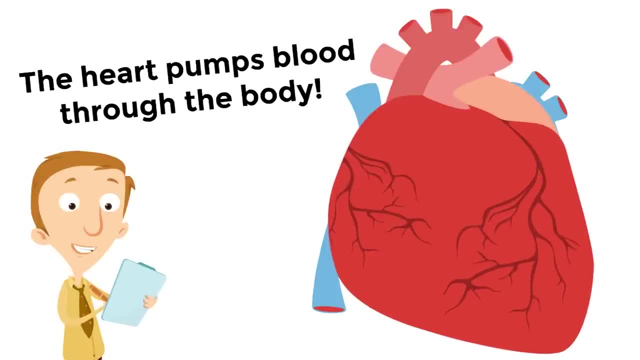 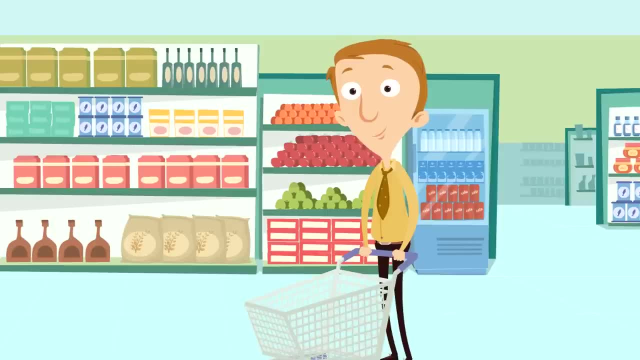 right now, your heart is pumping blood through your body. body, Isn't that incredible. So how does your heart do that? And why am I in a grocery store? I guess I'm hungry for fish again. So the heart has four chambers. Four chambers, If anyone ever asks you. 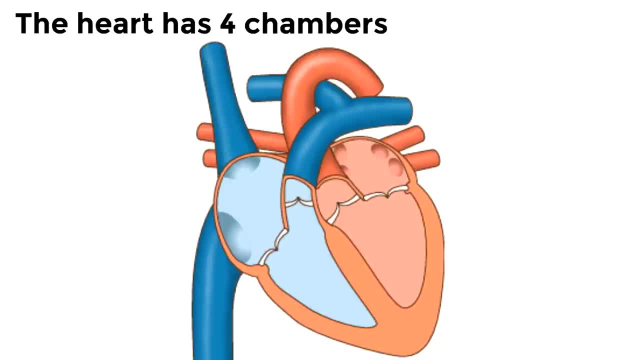 how many chambers does your heart have? You'll say my heart has four chambers. That word chamber almost means like a room. It's almost like your heart has four rooms. It has four chambers. There's the right atrium and there's the left atrium. These are the top chambers of your heart. 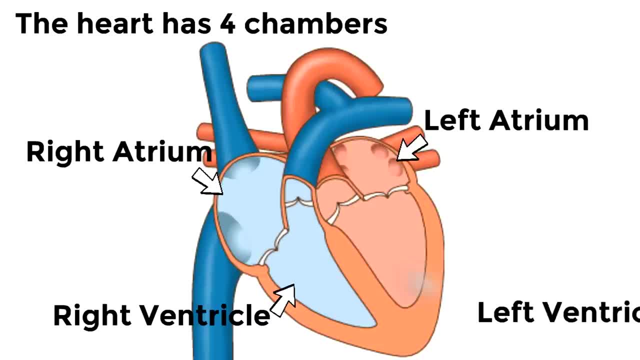 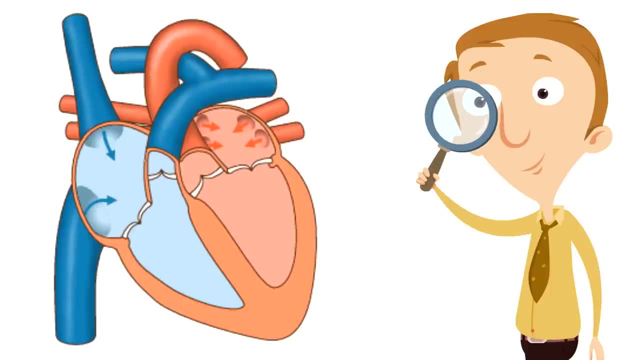 Then the lower two chambers are the right ventricle and the left ventricle. Pretty simple, The heart has four chambers: Two: Two on the top, Two on the bottom. So here is how the heart pumps blood through the body. The blood comes in through these valves. 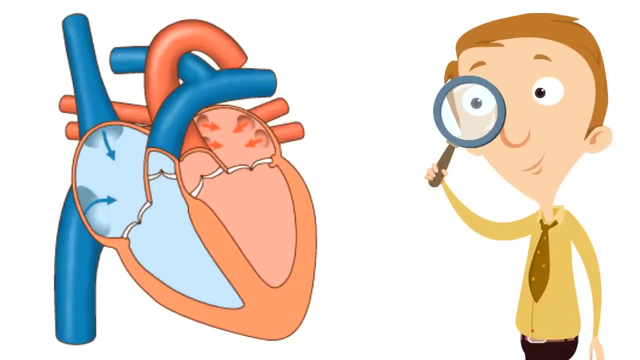 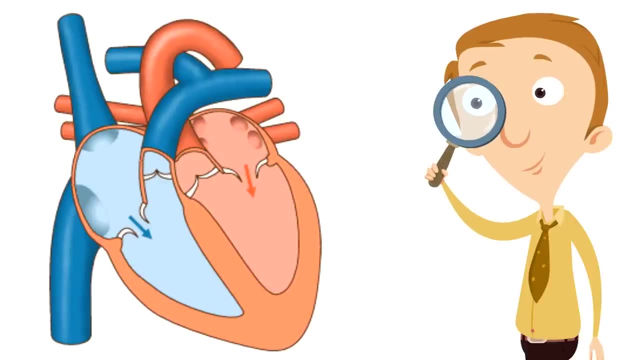 right here into the right atrium and the left atrium. Do you see those arrows? The blood flows in. Then the blood goes into the ventricles: The right ventricle and the left ventricle. Isn't that pretty cool? 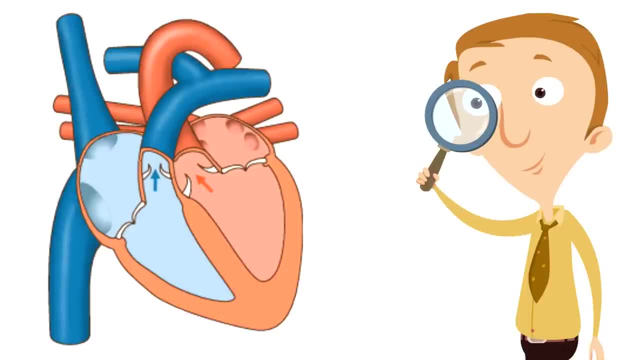 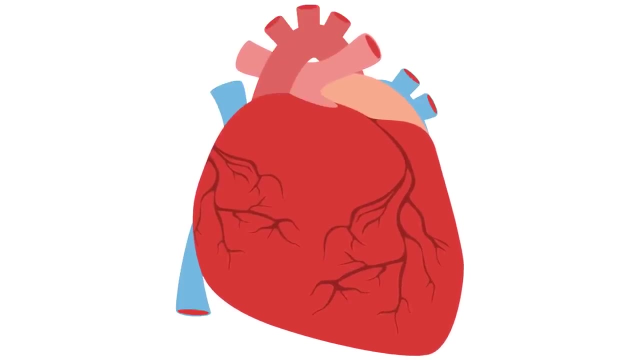 Then the blood leaves the ventricles through these valves up here and it's ready to replenish the body with the oxygen and nutrients that your body needs. This is all made possible because the heart is a muscular organ, meaning it has lots of muscles. Those muscles are what enables it to pump blood through your body. Isn't that cool? It's such a strong organ. 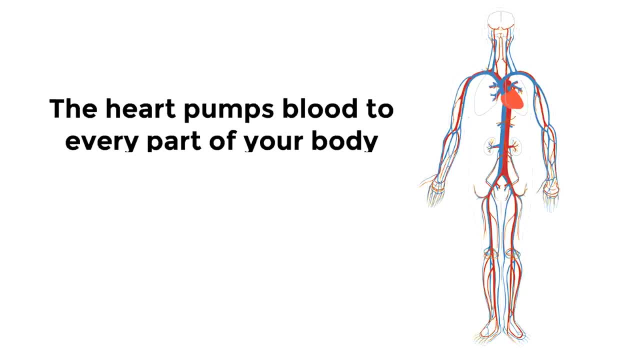 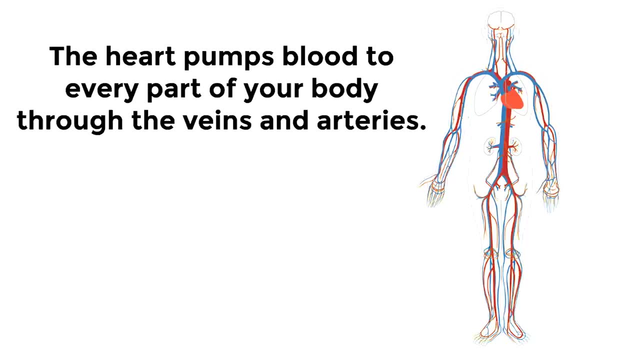 The heart pumps blood to every part of your body through the veins and arteries. This is called the circulatory system. It enables your entire body to get the oxygen and nutrients that it needs so you can be healthy and strong. The heart, What an amazing organ. 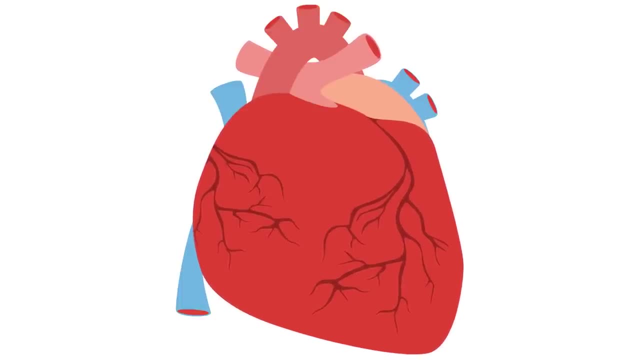 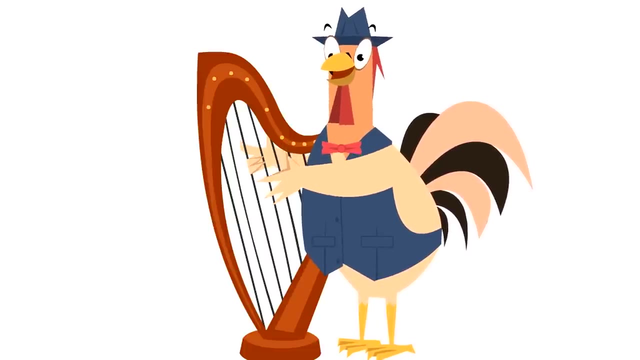 pumps blood through your body so you can stay strong and healthy. here's our friend Fred. we heard that he just took up the harp. he just started playing the harp. Fred, we can't. we can't hear you. we're having audio problems with Fred right now. Fred, you look so happy playing, we, we can't hear you. okay, you've got you. 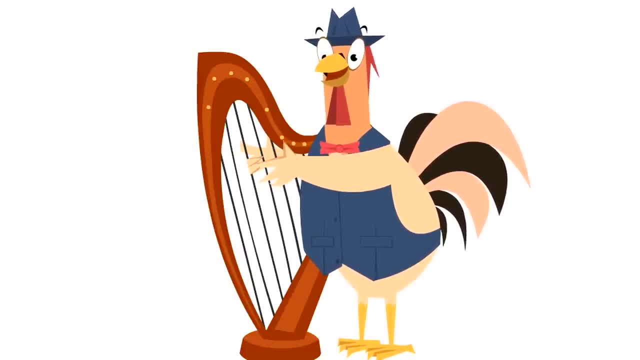 gotta wear your mic or something. we can't hear the music he doesn't even know. just you know. isn't that nice? you know Fred is just plucking away. he's having a good time- no kind of. we're having a good time right now with these. 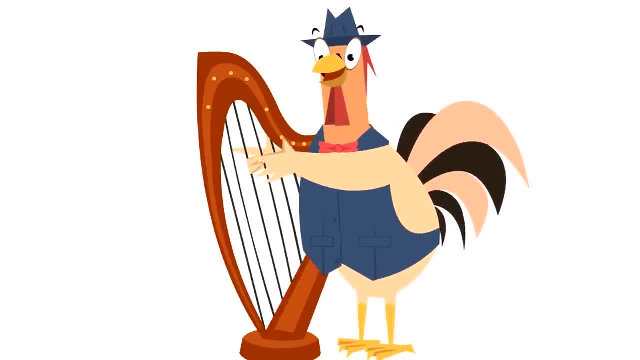 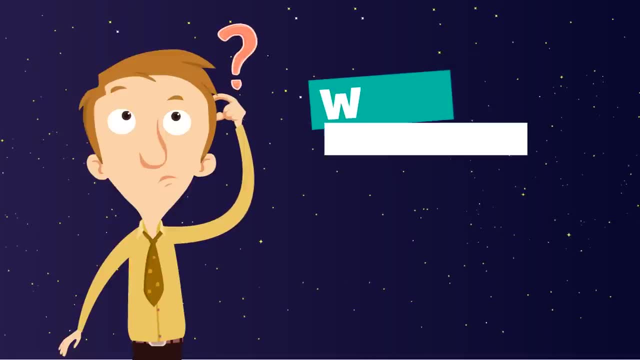 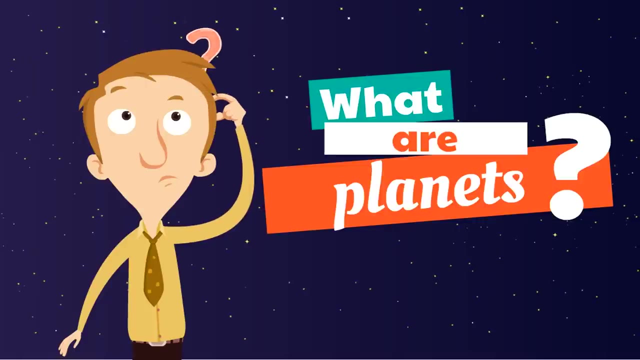 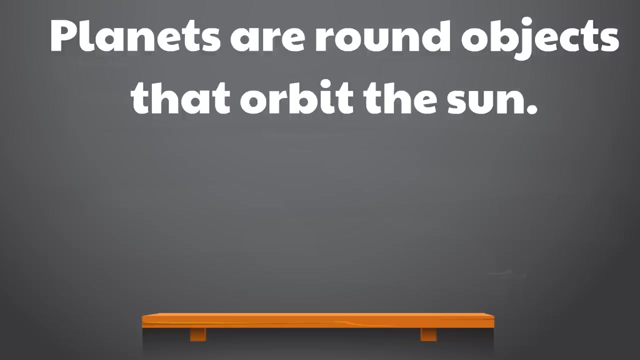 learning videos and next we are going to learn about the planets of the solar system. now, as we begin, we have to answer this question: what are planets? huh, there's some really good question. what are planets? planets are planets round objects that orbit the Sun. here is a picture of the Sun. it's the largest. 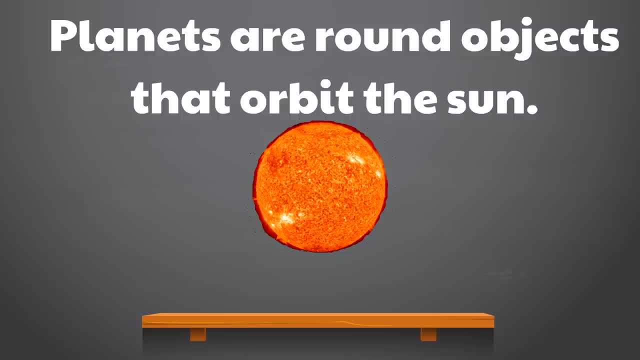 star in our solar system. it's massive and you can see there's a ring around. those are some solar flares fire shooting out of the Sun. absolutely amazing and stunning, and it kind of looks like a pizza. actually, the word orbit means to circle around. that means planets are round objects that circle. 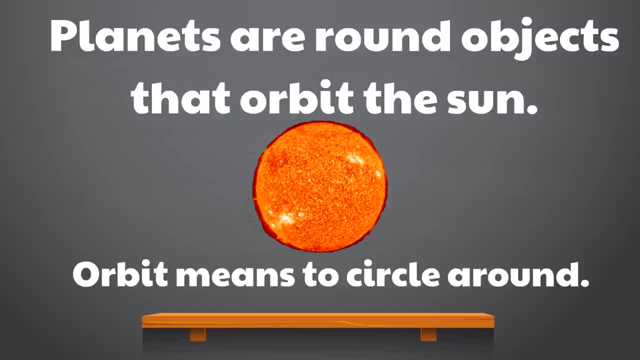 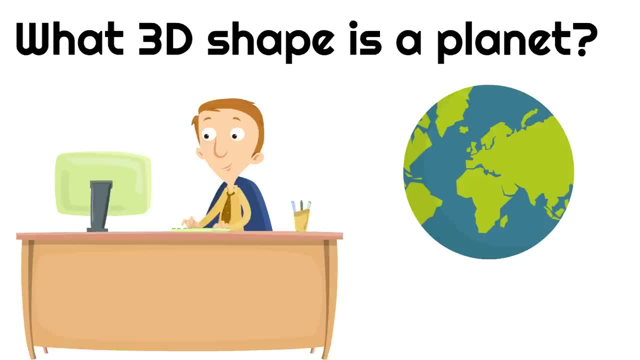 around the Sun. hey, what 3d shape is a planet? think about it. what 3d shape is a planet? we know that a planet is round. what 3d shape is perfectly round? yeah, a sphere. yeah, planets are spheres. they're perfectly round. good job. 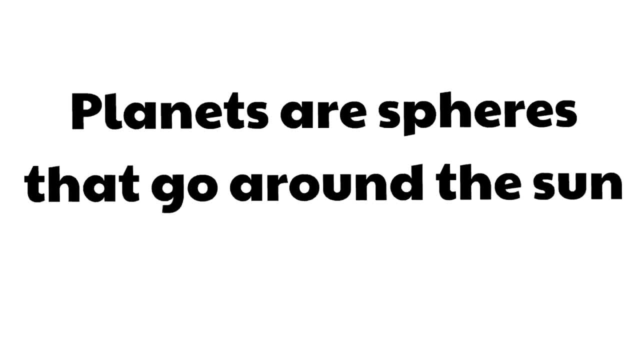 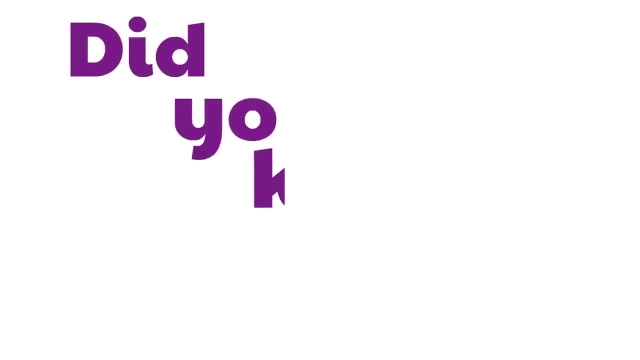 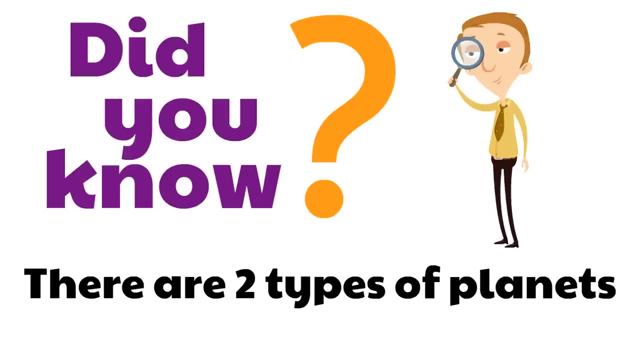 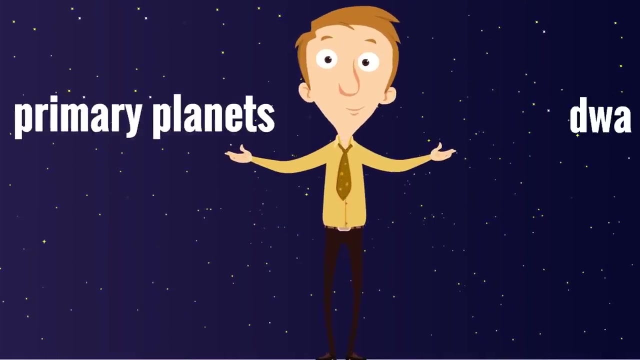 to summarize, planets are spheres that go around the Sun. pretty simple, huh. hey, did you know there are two types of planets? yeah, it's really interesting. there are two types of planets. ok, so there are primary planets and there are dwarf planets. those are the two types of planets. 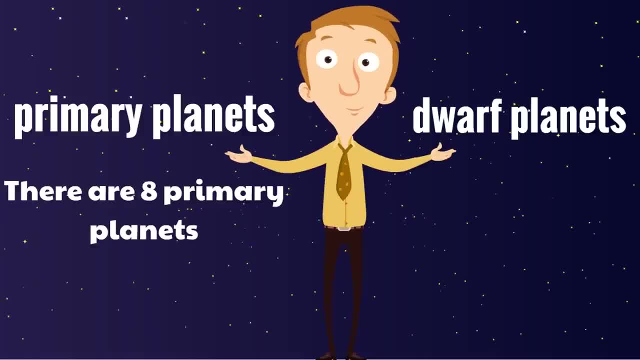 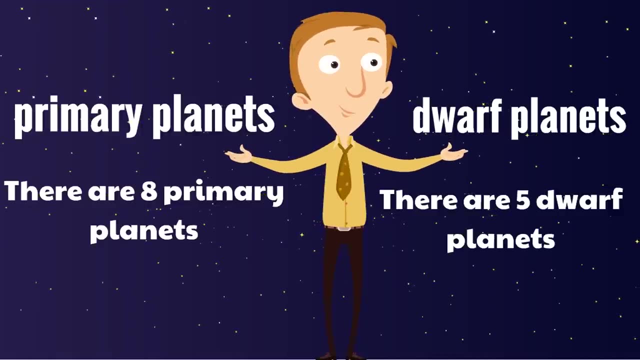 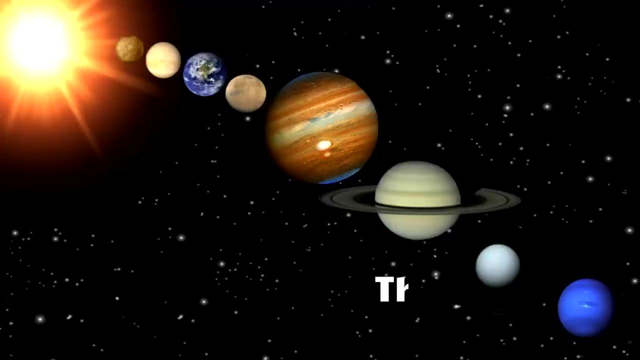 of the sun we're going to be studying in this video, and then there are five, eight of these primary planets. you're gonna know them so well. oh, my goodness, this is gonna be awesome. the first planet is mercury. mercury is the closest planet to the Sun. the second planet is Venus. pretty cool, huh. the second planet. 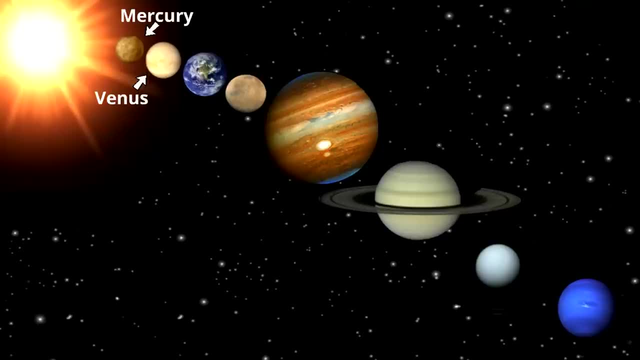 is Venus. our planet Earth is the third planet from the Sun. the fourth planet is Mars. Mars is the fourth planet. the fifth planet is Jupiter. that's the biggest planet of them all. the sixth planet is Saturn. you got to love those rings. Saturn is the sixth planet. Uranus is the 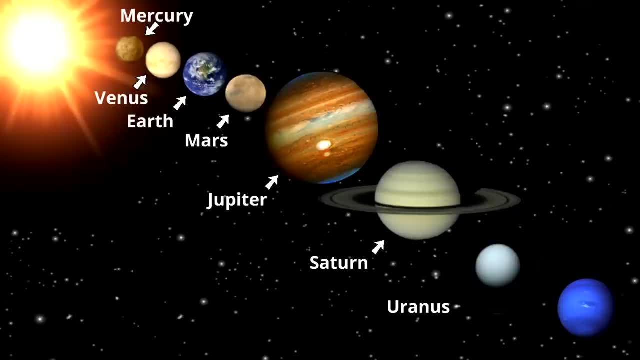 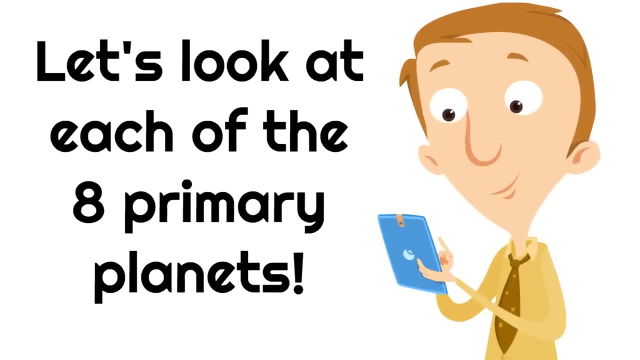 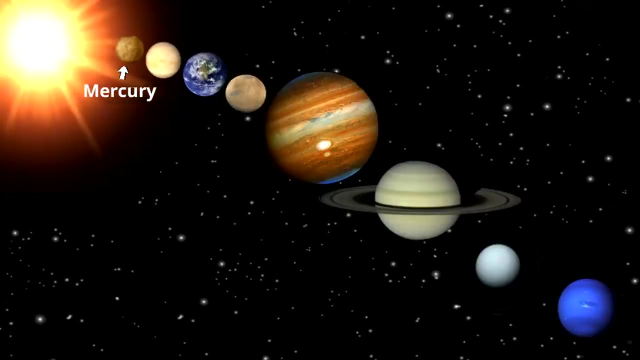 seventh planet and the eighth planet is Neptune. Neptune is the furthest primary planet from the Sun sun. Let's look at each of the eight primary planets. The first planet is Mercury. Here is where Mercury is. It is the closest planet to the sun. okay, The sun is super, duper hot. 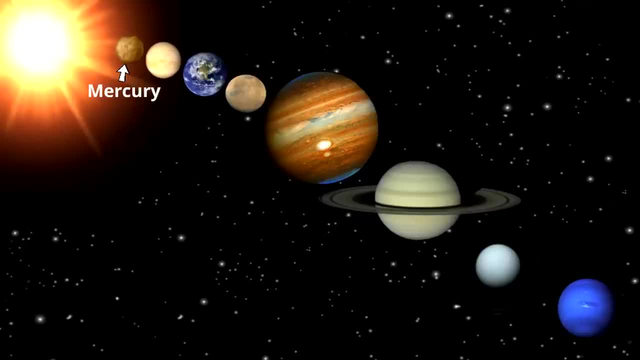 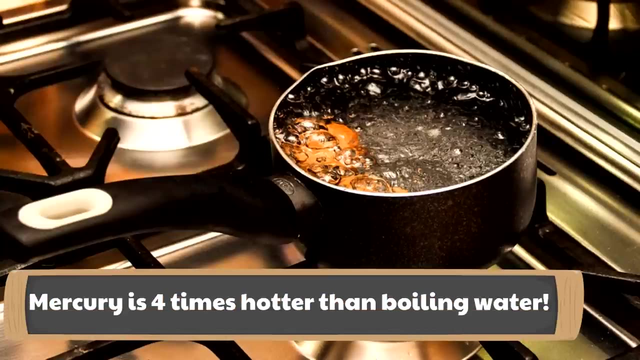 so guess what? Mercury is a really, really hot planet. In fact, Mercury is four times hotter than boiling water. Have you ever seen boiling water? It's so hot, It's boiling. It can cook things. It's really, really hot. If you barely touch it you will hurt yourself, so bad. 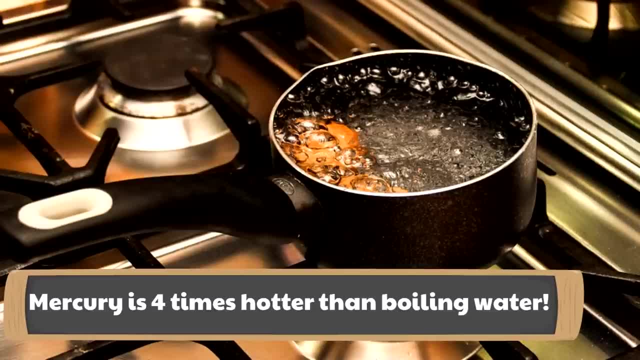 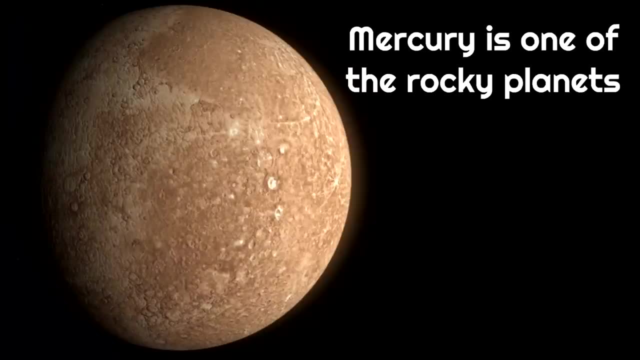 Well, Mercury is four times hotter than that. Oh my goodness. It is a very hot planet, Four times hotter than boiling water. Mercury is one of the rocky planets. There are four rocky planets and Mercury is one of them. Oh, and Mercury, it is the smallest primary planet. Mercury is so much. 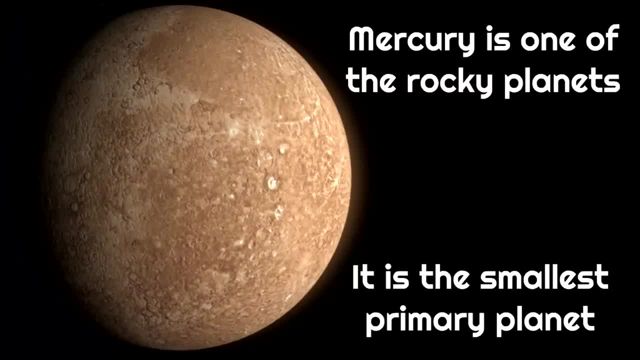 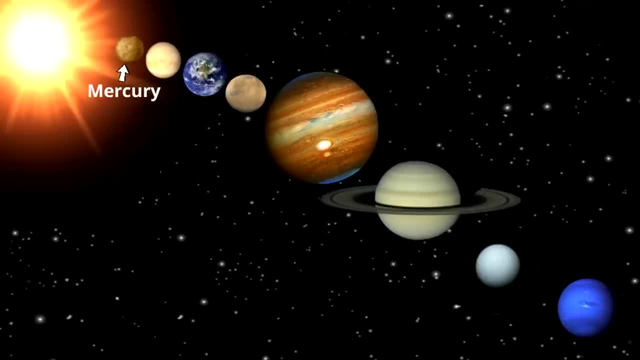 smaller than the other planets, Tiny little, little baby Mercury. It's the smallest planet of the primary planet. So if you think of a small planet, think of Mercury. It's small, It's hot. You wouldn't want to live there. The next planet, planet two. 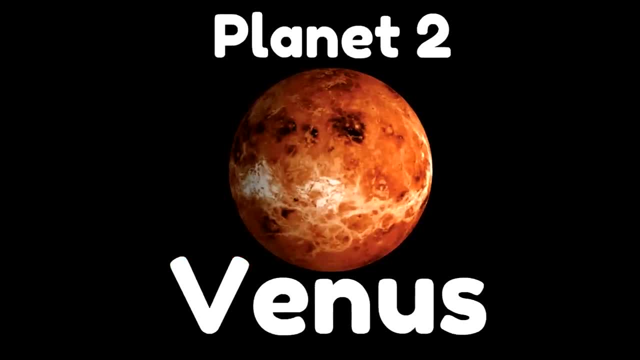 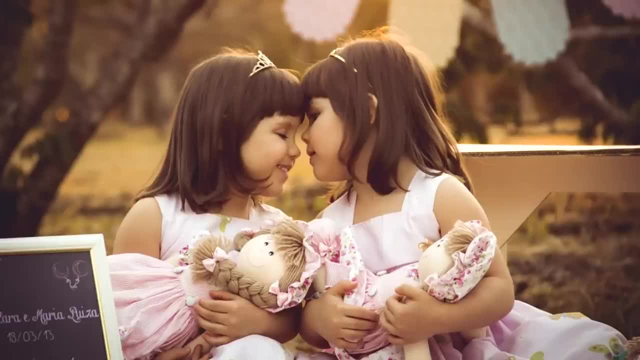 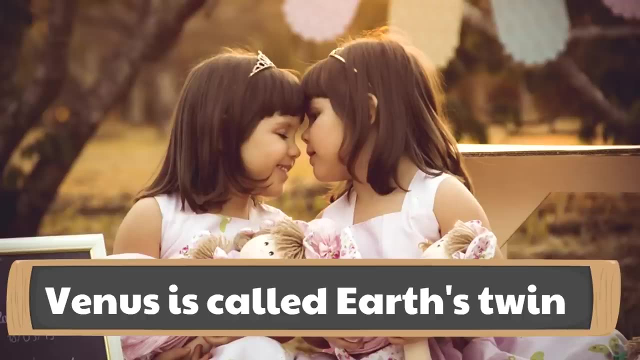 Venus. Venus is right here. It's the second planet from the sun. Now, this is interesting. Venus is called Earth's twin, and the reason for that is they are a very similar size. They're almost the same size And, what's interesting, they're both rocky planets, just like Mercury is. 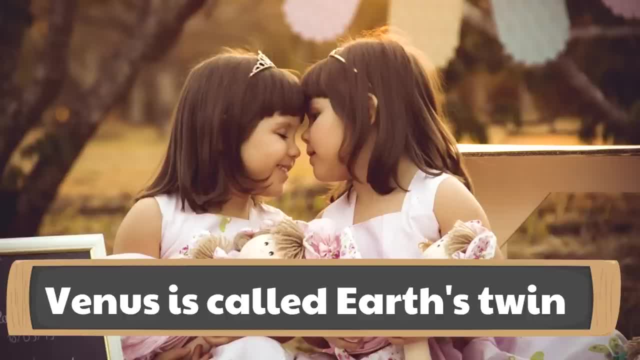 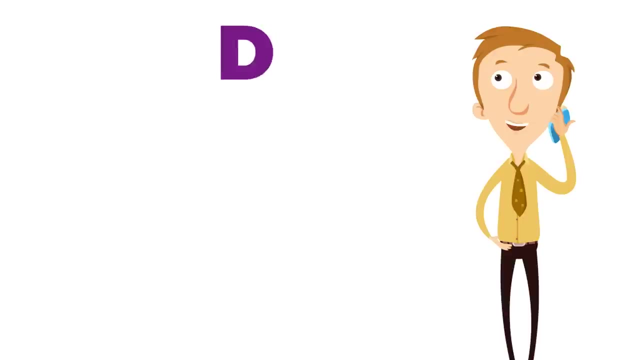 and Earth and Venus are made of similar rocks, So they're pretty much the same size, very similar size, and they're made of the same stuff. It's almost like the Earth and the planet Venus are twins. Hey, did you know? every day on Venus is a cloudy day and the clouds are yellow. 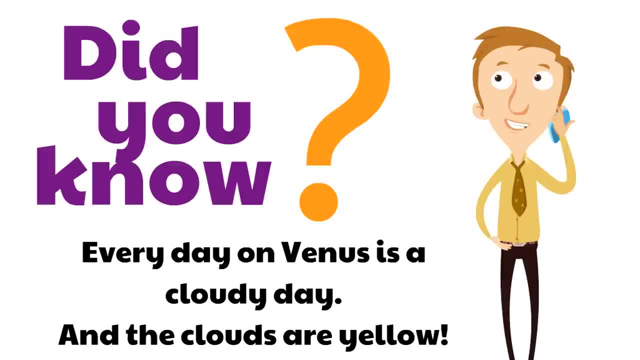 Oh, that's such a gross color for clouds. Clouds are much better when they're other colors than yellow. so the sunlight doesn't actually hit the surface of Venus. so it's not raining and it's not warm. it's just a cloudy day every day forever. but that's okay. 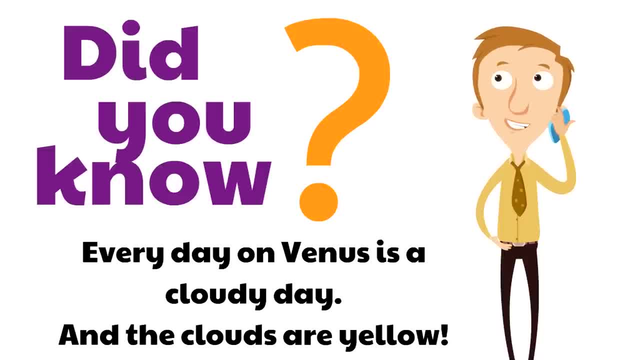 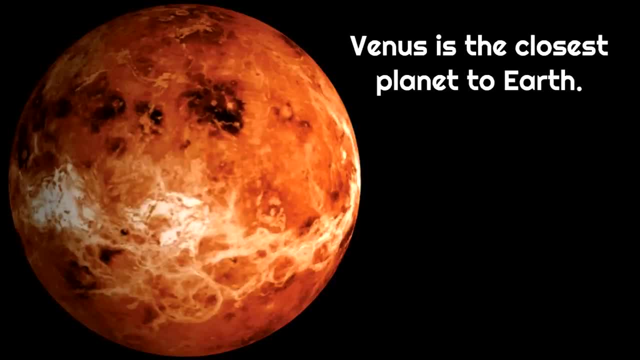 because there's no life on Venus, so nobody's crying about it. And this is cool. Venus is the closest planet to Earth. It is the easiest planet to see in the sky, You don't even need a telescope. How cool is that. 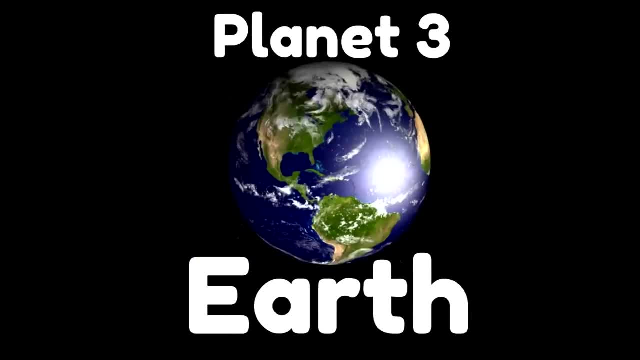 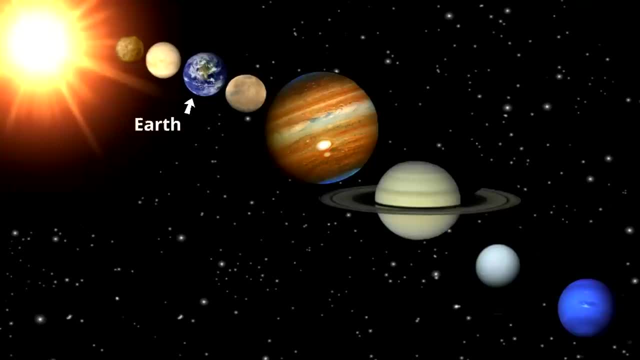 The third planet is well, ours, the Earth. The Earth is the ugliest planet on earth. even moving the earth, the earth is the third planet. here is where the earth is. yep, it's the third planet, from the Sun, by the way. 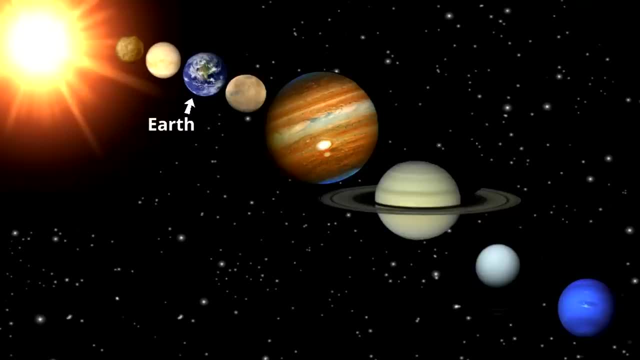 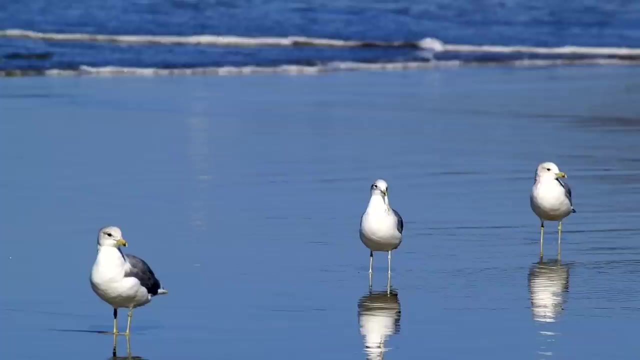 these planets never line up like this. we just have it like this so you can see the order of the planets, but they're normally very, very jumbled. they don't line up like this. just wanted to share that. but the earth is the third planet from the Sun. here's a picture of the ocean and some seagulls that are in some. 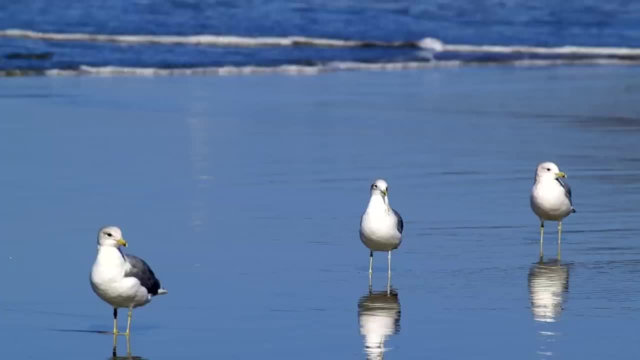 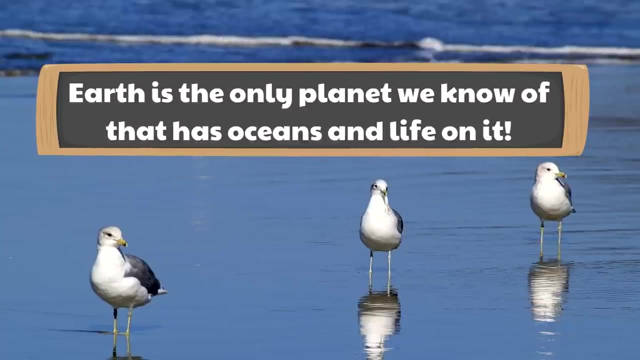 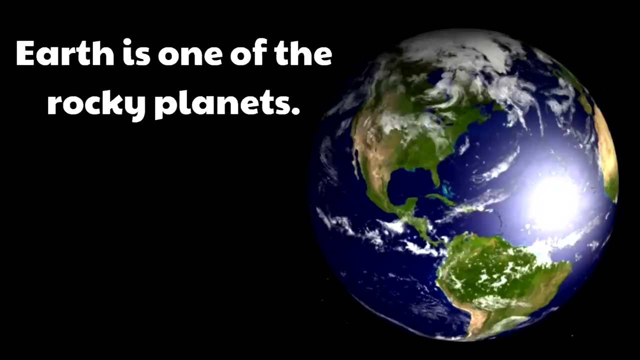 of the shallow parts of the water. it's interesting: earth is the only planet we know of that has oceans and life on it. earth is one of the rocky planets. yeah, we live on a massive rock that has oceans, that has life. I mean, that's absolutely incredible. 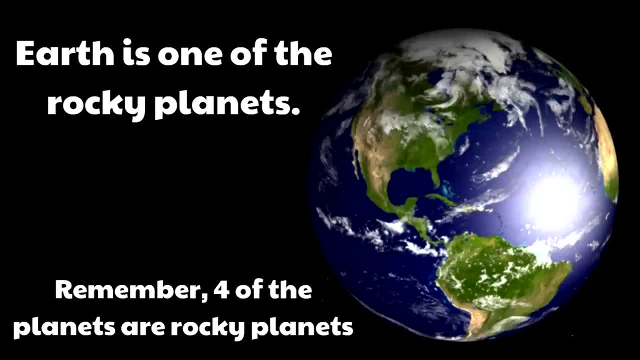 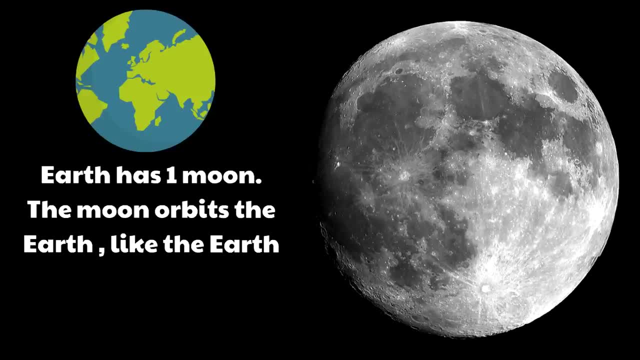 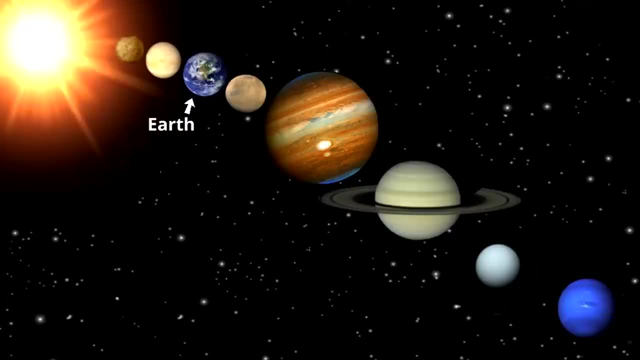 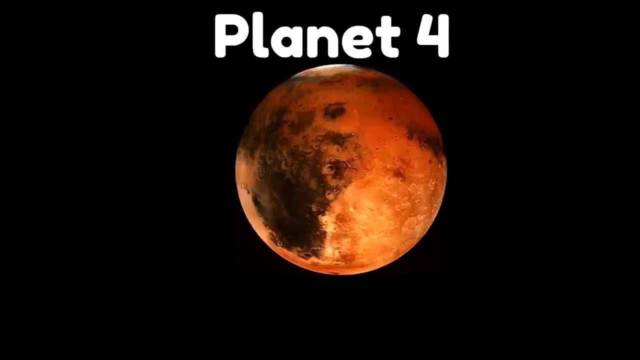 remember, four of the planets are rocky planets. earth has one moon. the moon orbits the earth like the earth orbits the Sun. Wow, there's our planet. that's where we live, the earth. the fourth planet is Mars. Mars is right here in the hot environment. we're gonna edit it out when we come back. 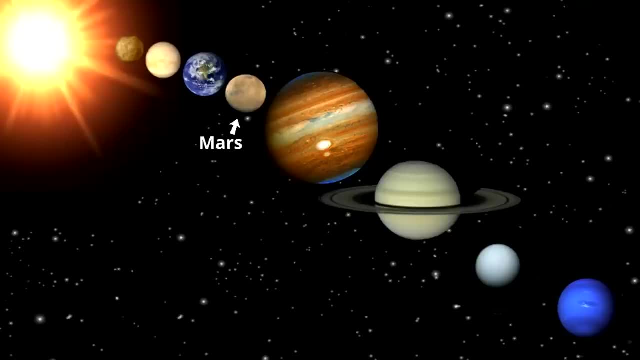 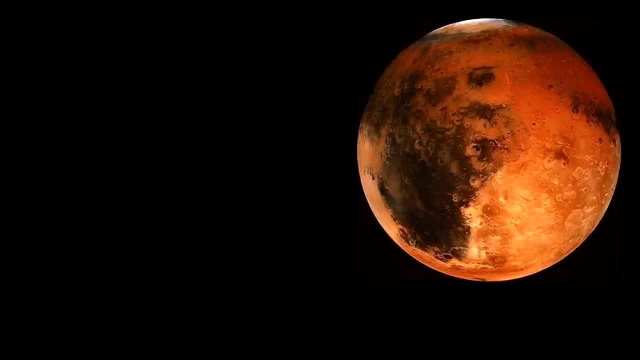 between Earth and Jupiter. What color is Mars? Look at Mars. What color is that? Yeah, it's kind of like a reddish orange. Because of its color, Mars is called the Red Planet. So if anyone asks you what's the Red Planet, Tell them: hey, the Red Planet is Mars, Even. 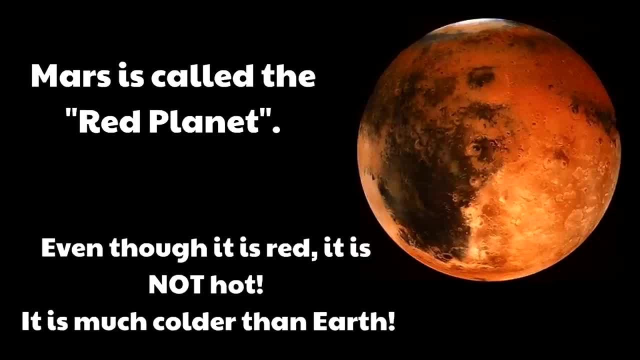 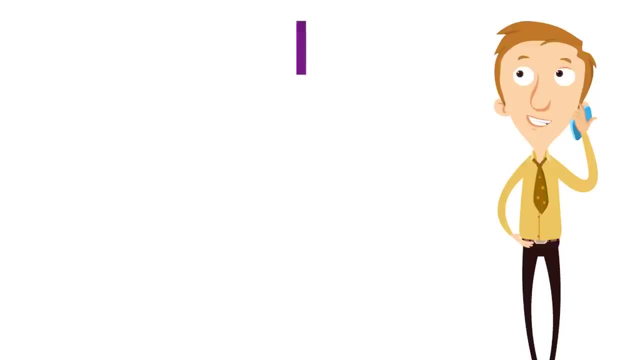 though it is red, it is not hot. It is much colder than Earth because, remember, Mars is further from the sun than the Earth. So Mars it's red, it almost looks like it would be hot, but it's cold. Hey, is there life on Mars? That's a really good question that. 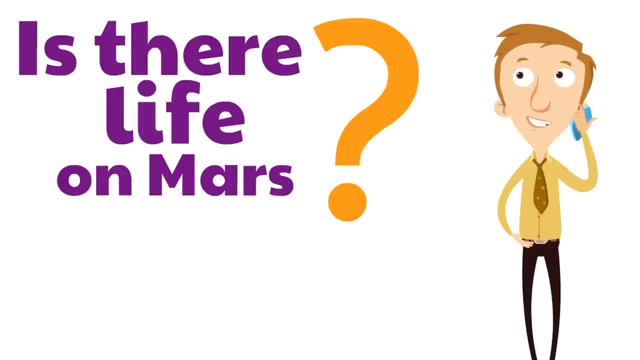 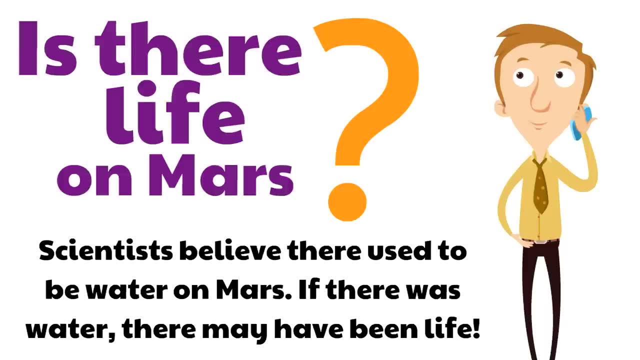 a lot of scientists have been trying to answer for a long time. Well, scientists believe there used to be water on Mars. If there was water, there may have been life. And, even stranger, there are some scientists that believe we may still find basic forms of life still living on Mars. 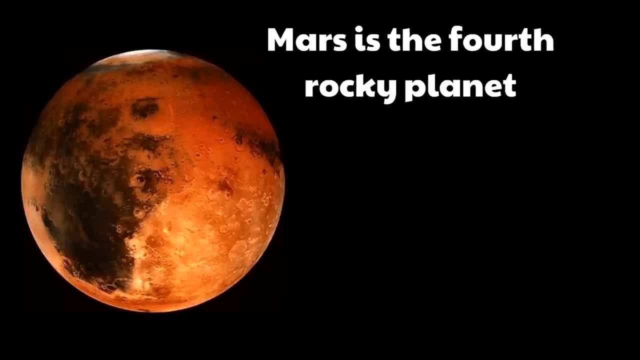 Mars is the fourth rocky planet. Remember, we said there are only four rocky planets, so it's the last of the rocky planets. Mars has volcanoes And valleys, just like Earth. they're just sometimes much bigger. In fact, there's a. 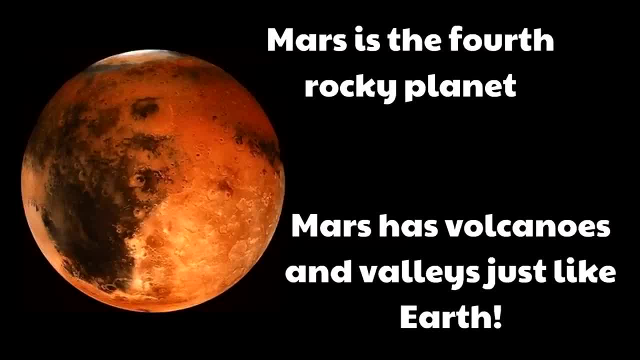 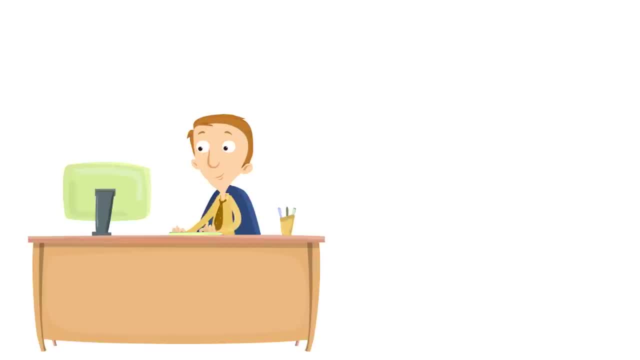 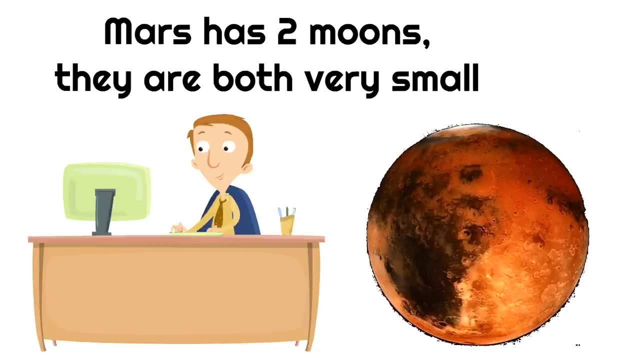 volcano on Mars that's as big as the state of Texas- Wow, Huge, And this is kind of cool. Mars has two moons. They are both very small. They're small moons, which is good. Mars has a couple moons. It's nice We've got a moon. Mars has two moons. 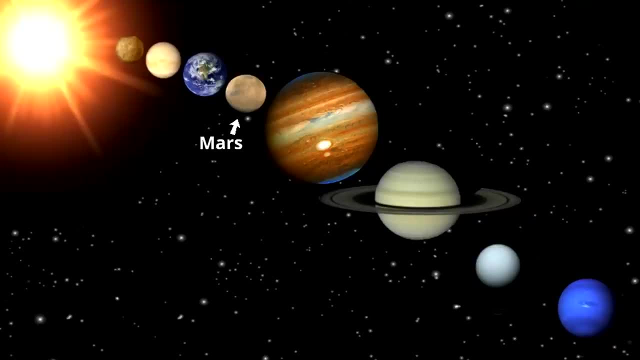 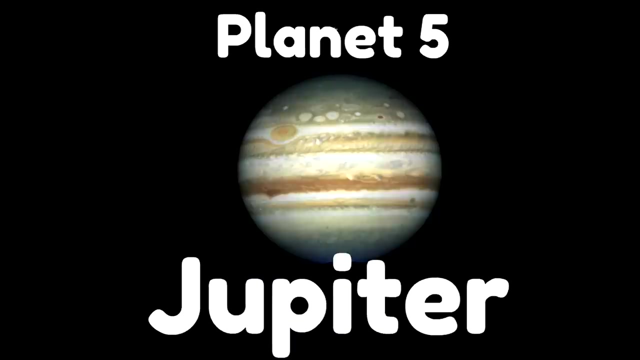 You know, OK, Wow, This is actually very unique. The surpluses are nggak Ha good job. Wow, that's very cool. Wow, The sun's around here. but where in the world were the suns and the gas planets? 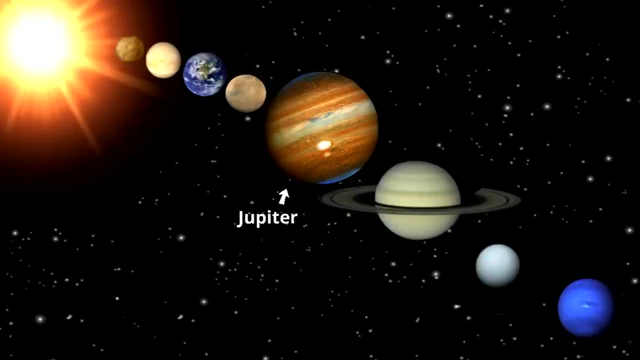 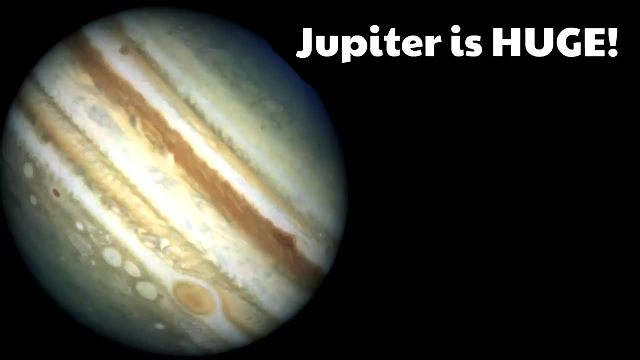 Well, there were gas planets and the gas planets. There was a lot of gas and there was so much natural resources. But look, It's a huge planet. So what system? in fact, all of the other planets could fit in Jupiter, and there would be. 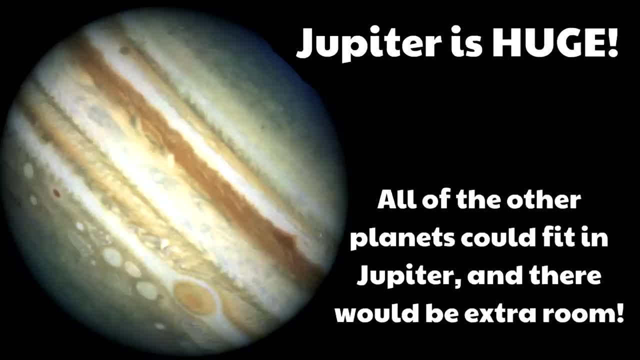 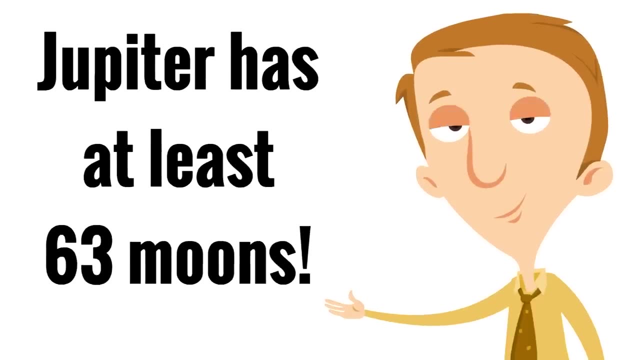 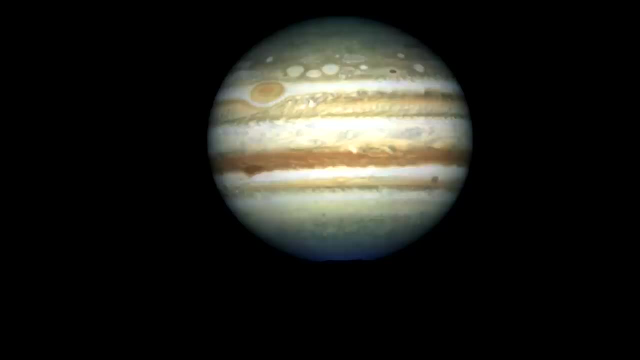 extra room. all of the other planets could fit inside of Jupiter. that's how big Jupiter is and this is amazing. Jupiter has at least 63 moons, and we say at least because they're still discovering more, Wow, and because Jupiter is a gas planet. if you ever visited it, you would just fall right through, just 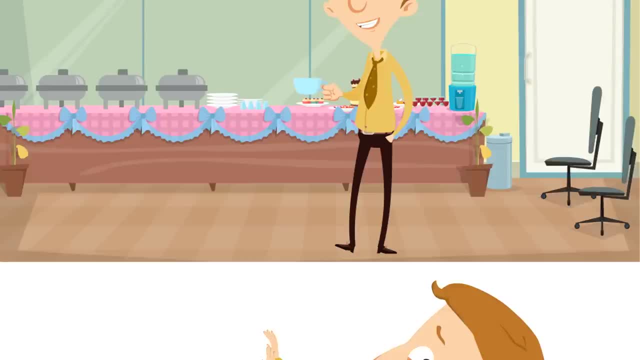 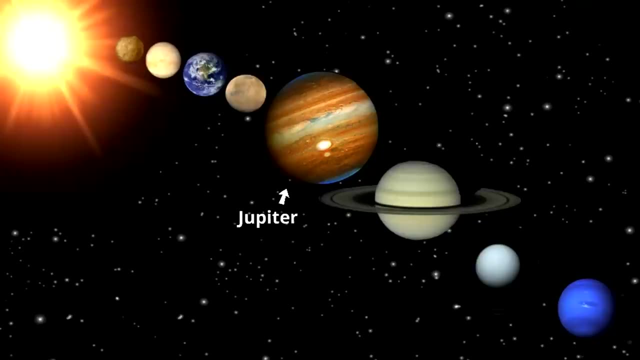 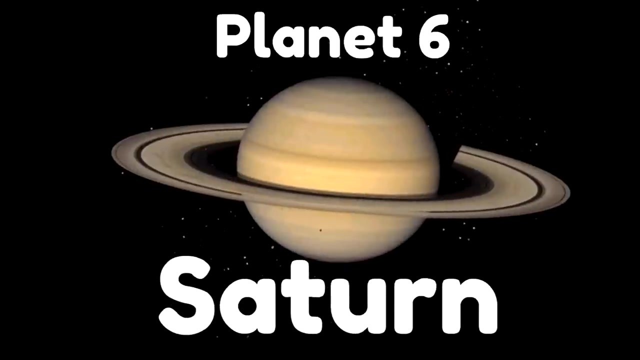 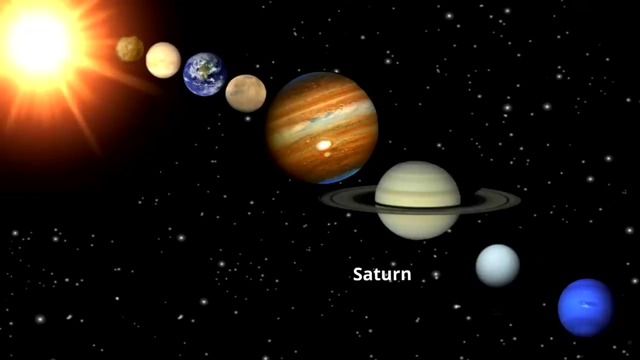 kidding you would float. I mean they wouldn't fall, the gravity wouldn't be there, you would just kind of float around. you know, Jupiter is the giant gas planet in between Mars and Saturn. the sixth planet is Saturn. another gas planet here is Saturn, the sixth planet from the Sun. you could spot it easily because of those huge rings and it's in. 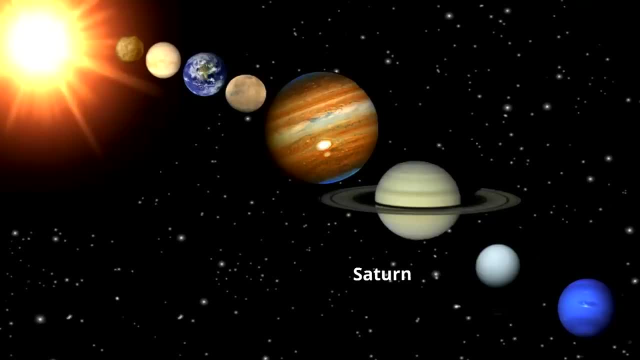 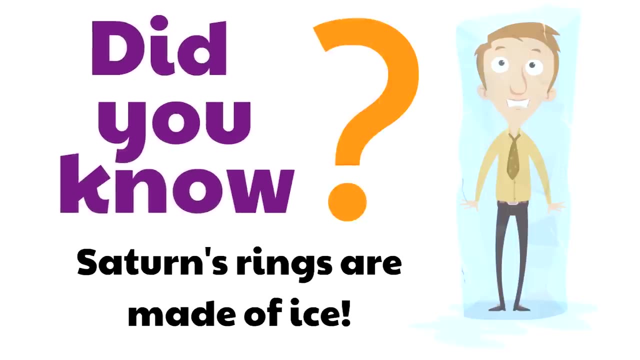 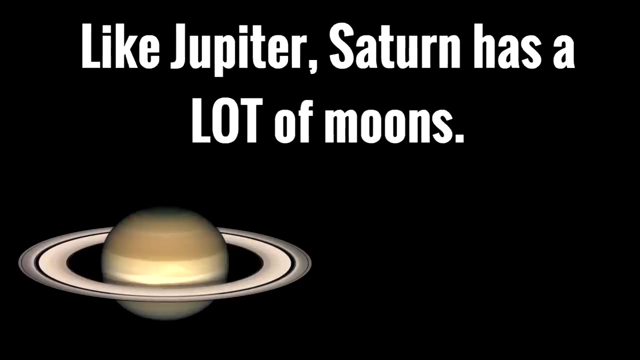 between Jupiter and Uranus. hey, did you know Saturn's rings are made of ice? oh, my goodness, how cool that must be. whoo, no, icy rings, those rings are made of ice. Wow, like Jupiter, Saturn has a lot of moons. Saturn has 62 moons. Wow, tons and tons of moons. what's up with Jupiter and Saturn? right? 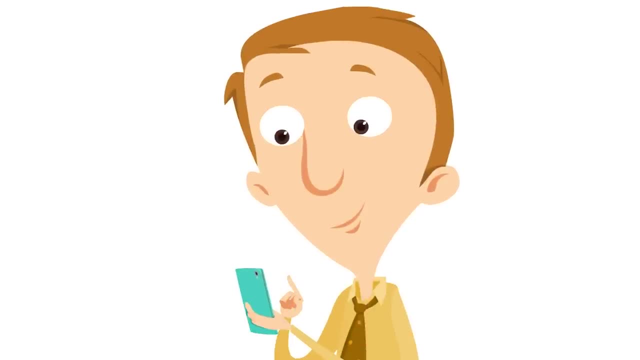 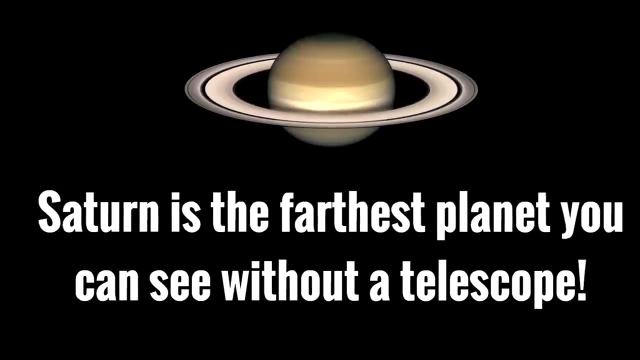 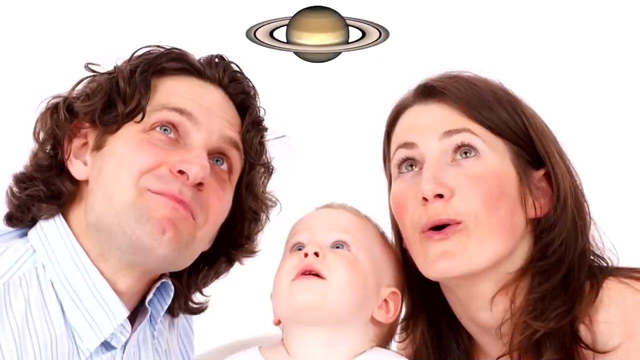 and now? this is pretty awesome. Saturn is the farthest planet you can see without a telescope. That's right, you can see Saturn with your own eyes, without a telescope. Look, Mommy and Daddy, I see Saturn with my own eyes. There's Saturn. I see the rings and everything. Saturn is. 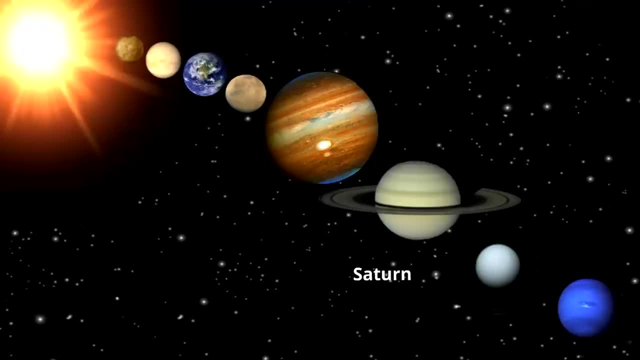 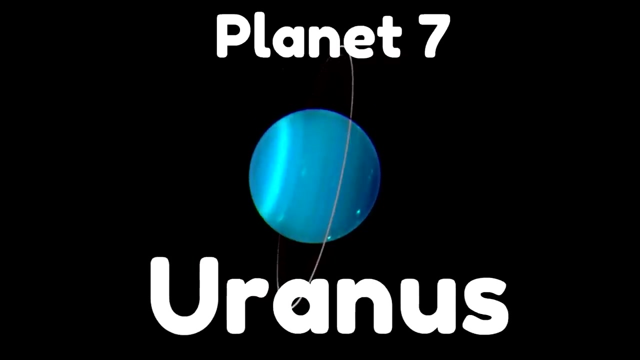 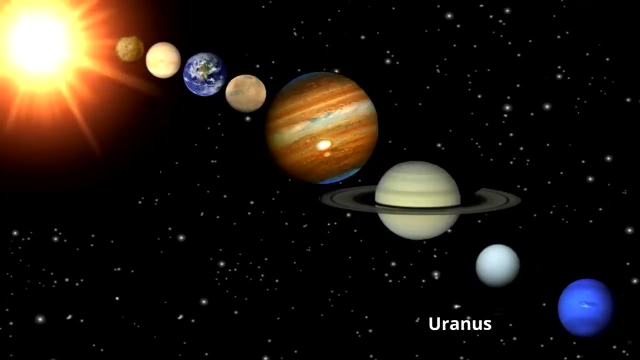 a gas planet. that's the 6th planet from the Sun and is in between Jupiter and Uranus. The 7th planet is Uranus, another gas planet. Uranus is the 7th planet from the Sun and is in between Saturn and Neptune. Both Uranus and Neptune are the only planets that are 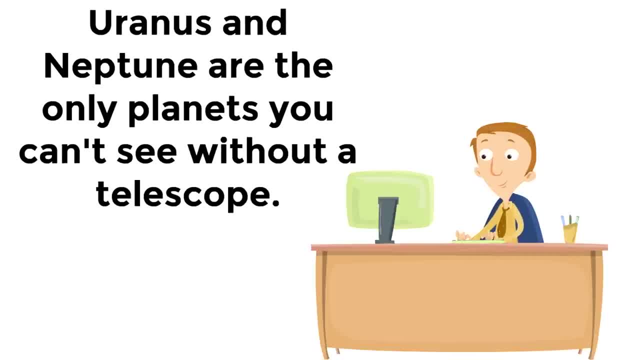 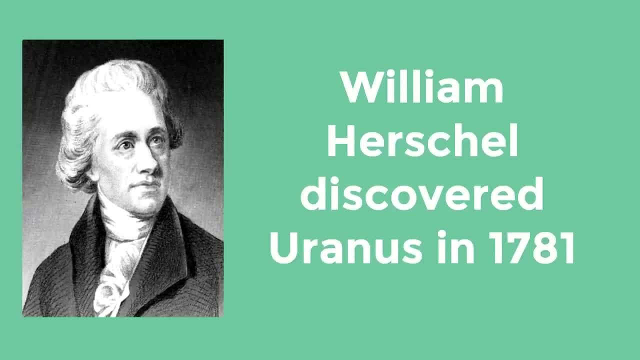 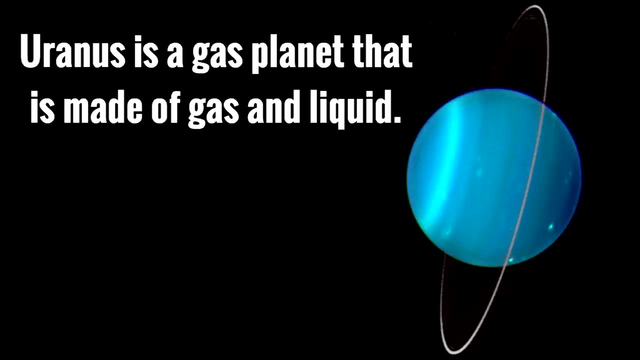 you can't see without a telescope, so it took a while for them to be discovered. Now this is neat. William Herschel discovered Uranus in 1781.. It took us a long time to finally find the planet Uranus. Uranus is a gas planet that is made of gas and liquid. What's cool is Uranus has rings. 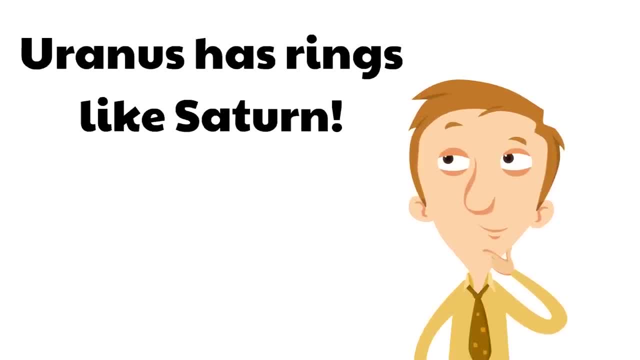 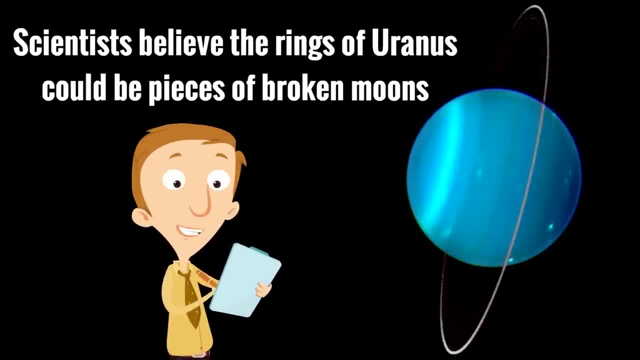 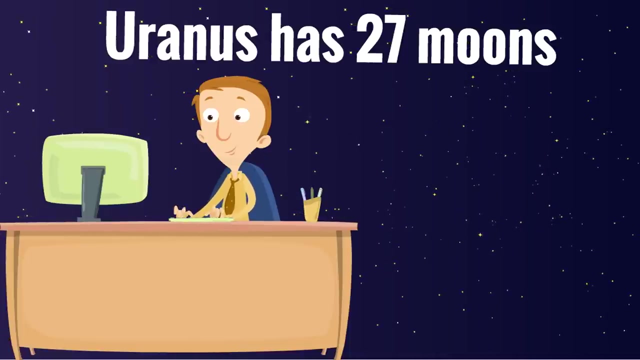 just like Saturn has rings. Yeah, Scientists believe the rings of Uranus could be pieces of broken moons. We don't know for sure, but that's really fascinating if that's the case. Speaking of moons, Uranus has 27 moons. 27 moons, I mean, we just have one, 27.. 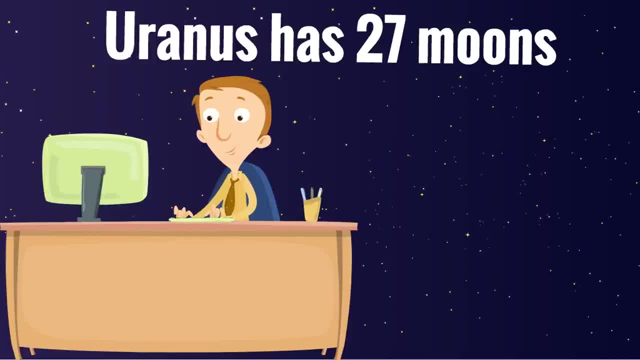 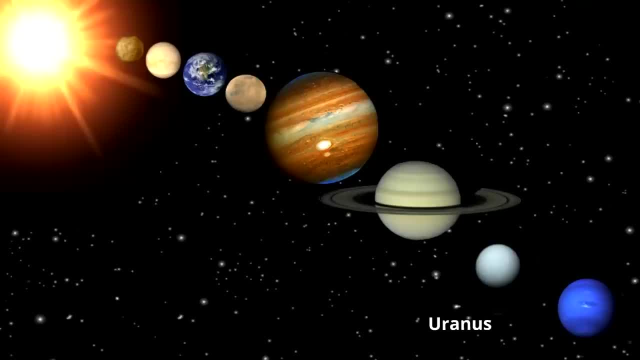 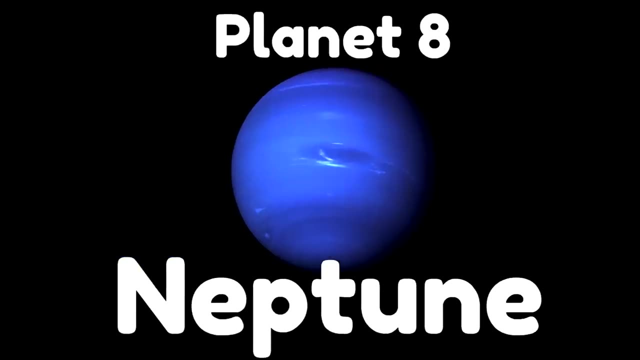 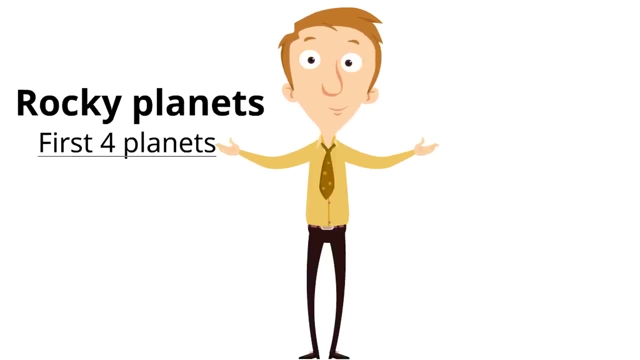 Uranus is the 7th planet from the Sun and is in between Saturn and Neptune. They're the only planets in the universe that have rings. The 8th and final planet is Neptune, And that is Neptune. Hey, That means the first 4 planets are rocky planets and the last 4 planets are gas planets. 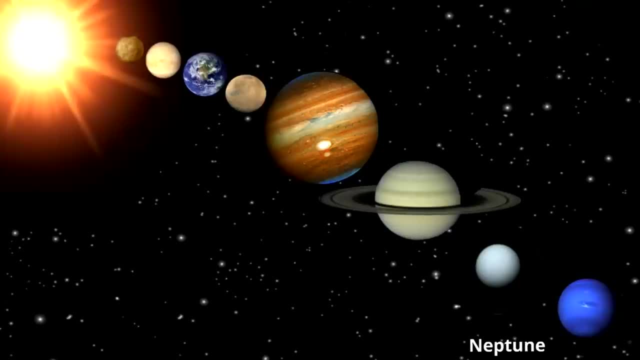 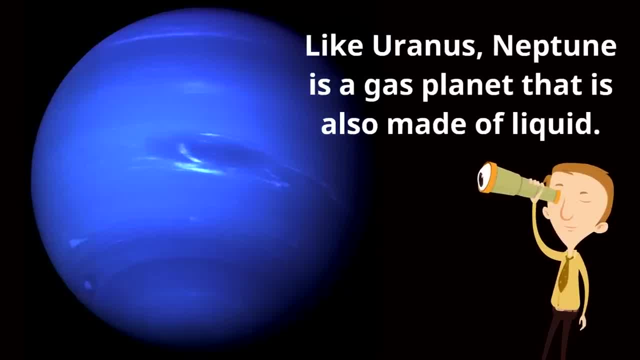 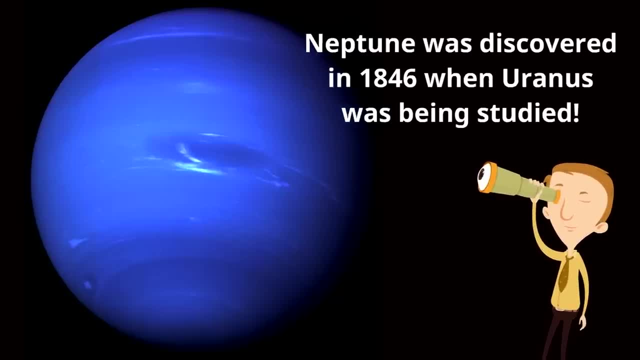 also made of liquid. Neptune was discovered in 1846 when Uranus was being studied. They're like: wait a second, there's a whole nother planet here on the end. let's call it Neptune. Neptune is known for its storms, the worst storms in. 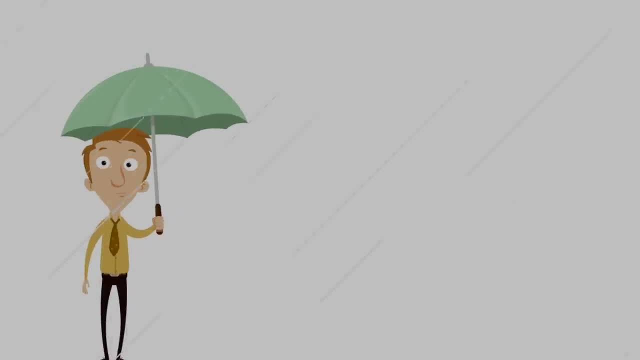 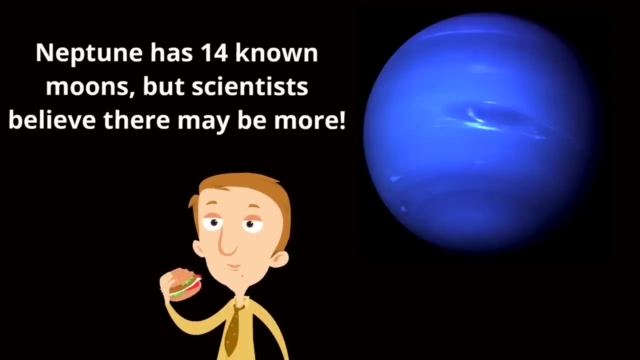 the solar system. In fact, winds reach over 1,000 miles per hour on Neptune. whoo, that's pretty intense. Neptune has 14 known moons, but scientists believe there may be more. Here's Neptune, the furthest planet from the moon. Here's Neptune, the furthest planet from the moon. 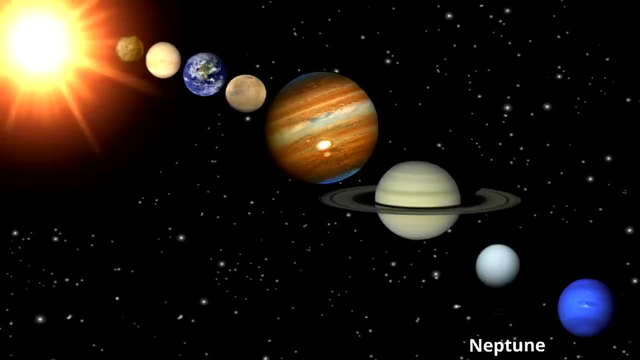 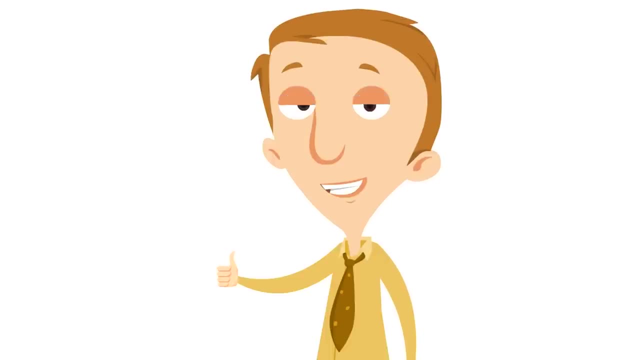 Here's Neptune, the furthest planet from the moon. Here's Neptune, the furthest planet from the sun. You have done such an amazing job from the sun. You have done such an amazing job from the sun. You have done such an amazing job with us today. Today, we learned. 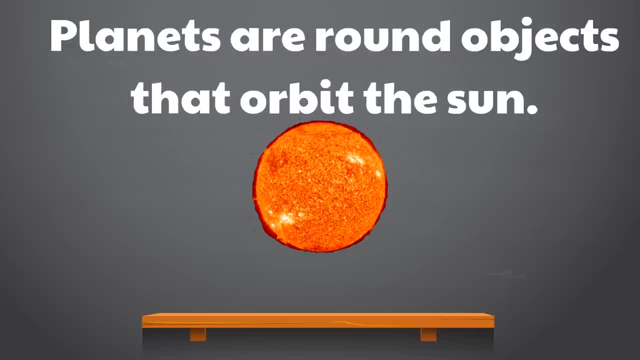 with us today. Today, we learned. with us today, Today we learned: planets are round, objects that orbit. planets are round objects that orbit. planets are round objects that orbit the Sun. The word orbit means to circle the Sun. The word orbit means to circle the Sun. The word orbit means to circle around. Basically, the planets are round. 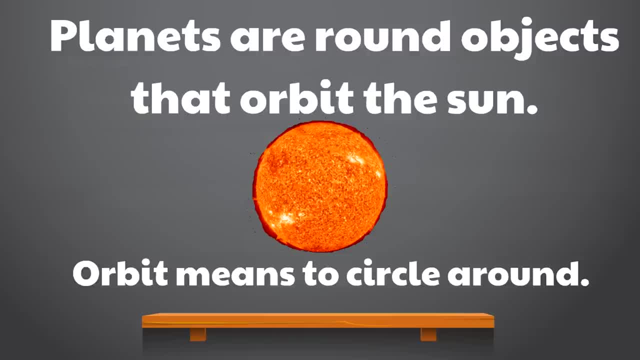 around. Basically, the planets are round around. Basically, the planets are round objects that go around the Sun. We learn objects that go around the Sun. We learn objects that go around the Sun. We learn there are two types of planets. there are two types of planets. there are two types of planets that go around the Sun. We learn there are two types of that go around the Sun. We learn there are two types of that go around the Sun. We learn there are two types of planets: Primary planets and planets Primary planets and. 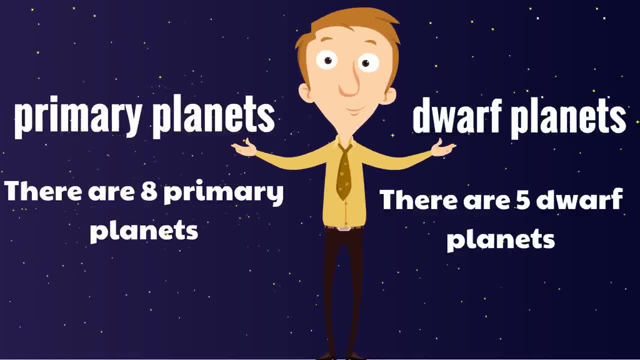 planets, Primary planets, and there are eight primary planets and there are eight primary planets and there are eight primary planets and dwarf planets. There are five dwarf dwarf planets. There are five dwarf dwarf planets. There are five dwarf planets And here are all eight primary. 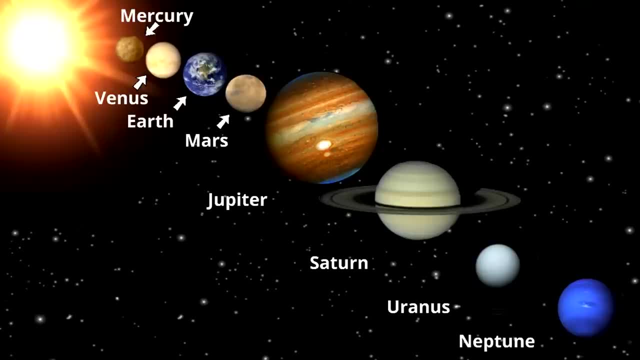 planets. And here are all eight primary planets, And here are all eight primary planets. They're familiar friends, now planets. They're familiar friends, now planets. They're familiar friends now: Mercury, Venus, Earth, Mars, Jupiter, Saturn. 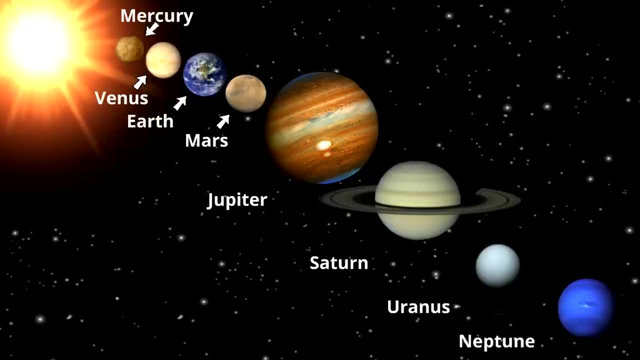 Mercury, Venus, Earth, Mars, Jupiter. Saturn, Mercury, Venus, Earth, Mars, Jupiter, Saturn, Uranus and Neptune. The first four: Saturn, Uranus and Neptune. The first four: Saturn, Uranus and Neptune. The first four planets are rocky planets: Mercury. 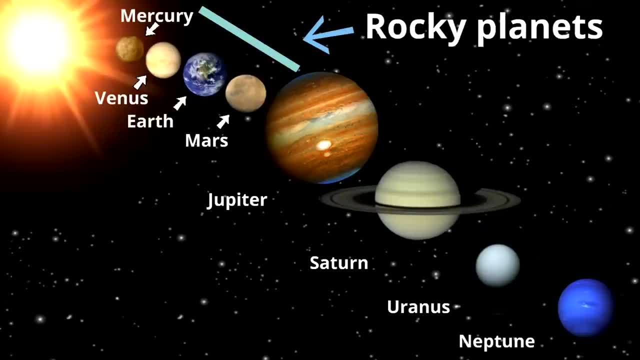 planets are rocky planets. Mercury planets are rocky planets. Mercury, Venus, Earth and Mars are rocky planets. Venus, Earth and Mars are rocky planets. Venus, Earth and Mars are rocky planets- The four planets furthest from the Sun. The four planets furthest from the Sun. 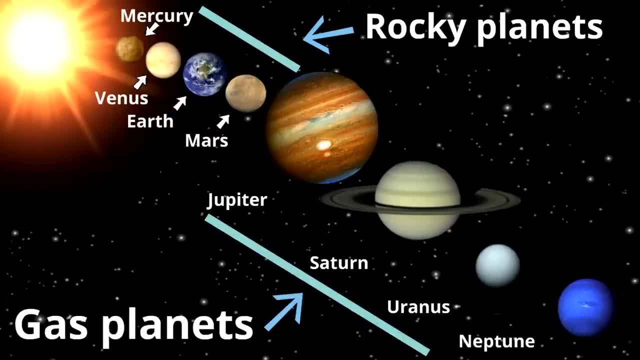 The four planets furthest from the Sun are the gas planets. Jupiter, Saturn are the gas planets. Jupiter, Saturn are the gas planets. Jupiter, Saturn, Uranus and Neptune are gas planets. You're doing great, You're increasing. 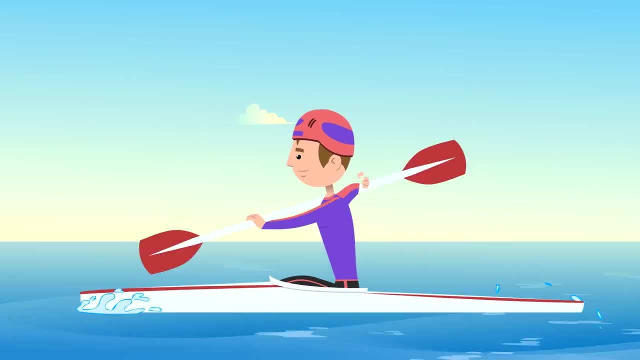 You're doing great. You're increasing. You're doing great. You're increasing your skills. just like this racer. your skills, just like this racer. your skills, just like this racer racing on the water. You're increasing racing on the water. You're increasing racing on the water. You're increasing your skills. You're doing a wonderful job. 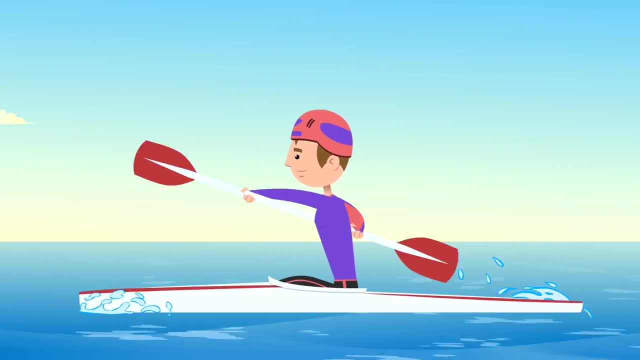 your skills, You're doing a wonderful job. your skills, You're doing a wonderful job, and next we are going to learn about, and next we are going to learn about, and next we are going to learn about sharks- Sharks. this is a video, so 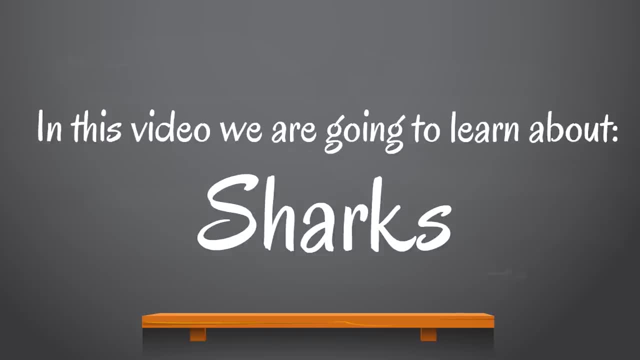 sharks Sharks. this is a video. so sharks Sharks. this is a video. so many of you have asked for It's time. many of you have asked for It's time. many of you have asked for It's time. It's time for the shark video. 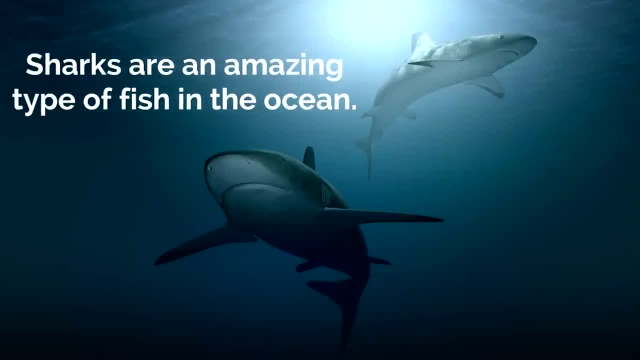 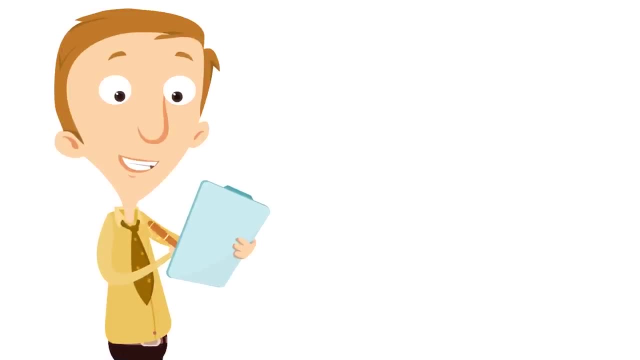 Sharks are an amazing type of fish in. Sharks are an amazing type of fish in. Sharks are an amazing type of fish in the ocean, the ocean, the ocean. Isn't that interesting Sharks are? Isn't that interesting Sharks are? Isn't that interesting Sharks are fish. Sharks are amazing fish. Now the 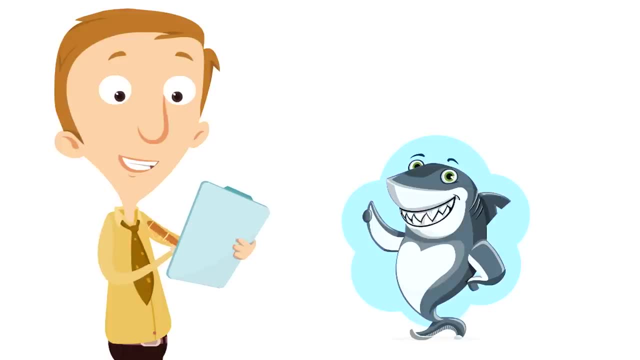 fish Sharks are amazing fish. Now, the fish Sharks are amazing fish. Now, the picture most of us have in our minds, picture most of us have in our minds, picture most of us have in our minds when we think of sharks, isn't always the 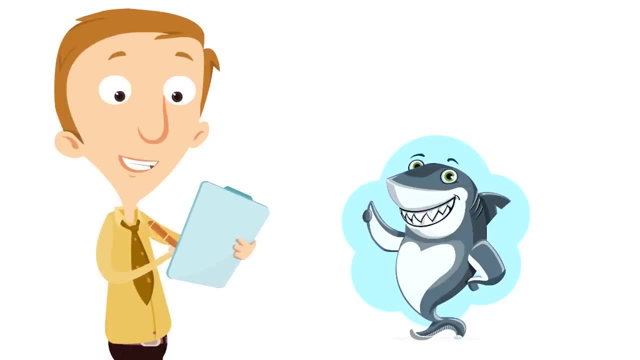 when we think of sharks isn't always the when we think of sharks isn't always the case. You see, there are 440 types of case. You see there are 440 types of case. You see there are 440 types of sharks and they can be quite different. 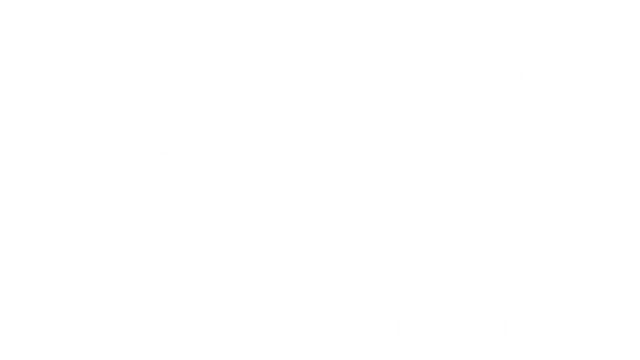 sharks and they can be quite different sharks and they can be quite different from one another, For example, the whale from one another. For example, the whale from one another. For example, the whale shark is the largest type of shark. It shark is the largest type of shark. It. 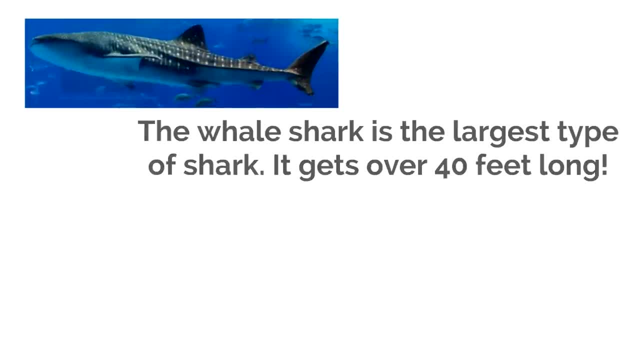 shark is the largest type of shark. It gets over 40 feet long- Wow. But the gets over 40 feet long- Wow. But the gets over 40 feet long- Wow. But the dwarf lantern shark is the smallest shark. dwarf lantern shark is the smallest shark. 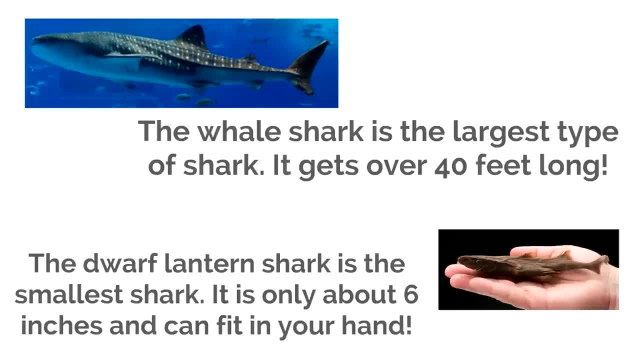 dwarf lantern shark is the smallest shark. It is only about six inches and can fit. It is only about six inches and can fit. It is only about six inches and can fit in your hand. Wow, This is not what most in your hand. Wow, This is not what most. 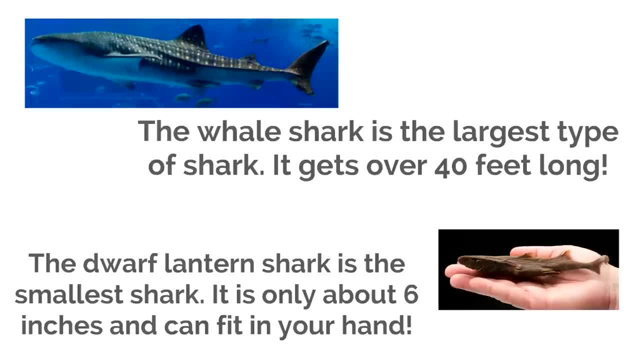 in your hand. Wow, This is not what most people picture when they picture a shark. people picture when they picture a shark. people picture when they picture a shark, But the dwarf lantern shark is just as. But the dwarf lantern shark is just as. 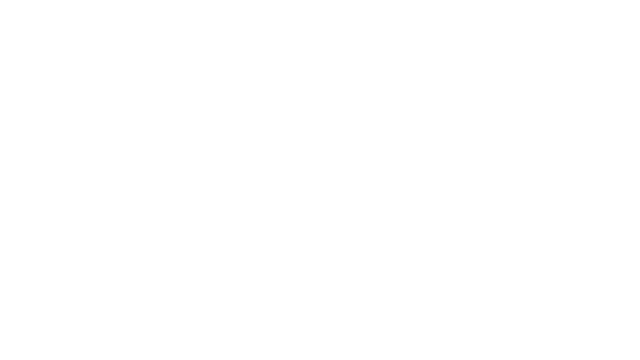 But the dwarf lantern shark is just as much a shark as the whale shark is much a shark as the whale shark is much a shark as the whale shark is. Remember there are 440 types of sharks. Remember, there are 440 types of sharks. 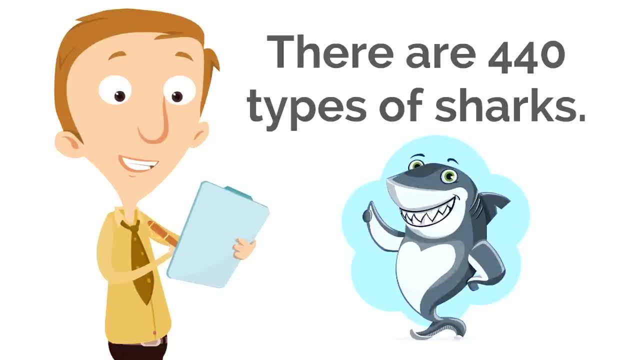 Remember, there are 440 types of sharks, so they don't all look like this guy. so they don't all look like this guy. so they don't all look like this guy. you know, Here's the thing, even though. you know, Here's the thing, even though. 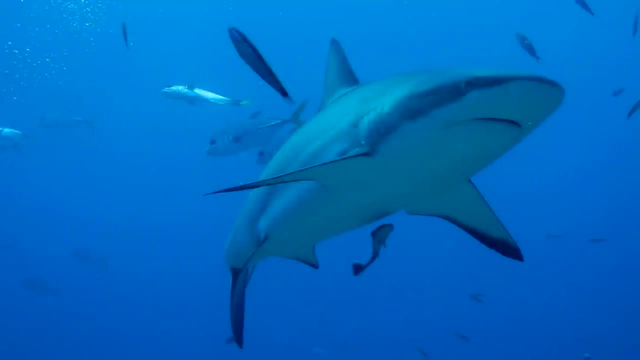 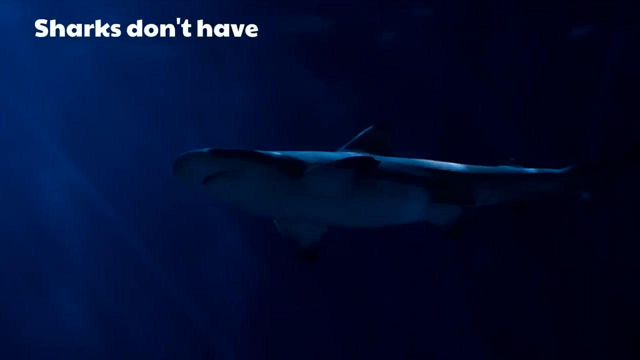 you know, Here's the thing: even though there are so many different types of, there are so many different types of, there are so many different types of sharks, all sharks have certain things in sharks. all sharks have certain things in sharks. all sharks have certain things in common. For example, sharks don't have 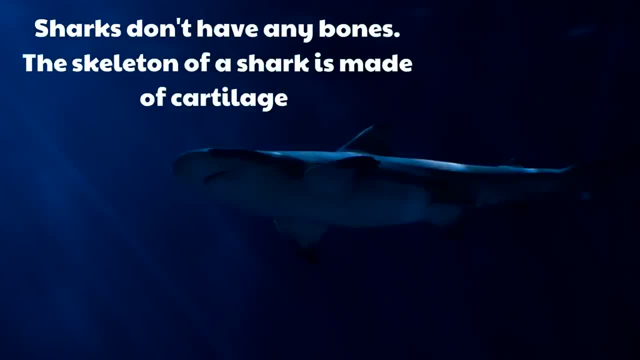 common, For example, sharks don't have common, For example, sharks don't have any bones. The skeleton of a shark is any bones. The skeleton of a shark is any bones. The skeleton of a shark is made of cartilage. That goes for all. 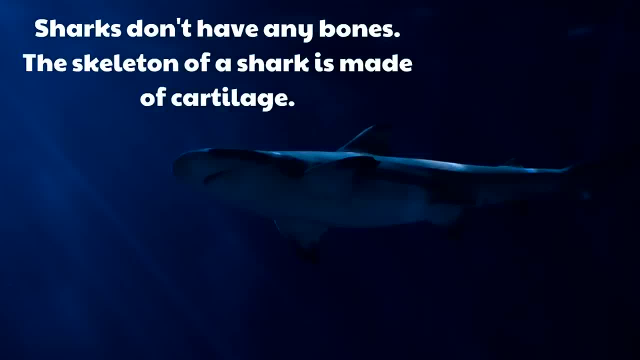 made of cartilage. That goes for all. made of cartilage. That goes for all. sharks. Sharks don't have bones and it's sharks. Sharks don't have bones and it's sharks. Sharks don't have bones, and it's interesting because most other fish do. 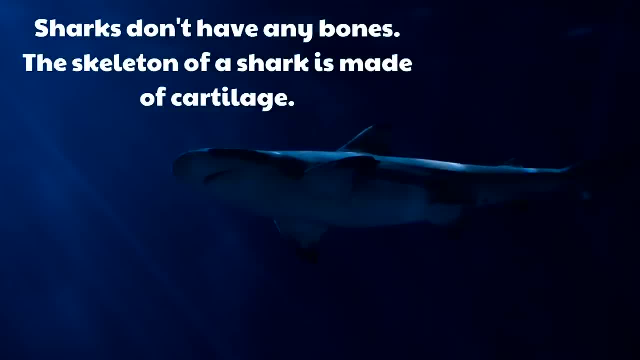 interesting because most other fish do. interesting because most other fish do have bones, but sharks don't Okay. so the have bones, but sharks don't Okay. so the have bones, but sharks don't Okay. so the skeleton of a shark is made of. 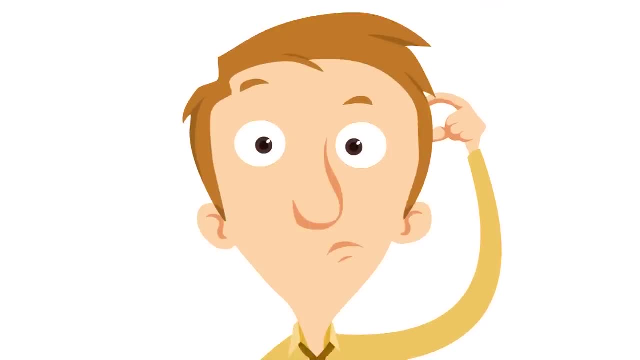 skeleton of a shark is made of. skeleton of a shark is made of cartilage. but what is cartilage? What cartilage, but what is cartilage. What cartilage, but what is cartilage. What does that mean? What is cartilage? Okay, 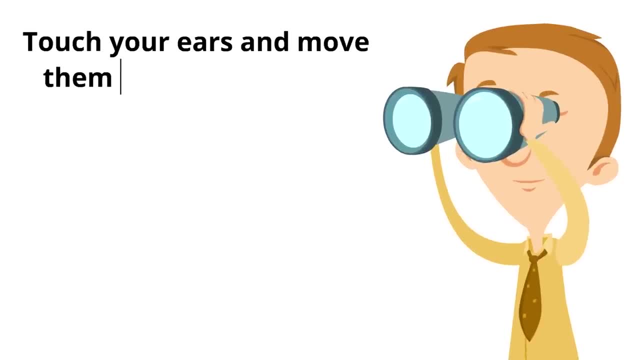 does that mean What is cartilage? Okay, does that mean What is cartilage? Okay, this is gonna sound weird. but touch this is gonna sound weird. but touch this is gonna sound weird. but touch your ears and move them around with your. 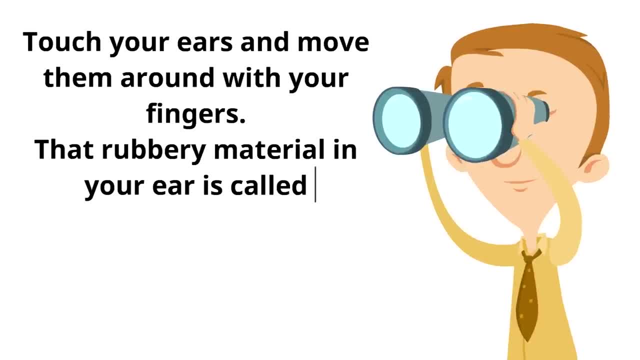 your ears and move them around with your, your ears and move them around with your fingers. That rubbery material in your fingers, That rubbery material in your fingers, That rubbery material in your ear is called cartilage. Isn't that ear is called cartilage, Isn't that? 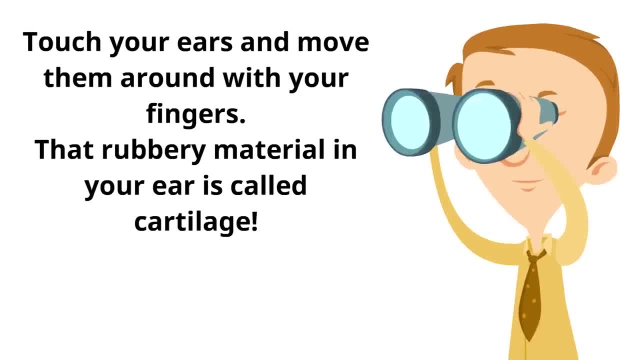 ear is called cartilage. Isn't that amazing. There's some cartilage in your amazing. There's some cartilage in your amazing. There's some cartilage in your body, just like there's cartilage in the body, just like there's cartilage in the. 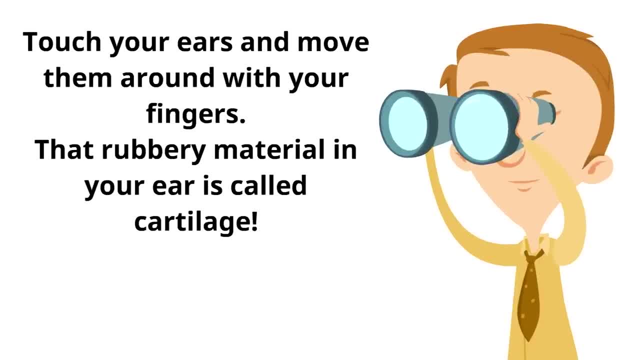 body, just like there's cartilage in the body of a shark. The skeleton of a shark body. just like there's cartilage in the body of a shark. The skeleton of a shark body. just like there's cartilage in the body of a shark. The skeleton of a shark is made of cartilage, which makes a shark very 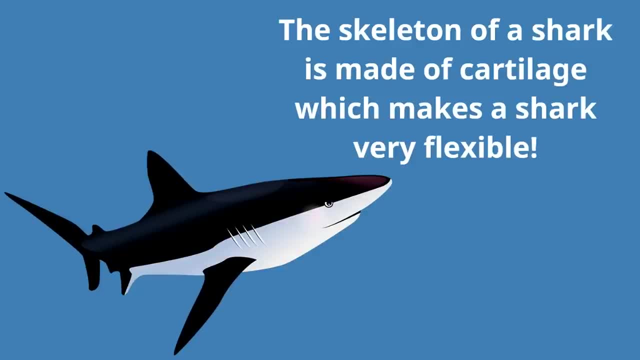 is made of cartilage which makes a shark very, is made of cartilage which makes a shark very flexible, kind of like your ears right flexible. kind of like your ears right flexible, kind of like your ears right. Your ears were kind of rubbery and 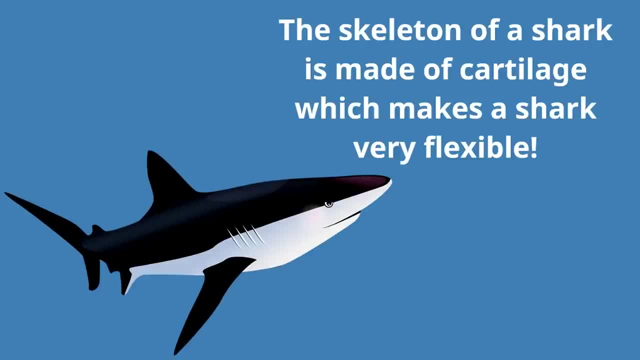 Your ears were kind of rubbery. and Your ears were kind of rubbery and flexible when you touched them. That's flexible when you touched them. That's flexible when you touched them. That's the way the skeleton of a shark is. the way the skeleton of a shark is. 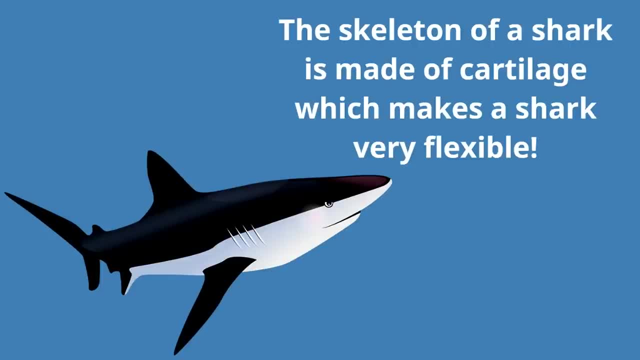 the way the skeleton of a shark is, which helps a shark move around. in which helps a shark move around. in which helps a shark move around in special ways. It makes a shark very special ways. It makes a shark very special ways. It makes a shark very flexible. 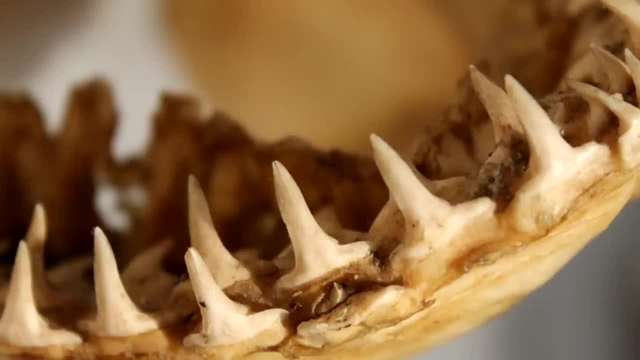 flexible, flexible. Hey, you want to know what's not. Hey, you want to know what's not. Hey, you want to know what's not. flexible Shark's teeth. Aha, flexible Shark's teeth. Aha, flexible Shark's teeth, Aha, Shark's teeth. 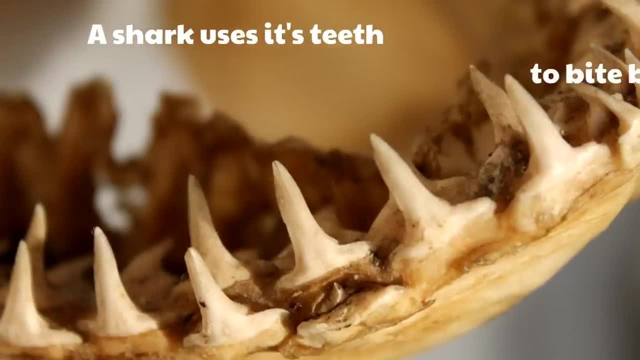 Shark's teeth, Aha, Shark's teeth, Shark's teeth, Aha, Shark's teeth. This is interesting. A shark uses its. This is interesting. A shark uses its. This is interesting. A shark uses its teeth to bite, but not to chew. 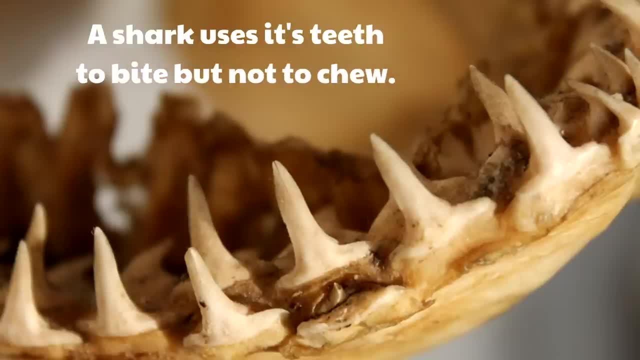 teeth to bite, but not to chew. teeth to bite, but not to chew. Whatever they bite that goes into their, Whatever they bite that goes into their, Whatever they bite that goes into their mouths. sharks swallow whole, We use mouths. sharks swallow whole, We use. 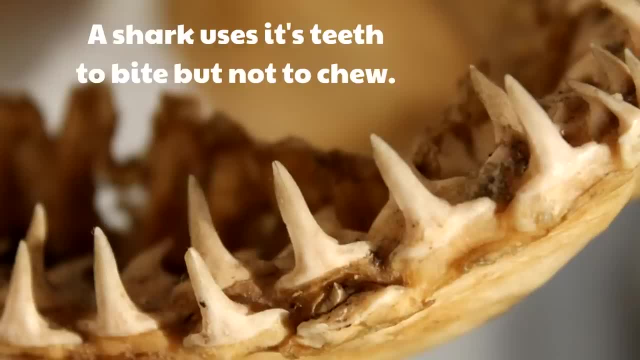 mouths sharks swallow whole. We use our teeth not just to bite, but to our teeth. not just to bite, but to our teeth. not just to bite, but to chew. But a shark only uses its teeth chew, But a shark only uses its teeth. 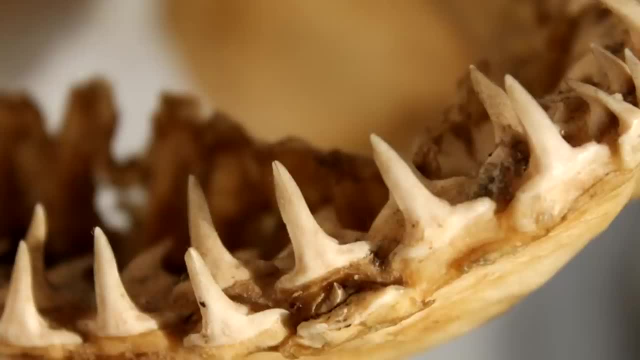 chew, But a shark only uses its teeth to bite, to bite, to bite, And a shark can have a lot of teeth in. And a shark can have a lot of teeth in. And a shark can have a lot of teeth in its lifetime. 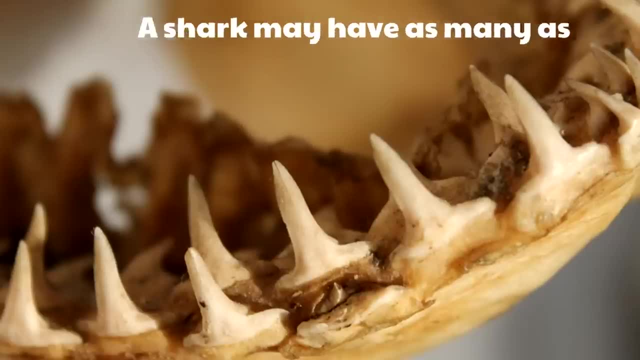 its lifetime. its lifetime. Now here's the crazy part: A shark may. Now here's the crazy part: A shark may. Now here's the crazy part: A shark may have as many as 20,000 teeth during. have as many as 20,000 teeth during. 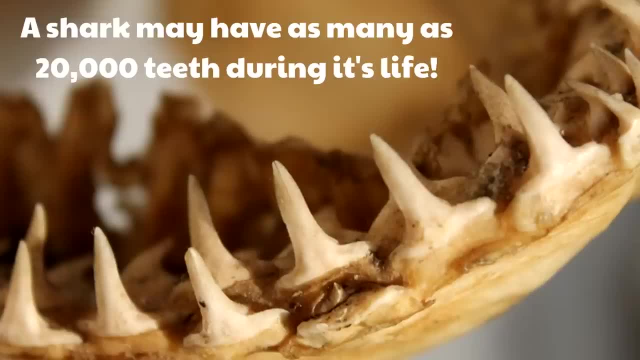 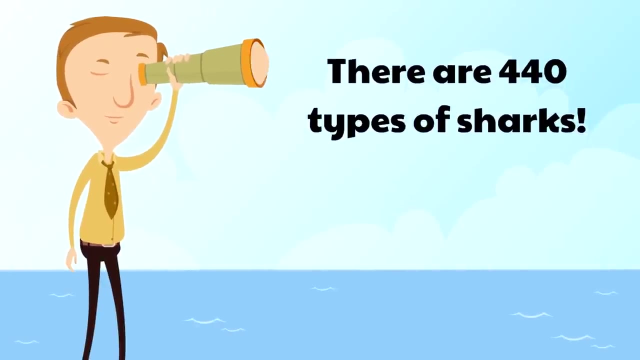 life. there are rows of replacement teeth that, in case a tooth gets broken or falls off and gets lost, a new tooth emerges. now we've already mentioned there are 440 types of sharks. in fact, you're probably sick of hearing the fact that there are 440 types of sharks. how many types of sharks are there? how many? 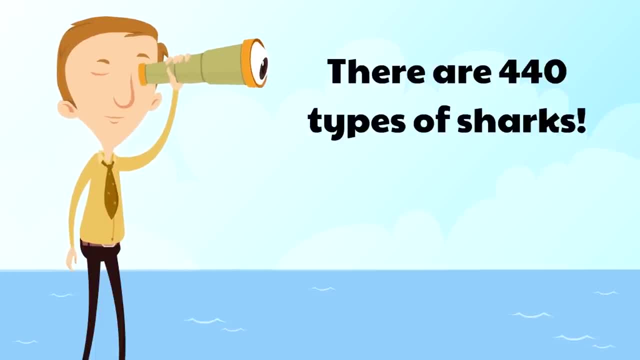 four, okay, 440. all right, we're gonna just show you four of our favorites. there are a lot of other cool sharks. we're missing a lot of them. we're gonna show you four sharks right now so that if you see these sharks in the future, you'll be like: I know what type of shark that is. the first shark is the whale. 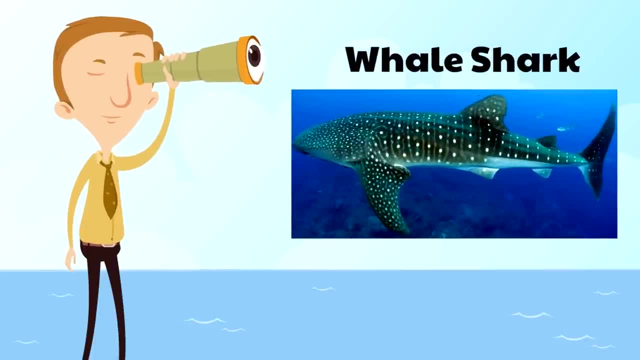 shark, and we've already talked about how the whale shark is the largest shark in the world. yeah, but what's cool about whale shark sharks? they have these white spots and they're very gentle. so even though they're huge, they're very gentle. in fact, some whale sharks have even let divers 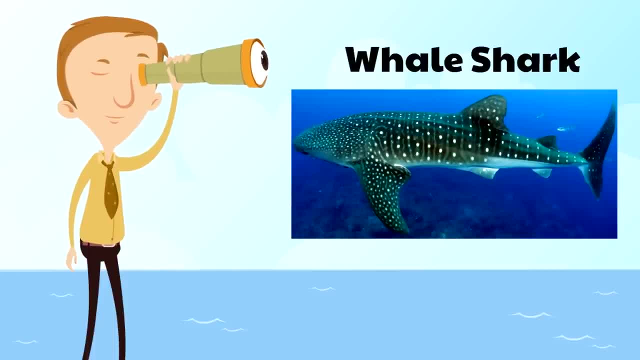 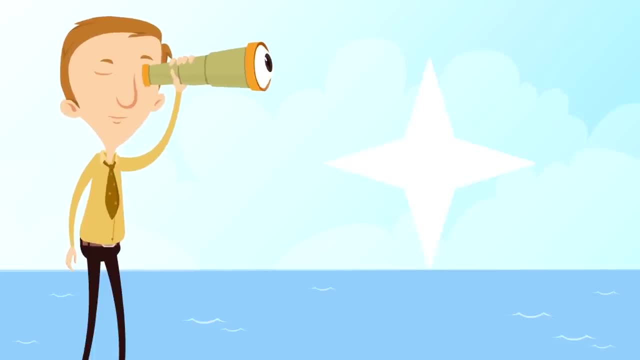 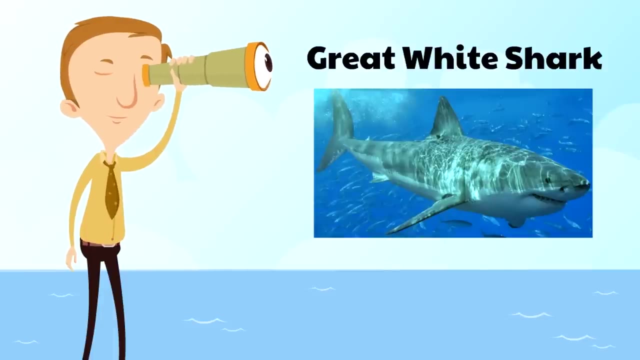 sit on top of them. how would you like to ride a whale shark? what next? we're gonna show you the great white shark, perhaps the most famous shark of them all. this is the shark that most people think of when they think of the great white shark. the shark that most people think of when they think of 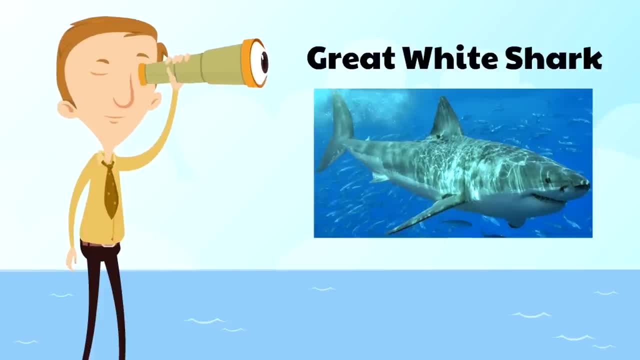 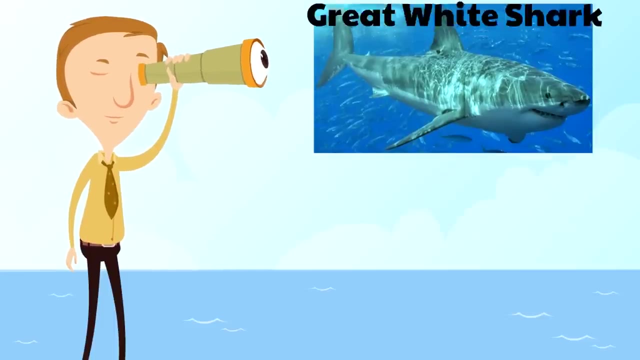 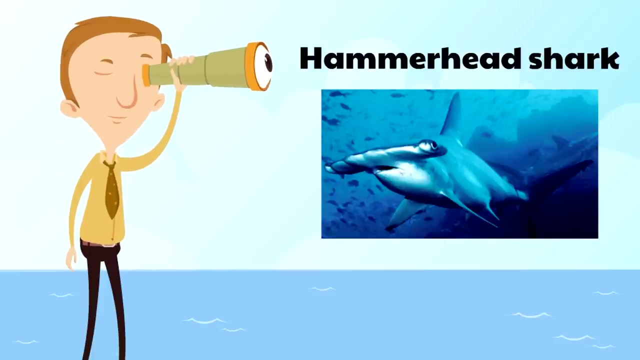 sharks, and the great white shark is really intense, 23 feet long, and they eat all kinds of things: dolphins, sea lions, whales, seals and even other sharks. next is the hammerhead shark, which gets its name because its head looks like a hammer, which it kind of sounds like a mean name. like you know, some of the 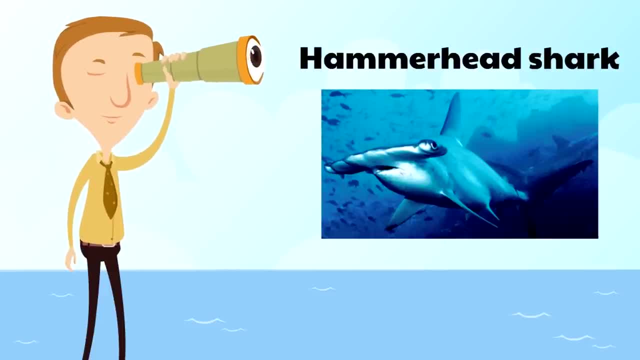 other sharks were like: hey, hammerhead. he was like: hey, you know, don't call me that, but you know the name kind of stuck the hammerhead shark. it's interesting. that's actually an advantage for the hammerhead shark. it helps with the swimming and also helps with the eyesight- the eyesight of the hammerhead. 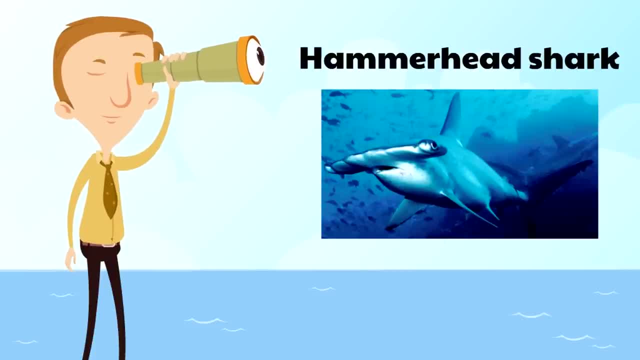 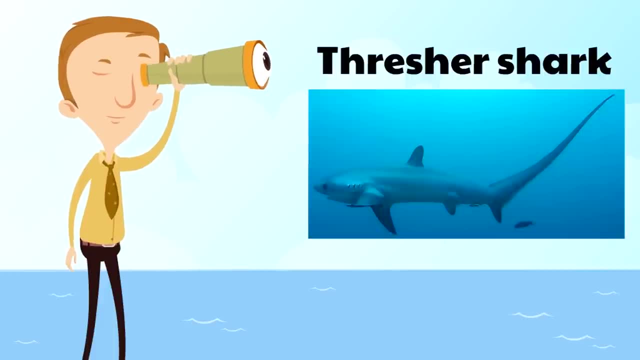 shark is much better, especially at gauging distance, than other sharks. finally, there's the thresher shark. the thresher shark is a very strong shark, known for its very, very long tail, and that tail can be huge. in fact, the tail of a thresher shark can weigh as many as 300 pounds or more. Wow, the 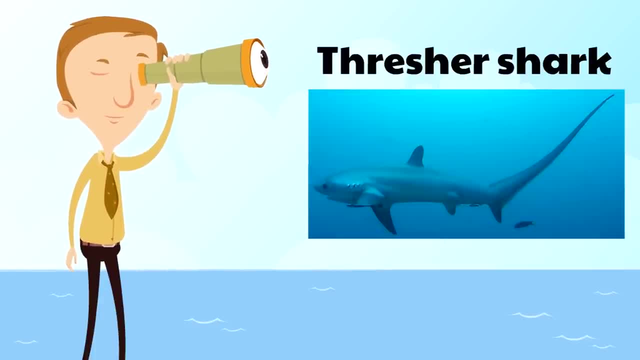 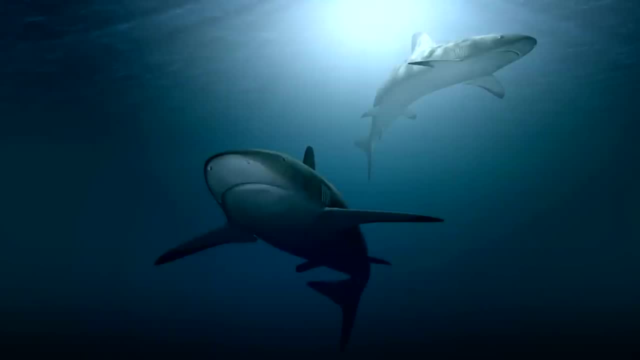 thresher shark. those are just four amazing types of sharks. we left out so many, but just understand, sharks are incredible creatures and, as humans, we need to be strong sharks. we need to be strong sharks. we need to be strong sharks. many people don't realize how much we need sharks. a lot of people don't realize. 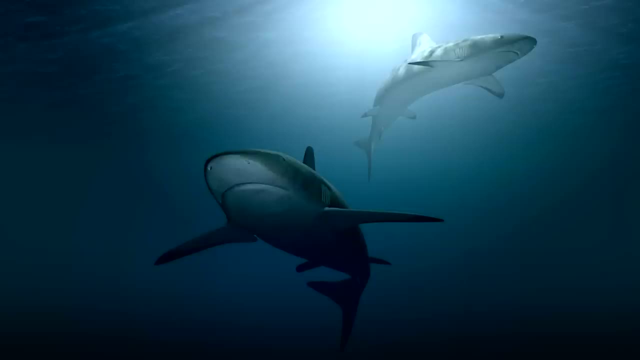 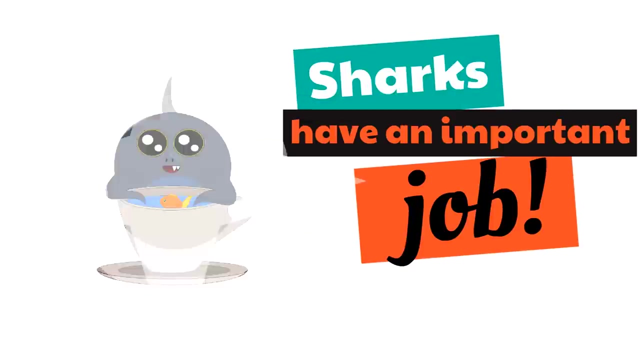 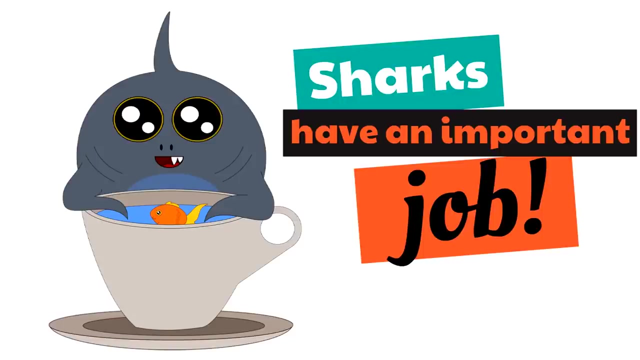 how much we need sharks. you see, sharks have an important job, a very important job, and it's not babysitting fish. because, Fred, I don't trust you with Henry. I really don't. I really don't think that you can be trusted with Henry, because I think what we're looking at here is a snack time, alright, and you're 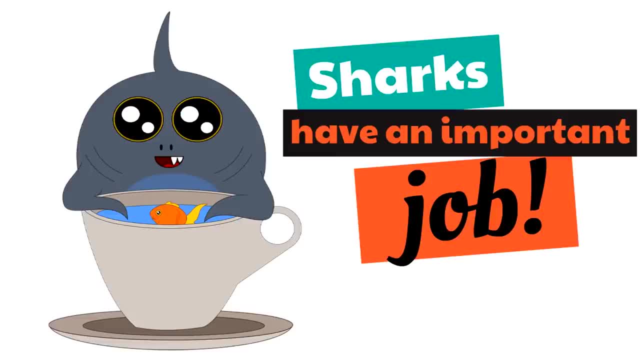 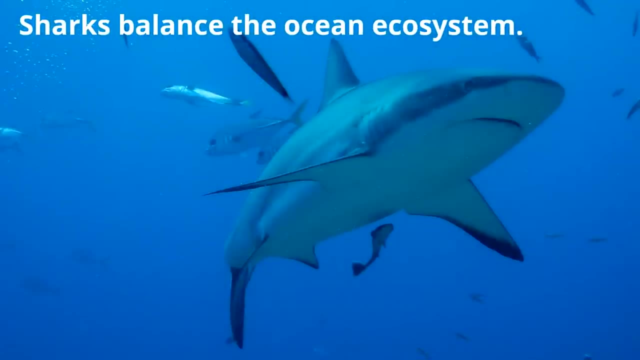 just not the best babysitter, okay, I don't really trust that. Henry is a snake. he's gonna make it throw, okay? so what is a shark's important job? what do sharks do? here's their job. sharks balance the ocean ecosystem. the ocean just wouldn't run as well without sharks, and there are a lot of ways that sharks balance the 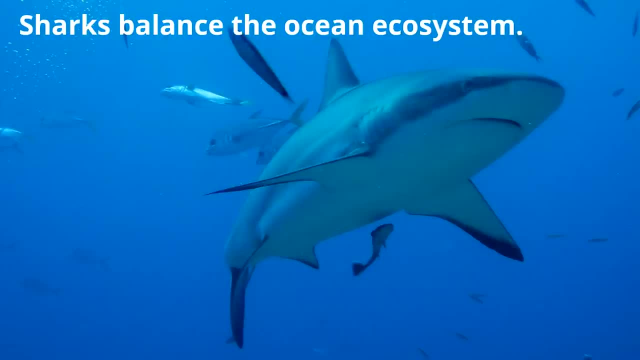 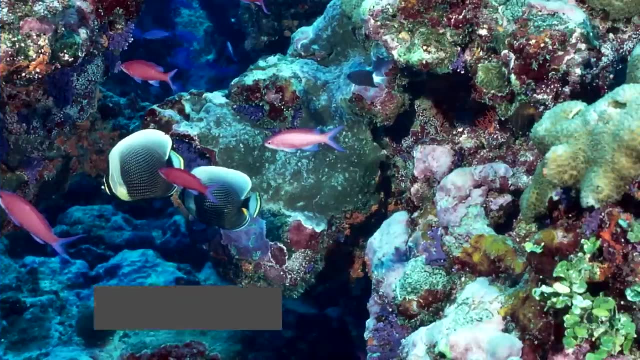 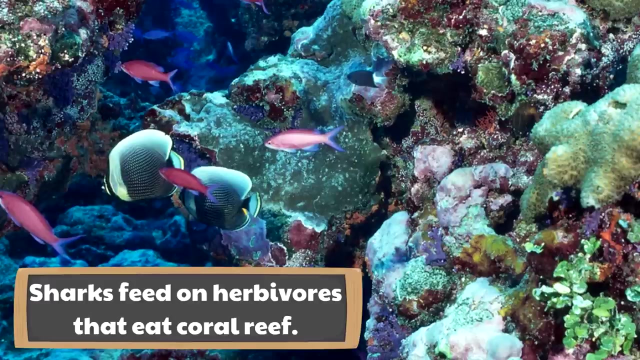 ocean ecosystem, but we're gonna give you one specific way, just so you can see how important sharks are. so here is our example. sharks feed on herbivores that eat coral reef, and you might say, well, how is that important? well, in places where there aren't enough sharks, coral reef has been wiped out and it's. 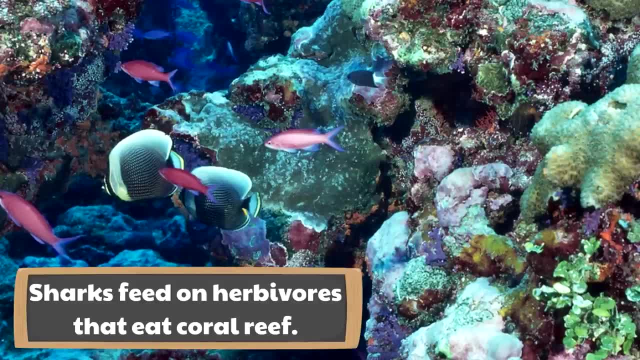 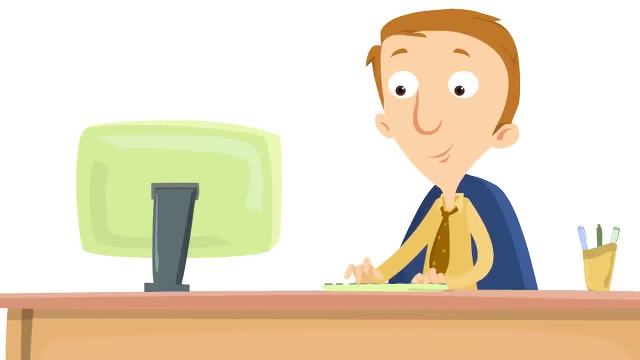 replaced with this gross, nasty algae. it's not just coral reef that gets affected. all different types of of creatures in the ocean would be affected by that. the balance is held together by these amazing fish called sharks, with the skeleton made of cartilage, that work hard to balance the ocean, even though they don't realize.